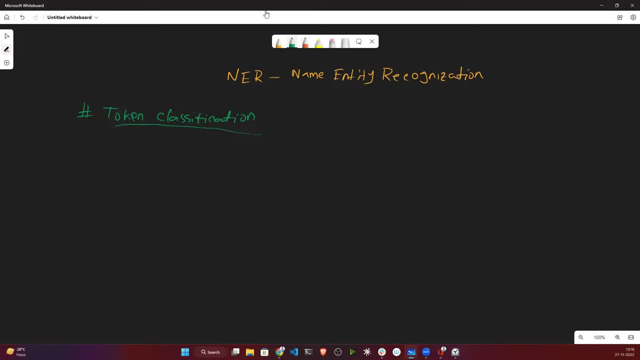 is in-ear. first of all, you need to understand what is in-ear. So if I tell about what is in-ear, so find entities, okay, Such a person, then you can talk about location or organization, okay, And so on. Okay, Now, how it can be token. 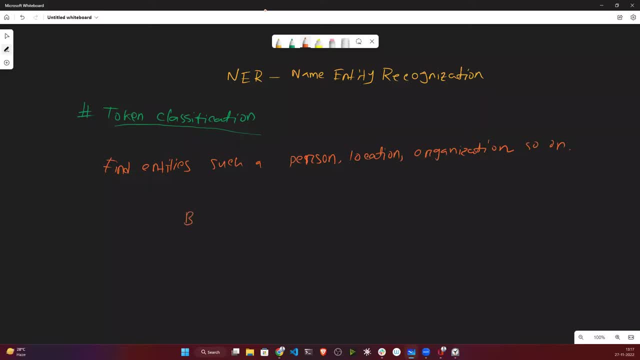 classification. Suppose here, if I write something, Bill Gates is a founder of Microsoft. Okay, Now here, using in-ear, what you are doing? actually you are doing token classification okay, Suppose I think you are already familiar with, like what is token okay In NLP. So 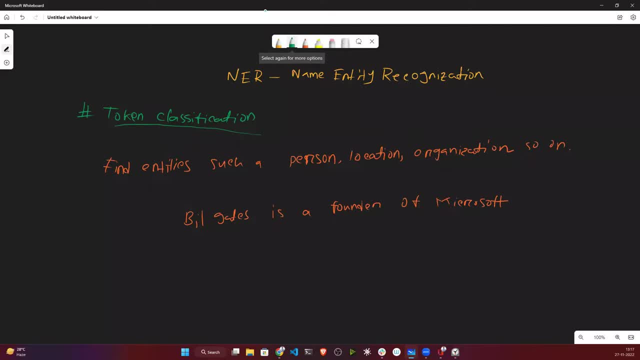 first of all, whenever you are getting the data, you need to convert it to token. okay, You need to apply the tokenizer. So, whenever you will be applying the tokenizer, so what it will give you, It will give you like separate, separate word, okay. 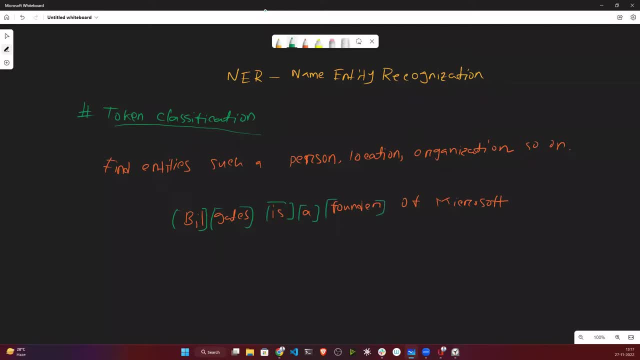 Like that. Okay, So now in-ear will be classifying each of the tokens, okay, In an entity Like how, Suppose, what is Bill here? Can anybody tell me Bill is a person, Okay. What is Gates here? It is also a person, Okay. Is you can define as: 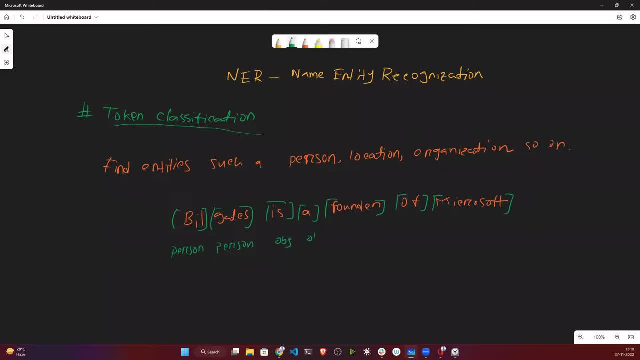 like objects. A you can define as objects, Founder you can define as designation- Okay, Designation Of you can define as objects, And Microsoft you can define as organization- Okay. So basically here what you are doing, you are classifying, 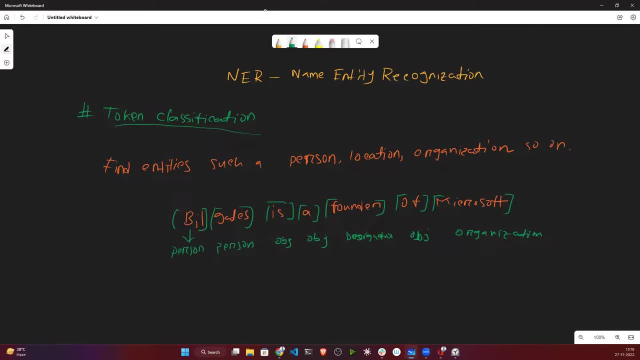 token-wise. Yes, yes, I will share no issue. Okay, No issue. See here what you are doing: you are classifying token-wise, Each and every, every token. see, you are trying to classify. So that means you are doing something called token classification. okay, So that's why. 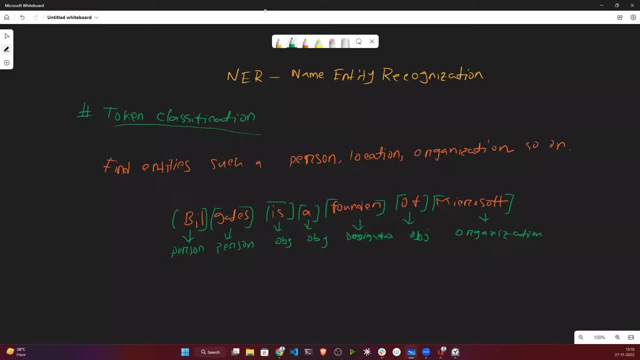 we call it token classification. Whenever we are doing N-ear, we call it token classification. So if you go to HuggingFace, so there you won't be getting any N-ear, okay, N-ear you can say like sector. So if you want to do, if you want to perform N-ear, so there. 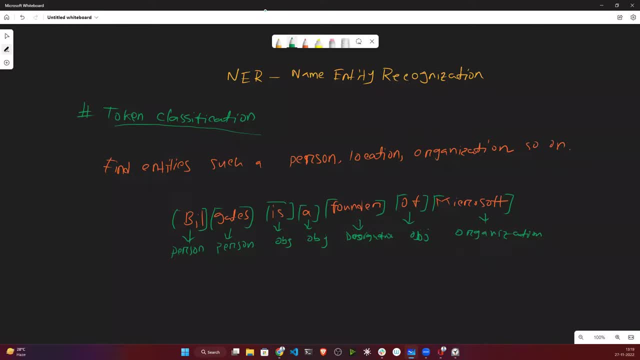 actually you need to select something called token classification Inside that you will be getting all the algorithm. Okay, So today I will show you one example. So I will be using BART. Okay, BART Anki's model, So it is one of the transformer-based architecture. Okay, I think? 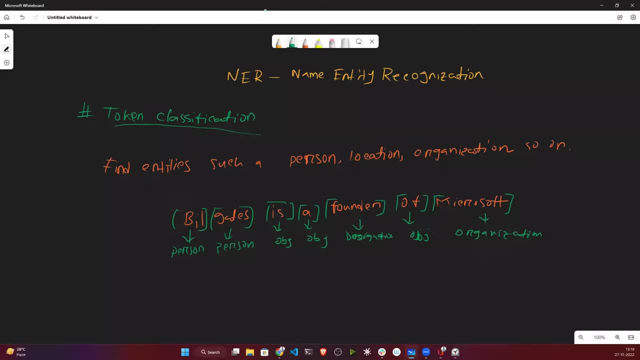 you have heard of BART, Okay, So I will show you, like, how to fine-tune BART, Okay, And how to train your own custom data. Okay, For this N-ear. So now I think you got it. like what is N-ear? 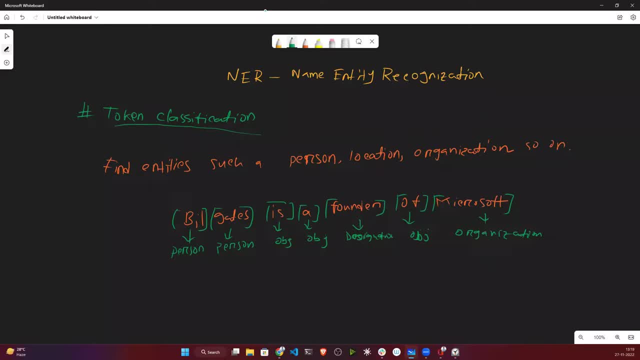 all about Now, if I talk about the application of N-ear. suppose you have bank checks or if you have like resume, So suppose you want to get information of the resume or get the information of the checks. Okay, So you can perform N-ear. So what it will return? It will return the name. 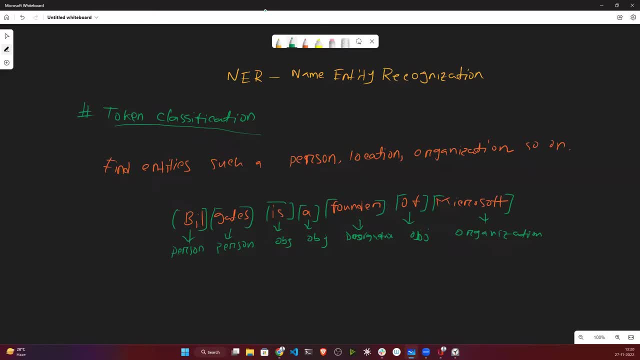 of the person. It will return like the experience of the person, Okay, The skills of the person. Then, where did he study? Where did he live? Actually, what is the email address? So these kinds of actually like required information you can. 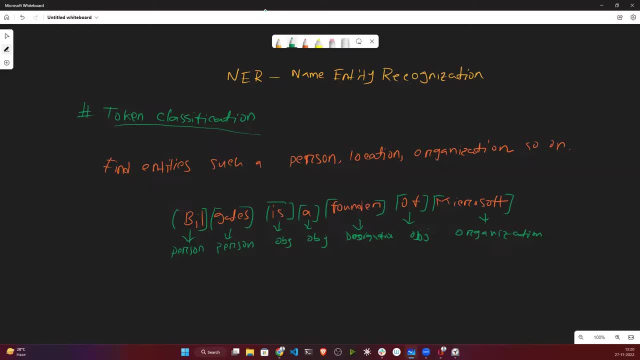 like collect: Okay, By using N-ear. Okay, So N-ear. most of the time you will be using resume parser, Then information extraction: Okay, So these are the actually application you will be. 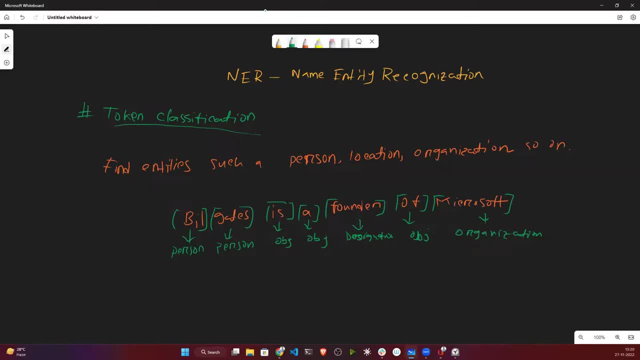 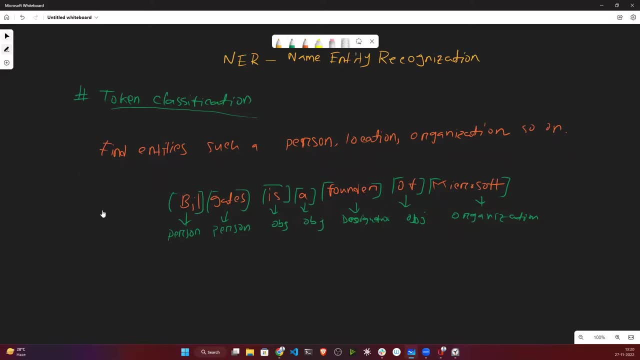 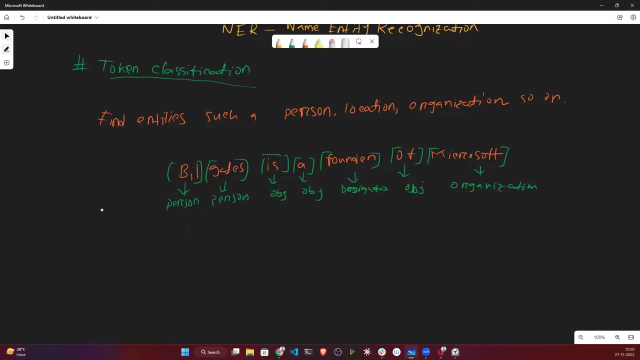 using a lot. Okay, So not only N-ear is present inside token classification, there is other two application is also there, or two tasks you can talk about Like. another is POS. That means parts of speech tagging. Okay, Now, what is the difference between parts of speech tagging? So here. 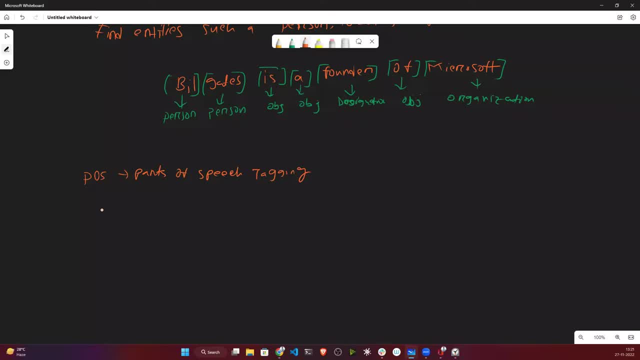 what you do basically here. you try to mark each word Okay In a sentence, Mark each one in a sentence as corresponding to a particular parts of speech, Okay. So I think you are familiar with parts of speech. So, such as: 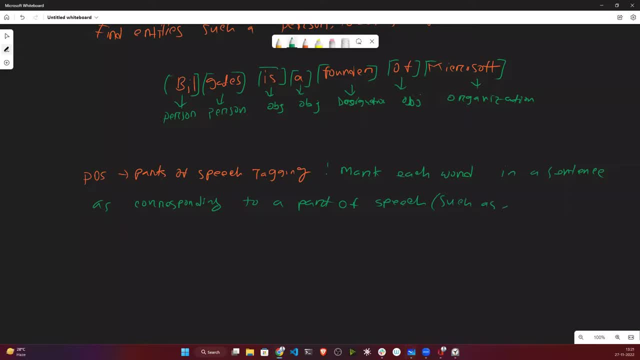 okay If I give you the example. so what would be the example? So you can write noun, Then verb, Okay, Then adjective, Yeah, So, yeah, How many like parts of speech you can think you can like do it Okay. So this is one of the like tasks parts. 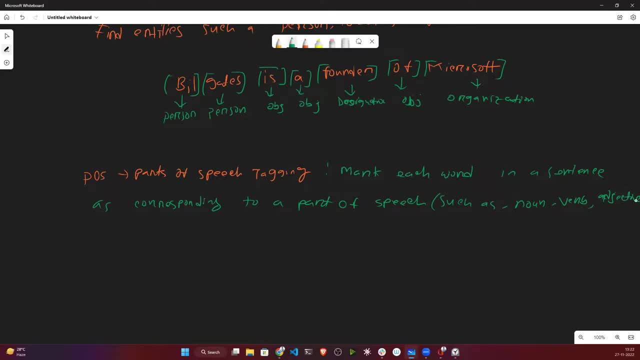 of speech, tagging And why this parts of speech is important, Because I already told you here creating any conversational agents or you can talk about like summarization, So at that time actually you need to understand the parts of speech, Okay. 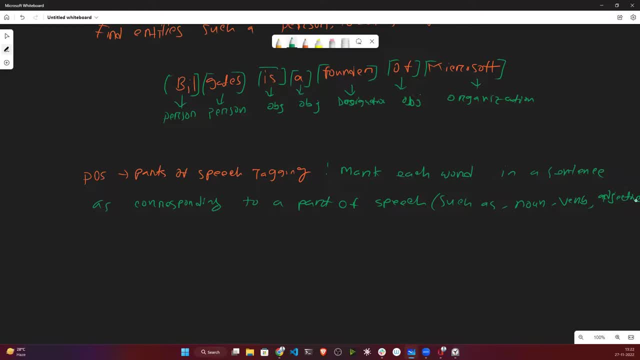 The sentence you are writing Right To get the better context is all about Right, So that is why this is important. So everywhere, whenever you are creating any kinds of advanced NLP application, at that time this POS tagging is like very important. Okay, After processing your 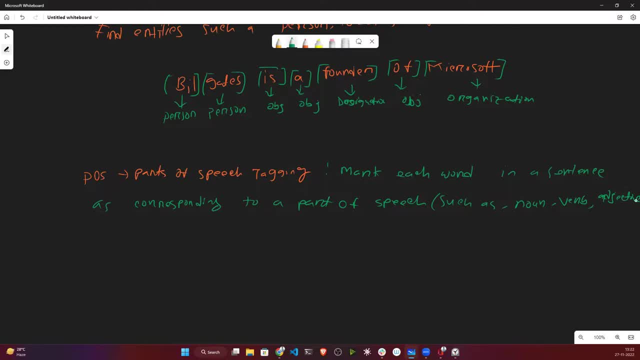 data you will be applying POS tagging. Then that POS tagging actually you will be passing to create your conversational agents and all So whenever you are passing any sentence- suppose I am passing Bill Gates- You are the founder of Microsoft. So actually, what is subject, What is verb? Okay, What is? 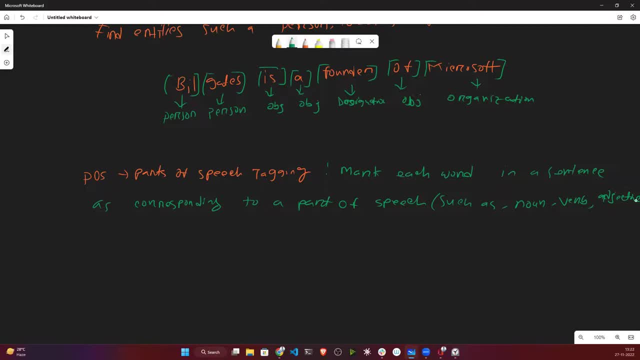 noun here. What is object here? Okay. What is adjective here? If you say everything, actually you need to like tags, Otherwise you don't be able to understand in a correct way. Okay, So now another task is there. You can perform inside token classification. 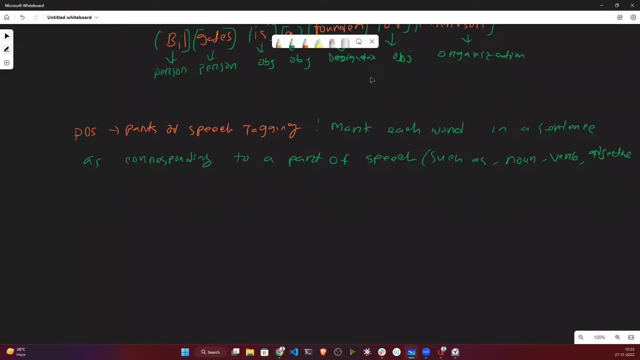 which is nothing but Jenkins. Okay, So let me write, Just give me a moment. Yeah, Which is nothing but Jenkins, chunking, okay. so what is chunking actually? suppose, uh, it is your n? er only, like name, entity only. but what you do here, you just try to collect the same entity, suppose? uh? 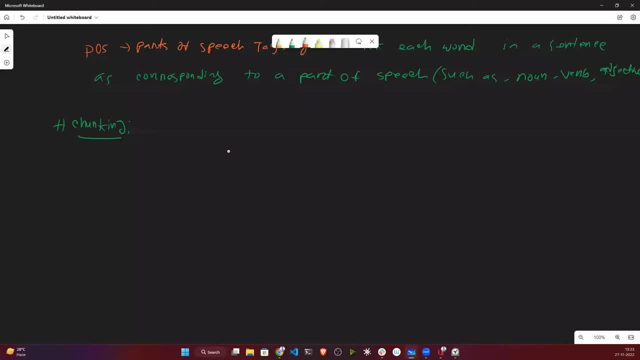 if i write the uh, the same example again. like bill gates is the founder of microsoft. okay, so here, what is bill? bill is a person per again gets. is a person per is objects. objects you can designation, you can talk about. okay, then off again, objects and microsoft. 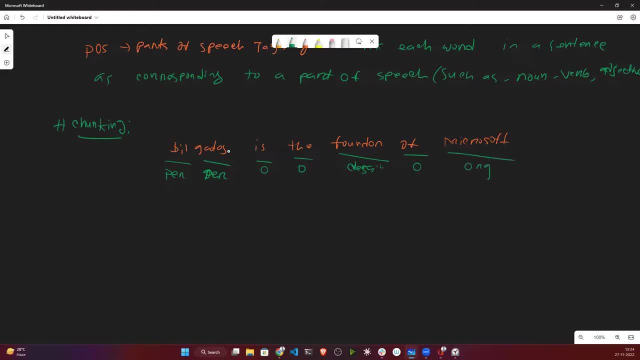 is organization. so here, basically what you are doing. so just tell me, here you can see similar kinds of entity or not. like if i talk about bill and gates, these two are person. actually it is mentioning, so i can talk about. these two entities are similar. so what chunkings? 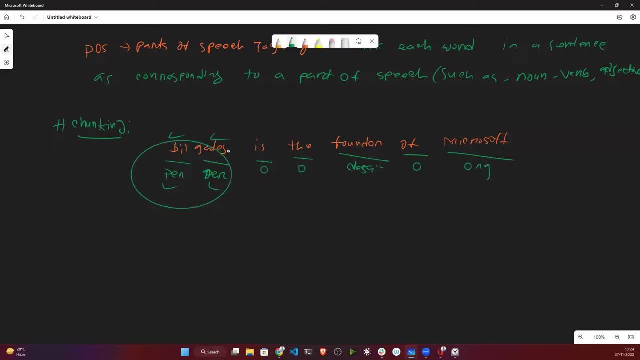 will apply. chunkings will just like combine them together. suppose bill gets, okay, it will combine as a person got it. what is chunkings? it will basically try to identify like what is the similar entity? okay, where it will see the similar entity, it will just combine because i, i i am not supposed to write bill- and gets separate, separate person because bill gets. 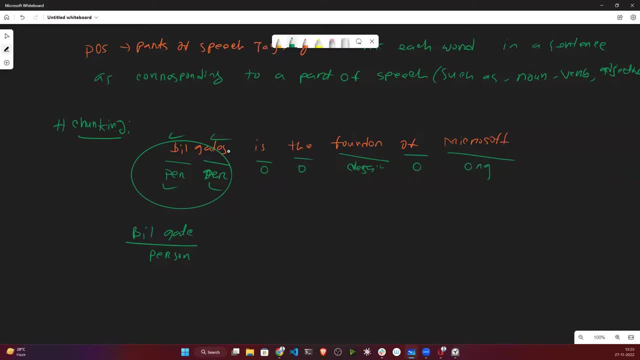 is like just one person, not two person, right? so chunkings will help you to combine them. is it clear guys? yes or no? okay, so, yeah, so this is all about your token classification task. so here, basically, this two is not required. uh, because, because parts of speech tagging, it's like a like advanced. 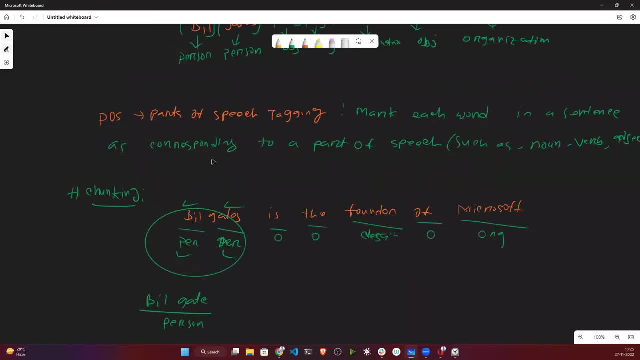 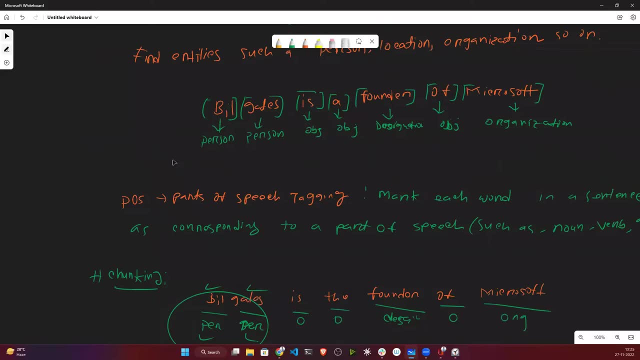 concept. so for that you need, like, language understanding, okay. so, uh, we don't need this one because i will be using transformer and like all the things that we are going to use. okay, so it is already known, these are the parts of speech and all, but this is like very much. 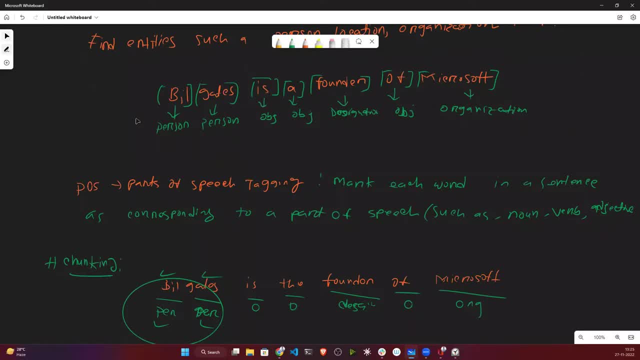 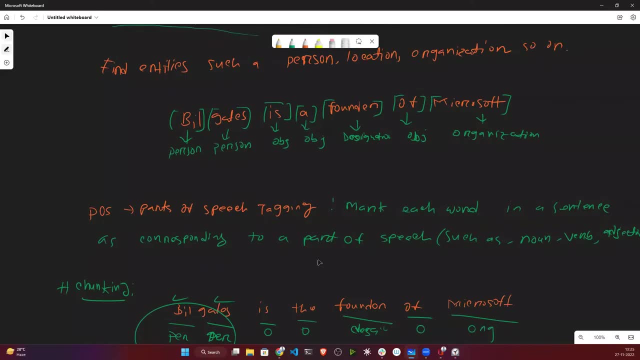 important inside token classification, which is nothing but ner. okay, name entity recognition. so now let's like see that any year. okay, any example. so the data will be working. first of all, let me show you the data. so this is the data guys. okay, i'll be using. so this data actually. 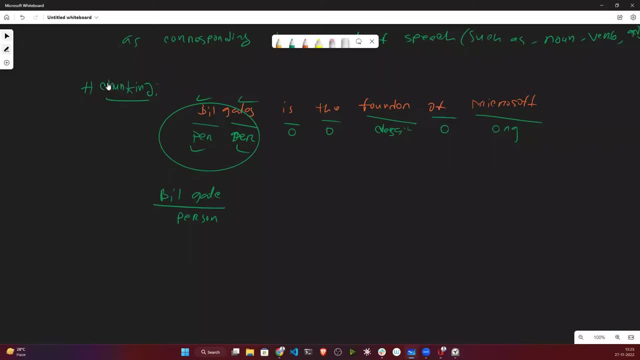 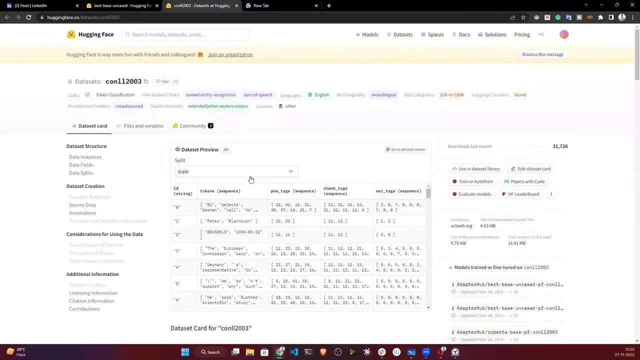 is available inside hugging phase. okay, so that data name is con. uh, ll 2003. okay, so this is the data. it's like a csv data you can talk about. so here, actually, what you have. you have id, unique id, then you have tokens. okay then with respect to that. uh, yeah, with respect to that. 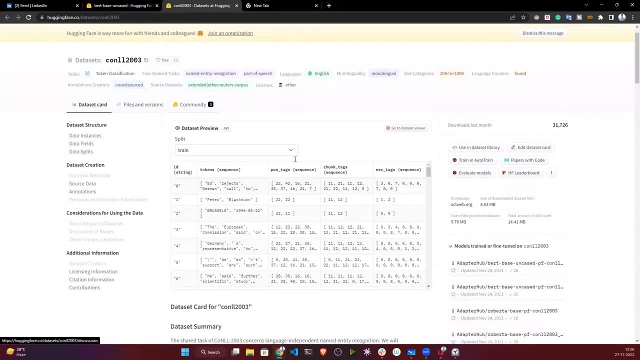 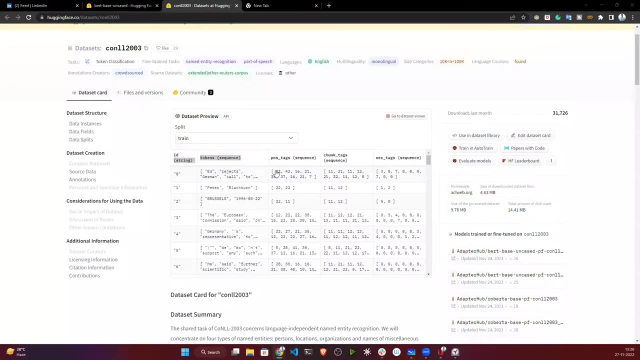 you have your pos tags okay. so see, it is already like label data. okay, they have already annotated this data and make the label okay. so pos tags is also available. but for our case i won't be using this column pos tag. it is not required because i am not doing the pos tags here. 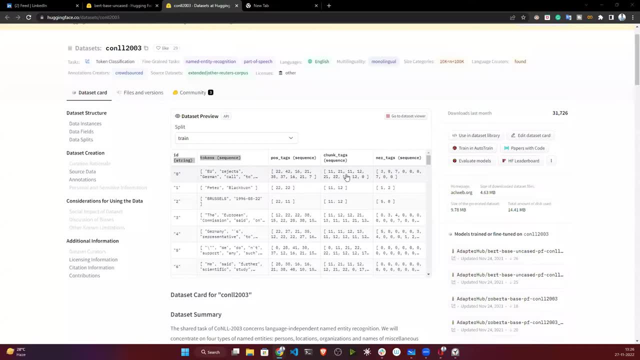 chance tag is also there. okay, i won't be using chance tag because here i'm not performing, so what i will be using? i will be using something called any other tags. okay, this one. now let's discuss, like, how they have created this data. let me copy one example from here. 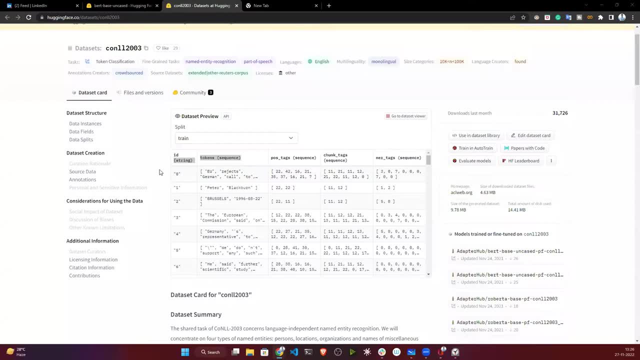 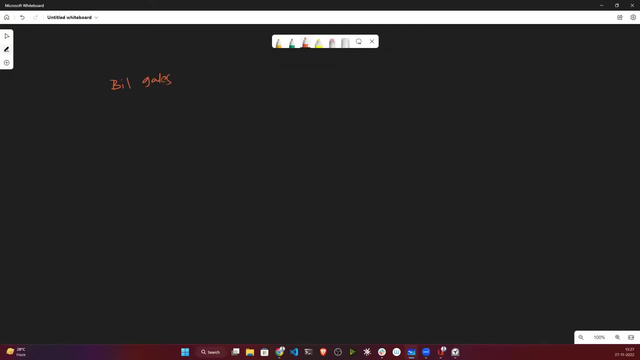 okay, let me write down like: first of all, let me show you like: uh, how you can annotate your data. suppose you have something here. let me take the same example. like bill gates is the founder of microsoft. okay, suppose this is your raw data. okay, this is one string. so, first of all, first step, what you 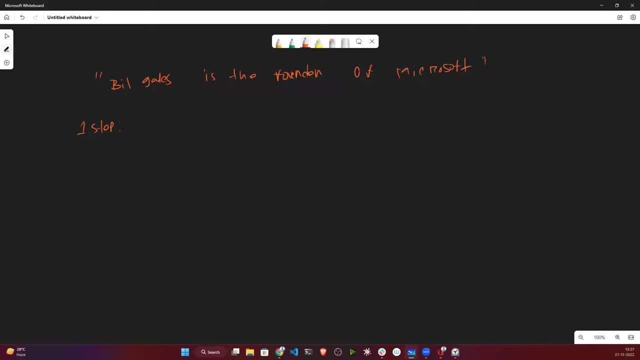 will do. can anybody tell me, first step, what you will do? okay, suppose this is your raw data token, right, so let's make it as token. so here you will. this is your list. inside list: you have bill, comma gets, comma is. then you have the okay founder of then Microsoft. okay, so now you have tokenized the data. okay, so now second: 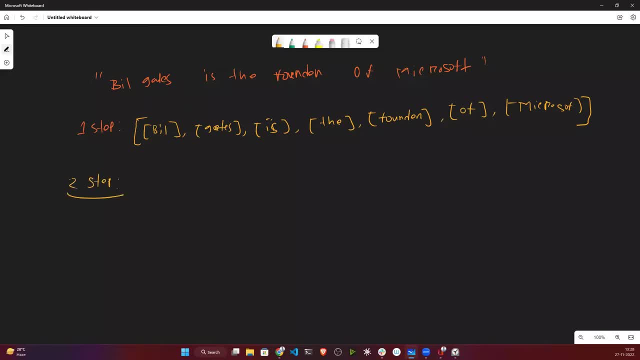 step, twin step. can anybody tell me what I need to do? no, actually stop words like it's not required here. okay, remove stop words not required because, see here, your task is to identify the relevant information you want. okay, so you can ignore the stop words as objects. 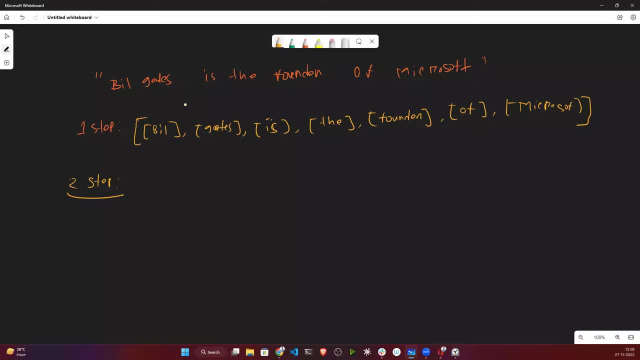 okay, because objects you won't be like taking only, you will be taking the name organization. okay, designation, these are the thing, okay, so removing strong words, not like required here. okay, yeah, someone tell like embedding: okay, he's correct, because now, see, this is my. okay, he's correct, because now, see, this is my. 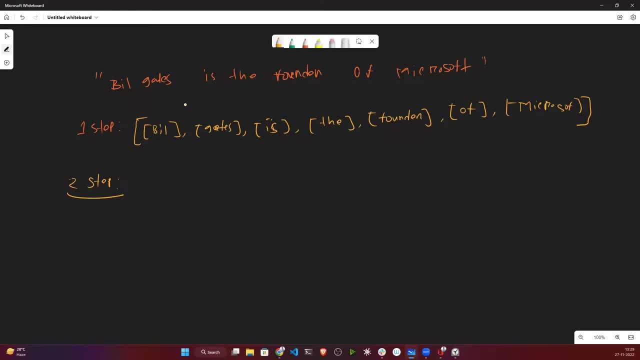 text data. okay, I can't give this text data to my model, so what I need to do, I need to generate some unique ID. got it? so let's let's generate. you can do one not encoding or any encoding like integer encoding. you can do so if you do include integer encoding. so suppose, 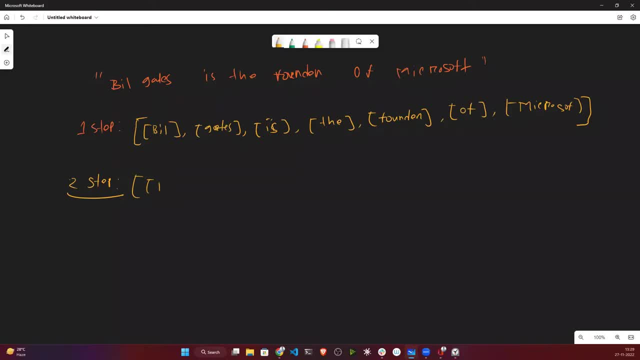 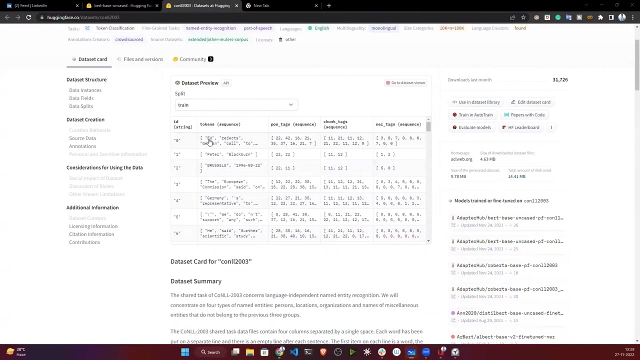 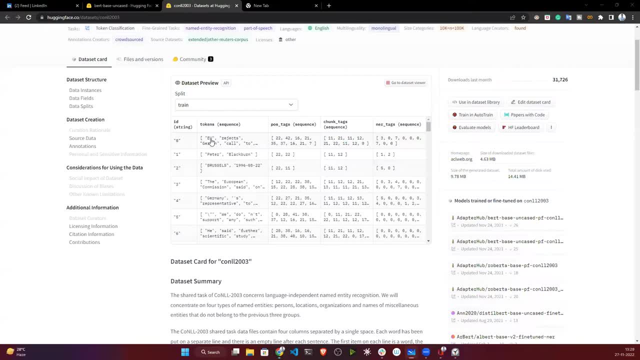 any attacks. now see each and every tokens. they are defined with some id, unique id: see 307. just count here: 1, 2, 3, 4, 5, 6, i think, 9, 9, 9. 1, 2, 3, 4, 5, 6, 7, 8, 9, 9 words is there. so 9 words has been, uh like. 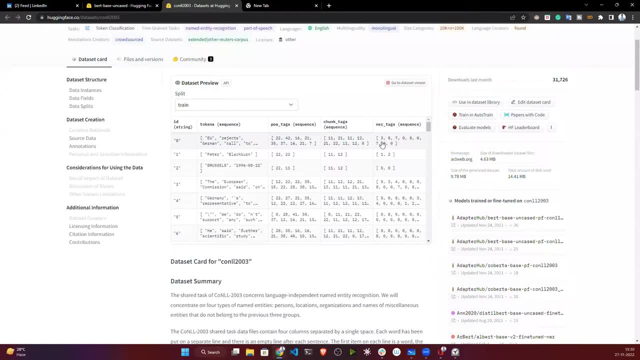 you can say it has been encoded here. okay, with a unique, unique number. is it clear, guys, how they did the annotation, how they came up with this number? okay, now you can ask me, like i can't see any, like what, what is three means? okay, three means person or organization or objects, okay. so if you 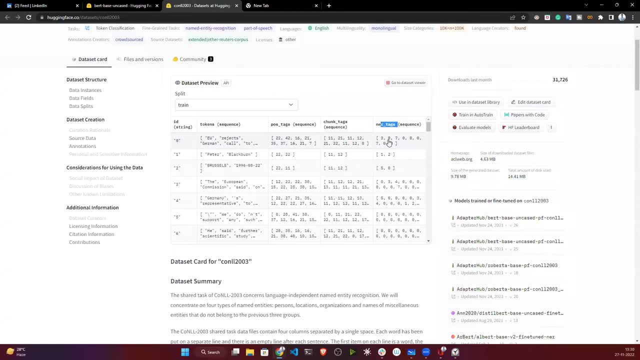 want to see. so if you just go below. so they have mentioned about that data. so see, this is one dictionary. they have created zero representing objects, then b person, it is representing one. i person, it is representing two. b organization it is representing three and four means you are defining i organization. i will tell you what is b organization and what is i. 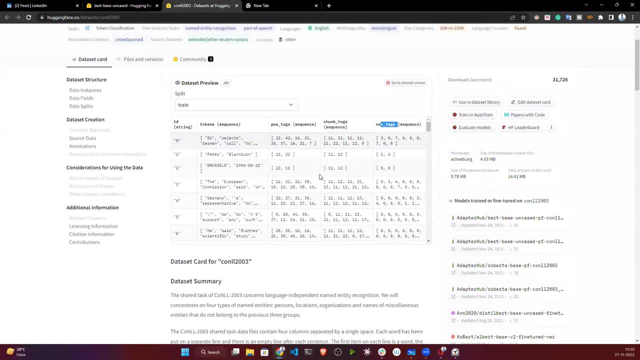 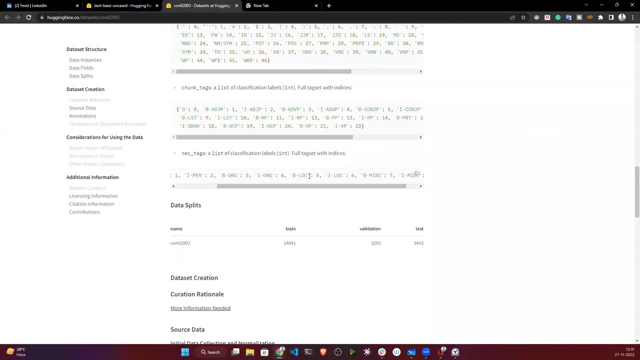 organization. okay, try to understand. like how they have encoded. okay, they have created one dictionary and they are representing each and every tax with some unique id. is it clear or not? guys, just tell me, i will tell you what is i means, what is b means? is it clear? 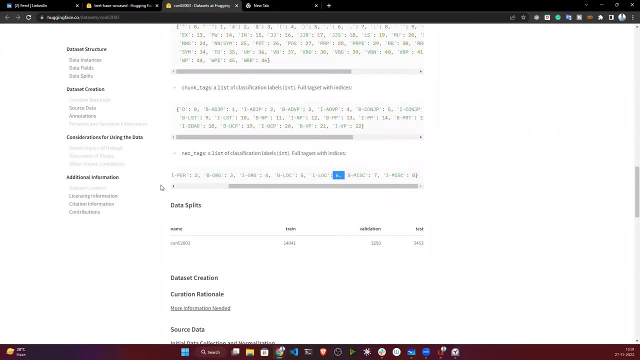 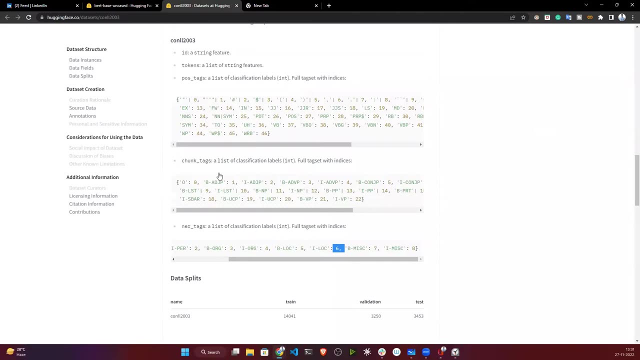 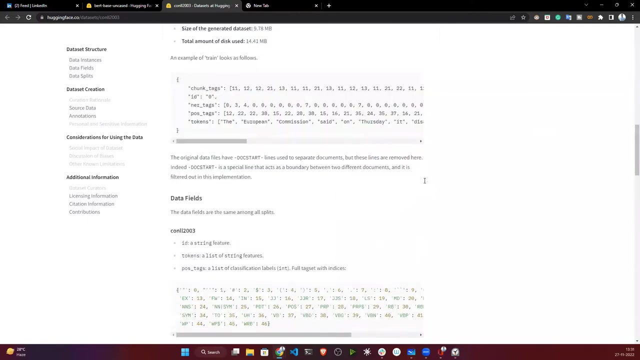 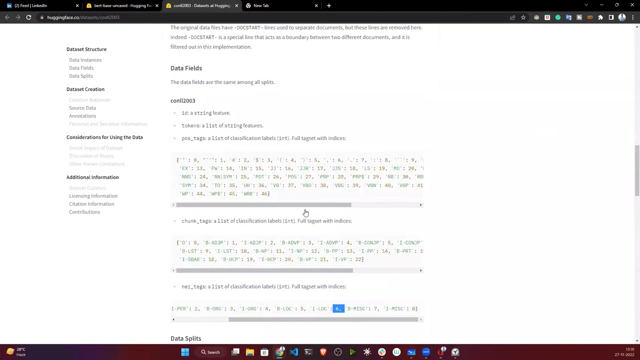 now, if i, if i show you this one, if i tell you what is three means what he will tell. just go here, see three. three means like i, organization, okay. so you can see xeerman, uh, zero one, two, three, okay, first one, you, you, okay, you is organization. 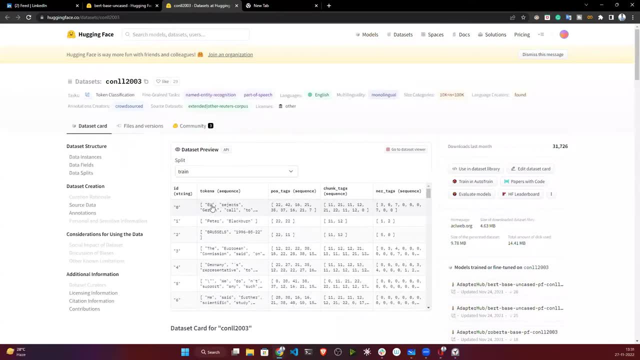 got it because if you read the, i will tell you whenever i will import the data to my notebook. at that time it will be very visible. okay, you reject sherman call. so you eat what. you read the sentence, you will see it's organization. okay, now let's talk about like. 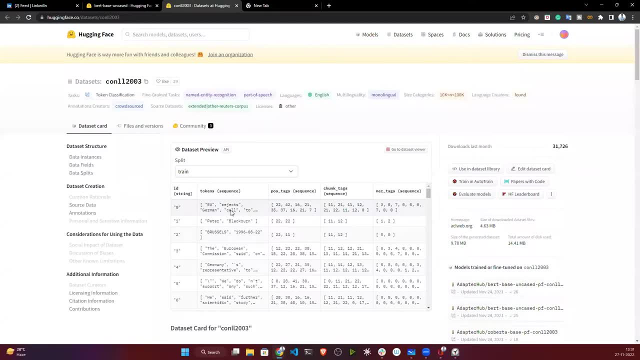 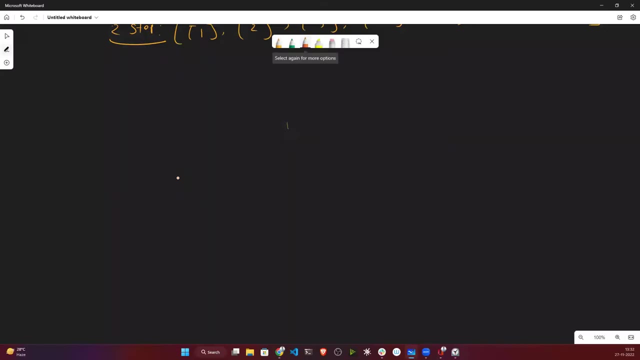 what the label mean. actually, they have mentioned, like: b person, i person. okay, b organization, i organization. what does it mean of b and i? okay, let's talk about so. here you have six, six level, okay, six level. first of all, you have object, object- okay, that is represented by o. then you have something called b par. 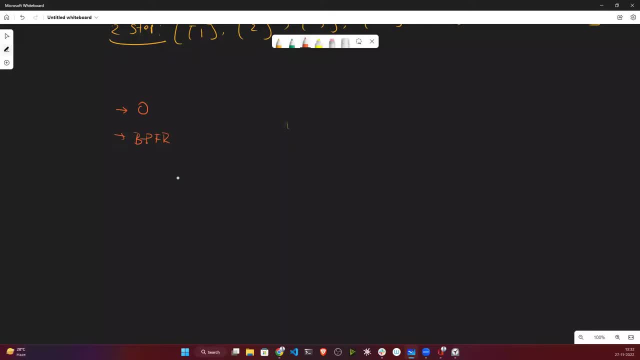 okay, b? per you can talk about so. or you have ipar, okay, so that means, uh, your, what is b? b means beginning of the word. okay, suppose p? e? r is what it's like: a person, nothing, but you are tagging as a person, but here you are mentioning b. 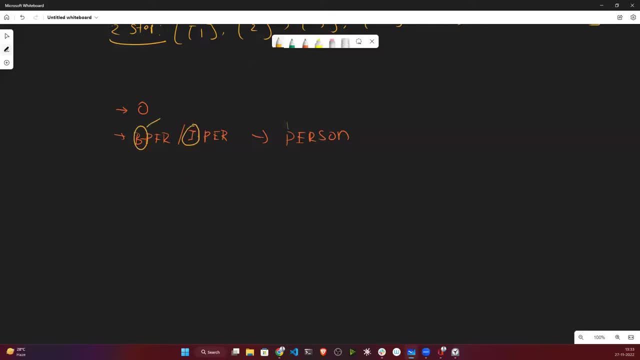 and here you're mentioning i okay. so this b means beginning, beginning of the sentence, and i mean inside of the sentence. okay, now, how? let me give you the same example. now, if you see here bill gets, what is bill and what is gets, guys tell me what is the entity of bill and gates. 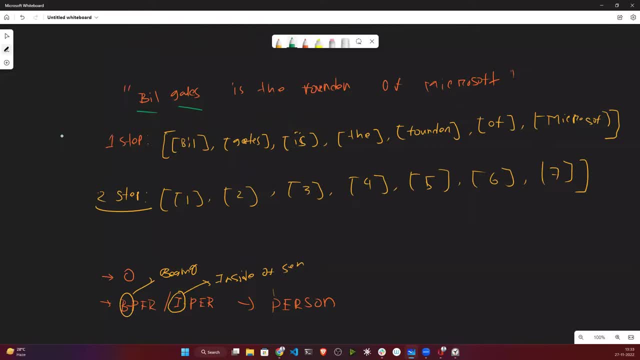 person, right. but if you see, bill, it is the start of the word, right, guys? beginning of the beginning of the word, right. so that means you can annotate this one as b part. okay, and gates, you can annotate as i per. that means beginning of the words and inside of the words that means beginning of the person and inside of. 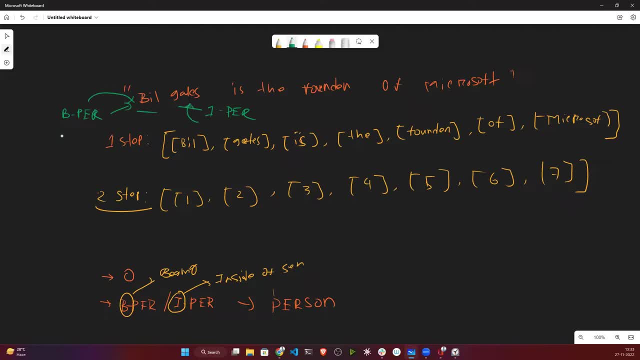 the person. is it clear or not? just tell me. this is the simplest explain i can give clear. now i think you got it. what is b and what is part? okay, everywhere. if you see here b, i has been written. what does it of mean? just focus on this one now. what is the mean of misc, misc and uh, there is. 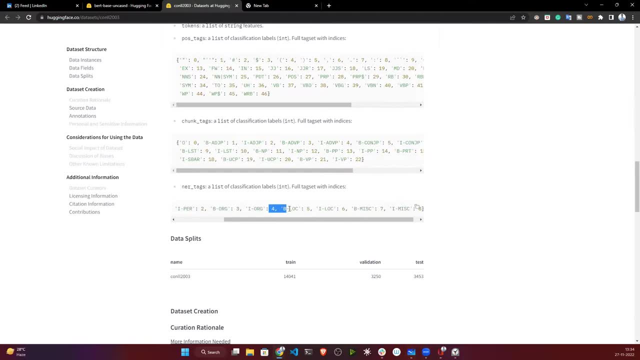 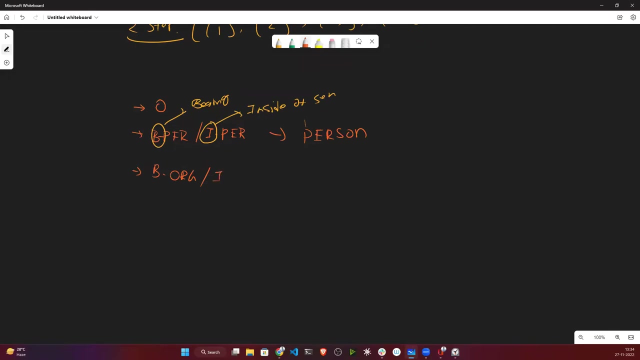 another one, one l-o-c, okay, o-r-g. let's discuss, like, what they are representing by that. so again you have something called uh. here they have written b, org or you can talk about i-org, so org means nothing but it's organization, okay, and uh, and what is b? b is like beginning and i is like in the beginning of the sentence. 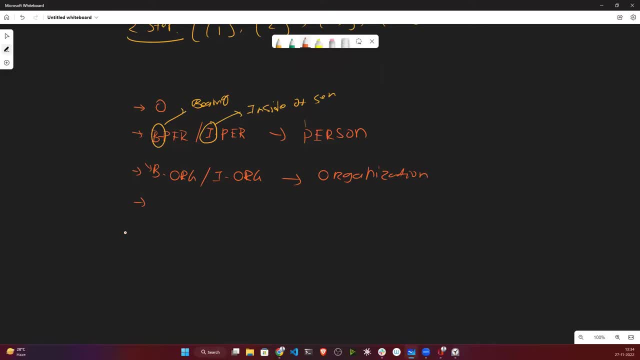 like inside. okay, if some organization is starting with like uh, beginning of the sentence, so you can annotate as b organization, and if some organization is inside of the sentence you can notice i, i organization. okay, now you have something called b location, b lock and i lock. so that is means 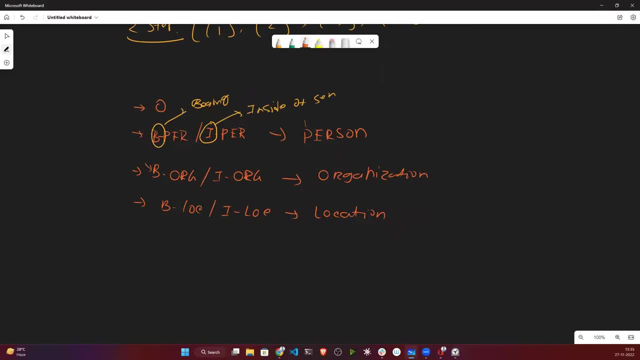 location. okay, you want to represent. and at the last you have something called b misc, m, i s, c and i m-i-s-c. that means miss uh, play neos entity. okay, so misc means uh, miss uh, selenius and t. okay, so that's actually you have. 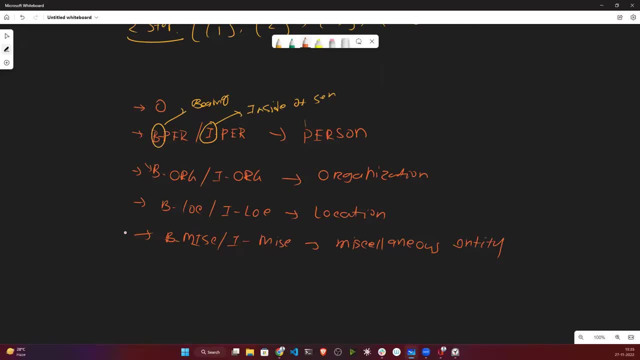 how many classes you have if you count, uh, one, two, three, four, five, um, i think, yeah, it should be five. yeah, so you have here actually five classes. okay, five classes. but if you see again, you are representing as b and i. okay, so you can talk about like how many classes. 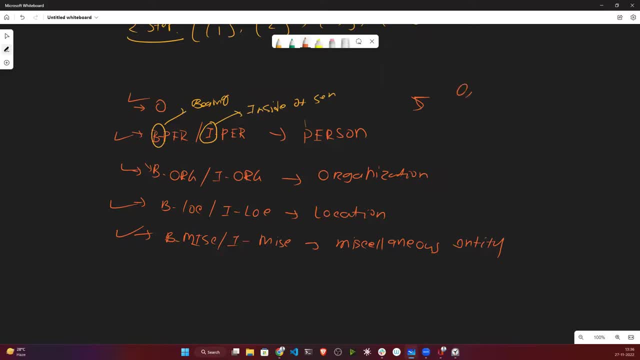 you have objects, you have. you have b person, two, okay. then you have, uh, b i person. that means three, then b organization, four, two i organization, five, then six, seven, eight, nine. okay, you have nine classes here. okay, but if you see as like a unique entity, you have like five classes, but here you are mentioning b and i. so 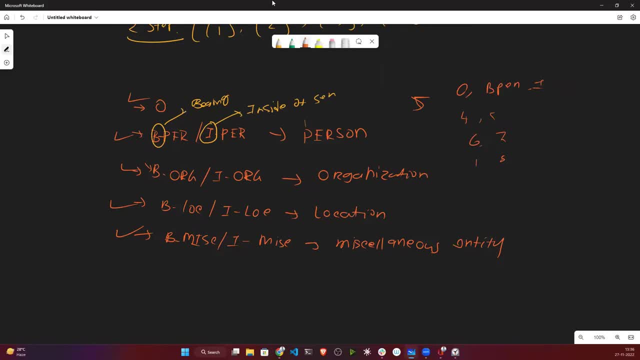 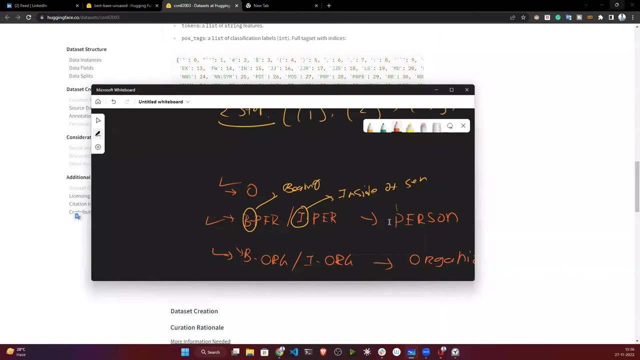 it's becoming nine. okay, so here, if you see uh, let me show you. you have nine entity, uh, one, then two, three, four, five, six, seven, seven, eight, nine. okay, i think it should be clear how they have annotated their data and how they have created this csv file. there is: 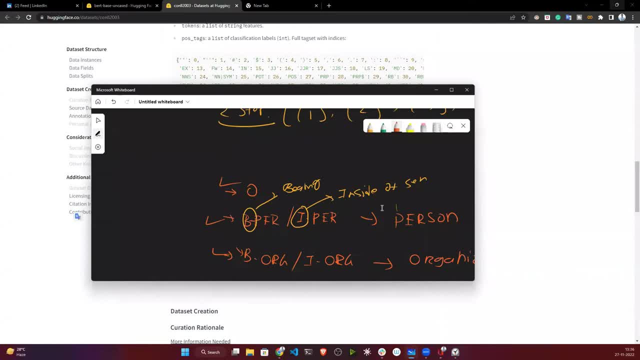 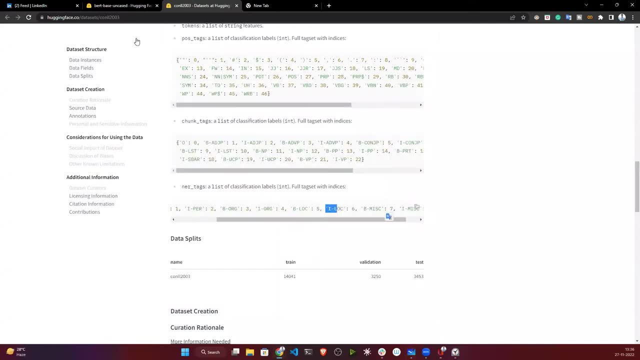 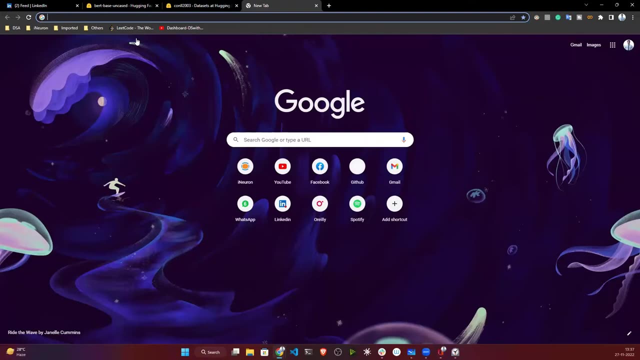 okay now if you want to do your own annotation. okay, any other notations? so there are various tool. i think i already uh like shared with you some of the tools, like around five to six. there is uh like various tools like species there. then protégé is there? okay, there is one free tool. any annotation? okay, if you just search any annotation. 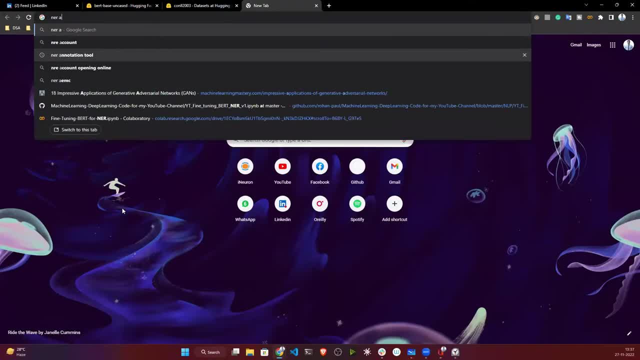 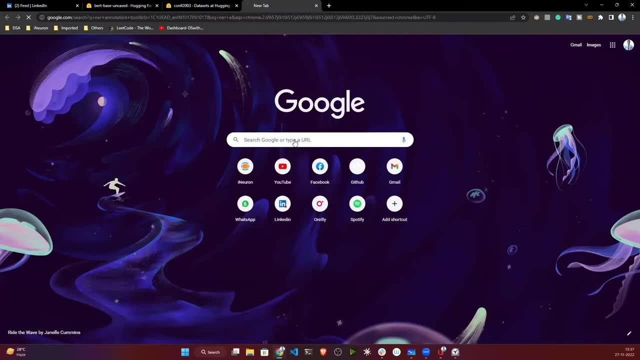 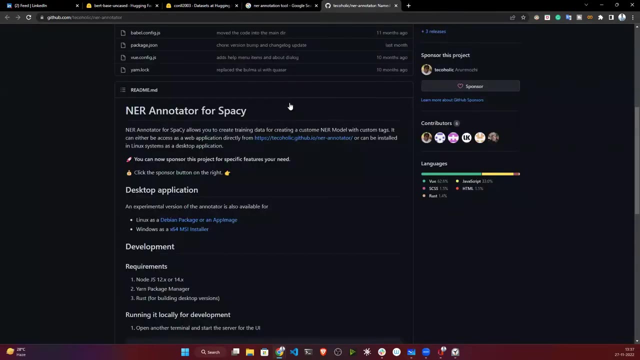 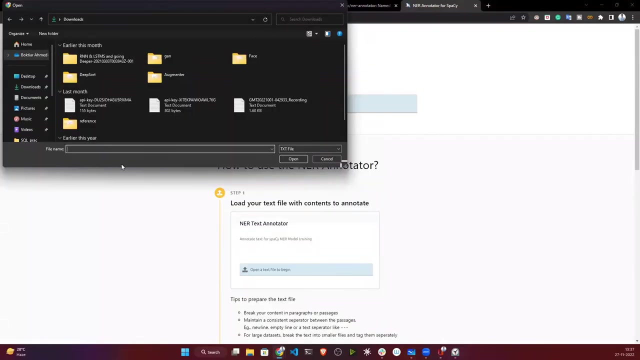 uh, there you will get one github, just open it up any annotation for space here i think this one, yeah. so there is a like one hosted app you will get if you just open. so here, basically, you can uh upload your file. suppose, let's upload some of the file. let's upload this one. this is the txt file. 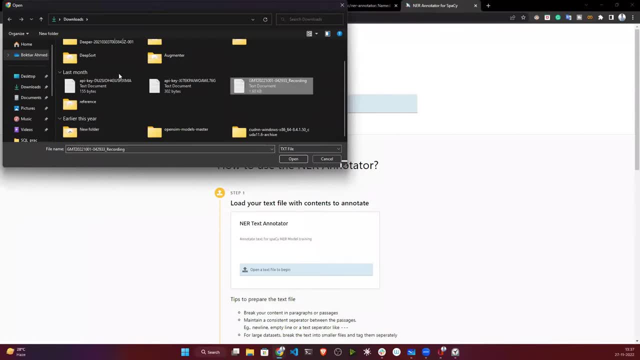 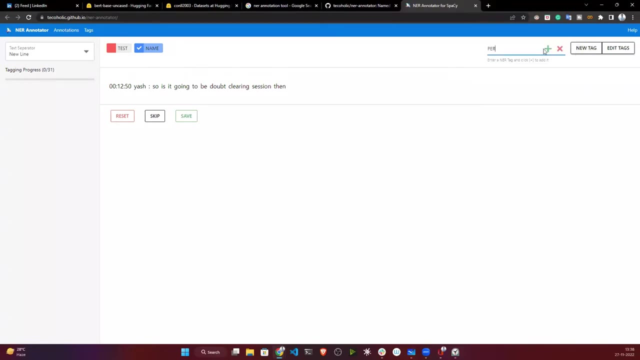 and here, suppose this is one. this is your text. okay, now you can annotate. so, first of all, what you need to do, let's delete. these are the thing i don't need. i think how to delete. let's create some new tags, suppose let's give as a person, okay, so now let's select person, and who is person here? 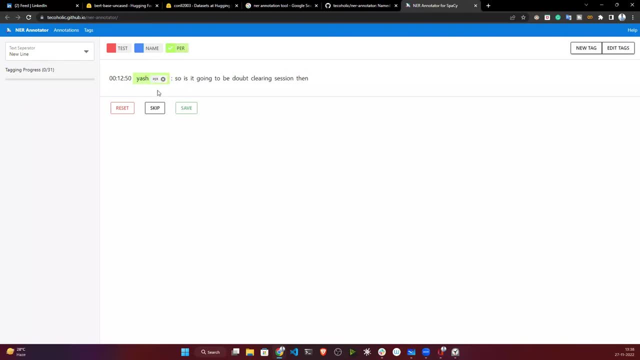 yash. so now, if i select person, select yash, okay. so yes, has been represented as person, okay now. so how we can annotate: let's give. give it as objects, okay. that means: o let's select, o. this is also objects. this is also objects. this is also objects. you can consider. this is also also objects. okay, that's actually. you can annotate. 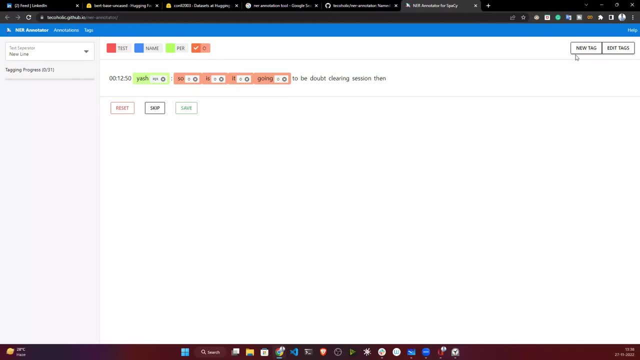 suppose there is some organization is written. okay, just create a new tag called organization, org select. okay, suppose this is organization. let's consider this organization just select as organization. okay, now, once you will save, okay, you will have all your entity. okay, you will have all your entity. like that is it clear guys, yes or no? 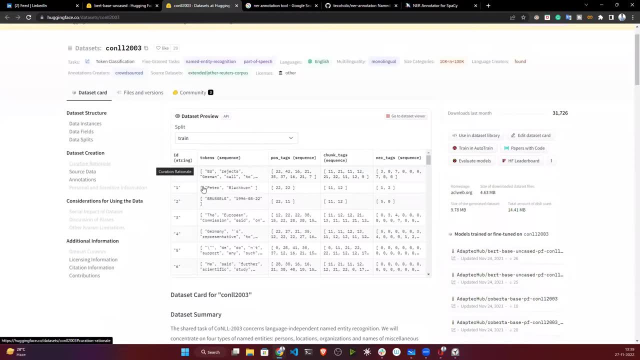 okay, now i think you are pretty much uh like family with the data, how they are prepared, because i'm not using any custom data here, like i'm not doing annotation, because nlp annotation is like very much time taking. so that's why you should always use some like annotated data. 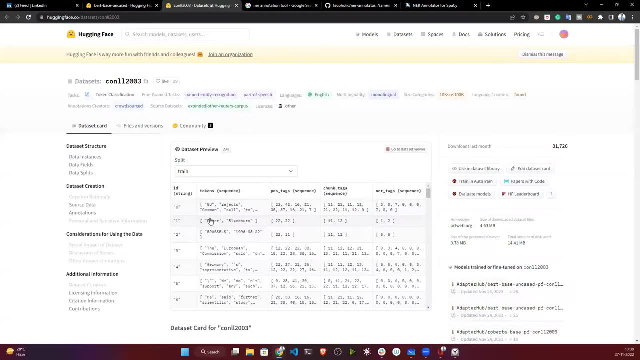 because it's not like a computer vision you are doing. uh, because nerc, you have to annotate each and every words. okay, it's like very much time taking. so better if you are using existing data. okay, so that that's why nlp is like used costly in the market. okay, you will be getting these kinds of. 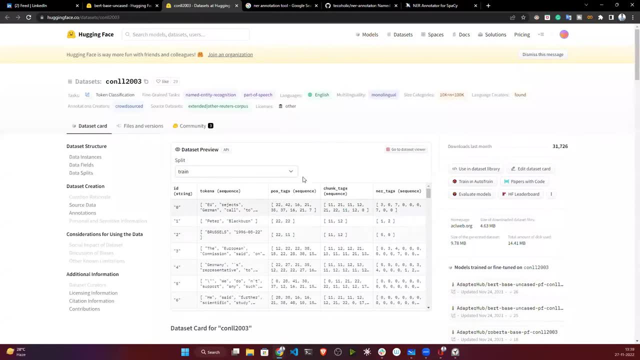 data in kaggle also you can download, you can do your job. but is it? it is available in hugging face, because hugging face has already like all the things, it is like one of the best uh organization you can refer for the nlp, so i'll be using from from the hugging face itself. okay, so i don't have. 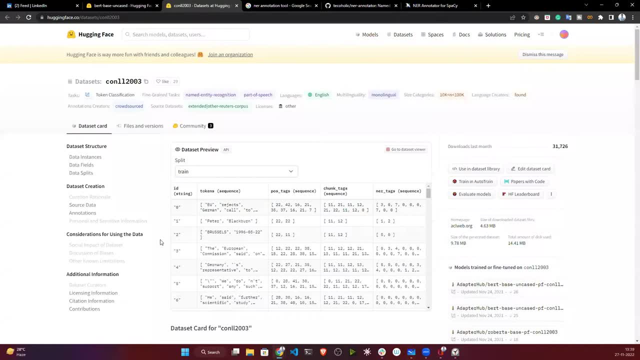 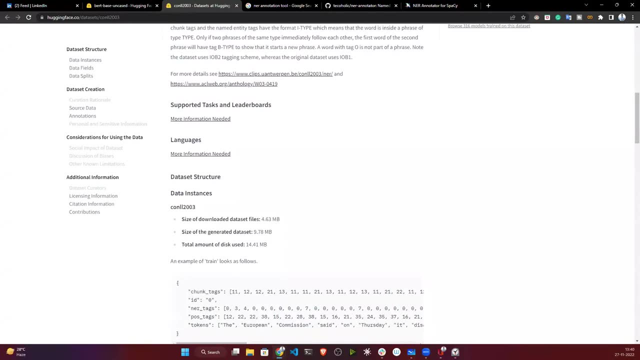 to download it so i can call it from api only this data. i will show you like how to call it. okay, you can read the data set summary. i will. i'll share the link with you. just keep the link. okay, you can see like many data set a layer there if you just click on the. 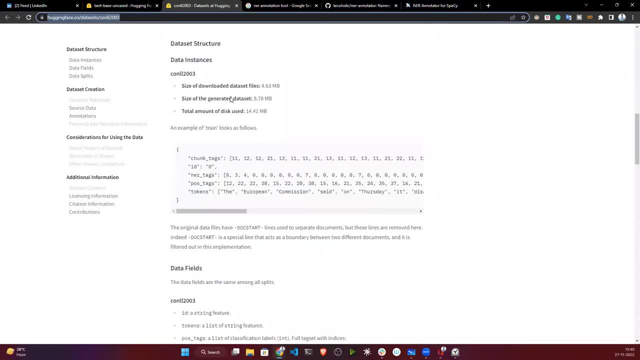 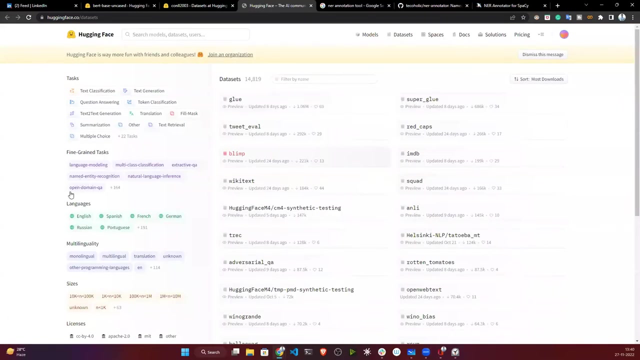 data set, not only this one, there are many data sets. suppose which task you want to select. suppose you are doing token classification. just select token classification, then you can select a task. i won't be selecting any. which language you want? i want english language, then your this one. you can select size, how, how many examples you want. okay, you can select. 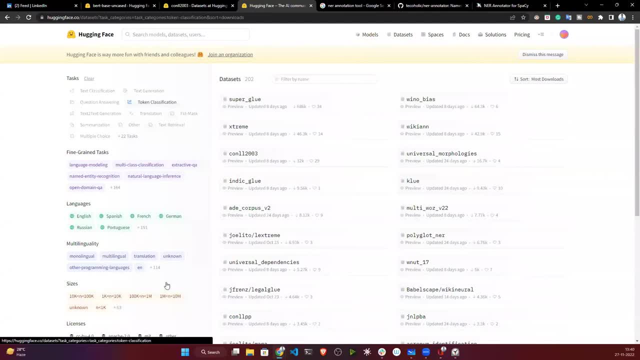 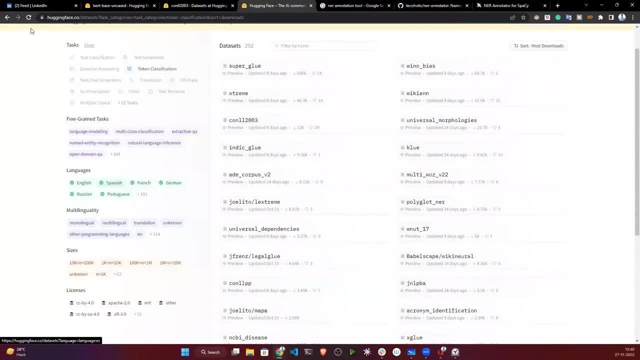 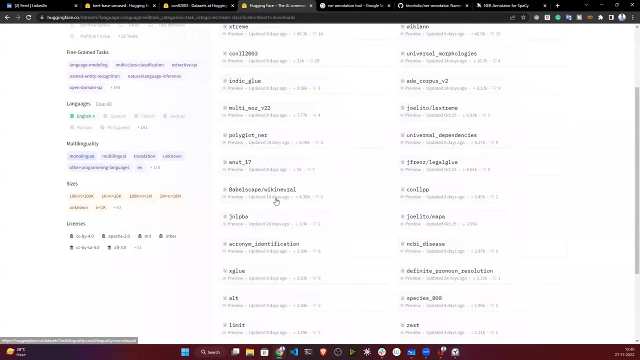 and license you want. okay, and after selecting, these are the data you have. okay, you can click. click on any data. so this is one of the data. it is called uh con ll lpp. okay, this is one of the any data. okay, now i think you got it, like how to use hugging face website to select any data. 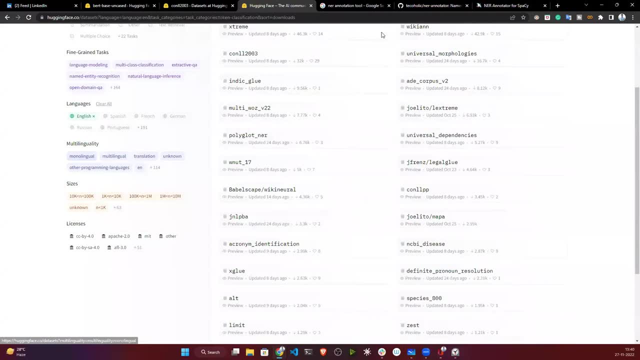 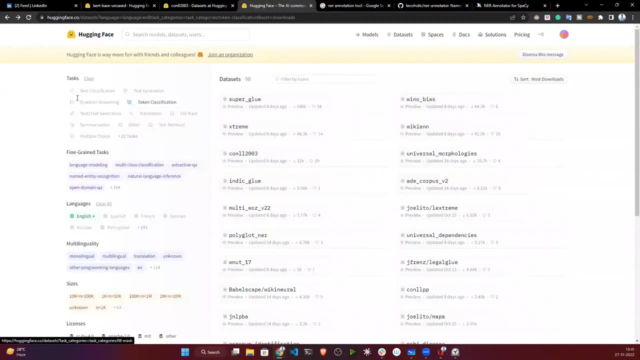 suppose you want any model. just click on the model, select your task. suppose you want to do uh. like token classification? again click on the token classification library one suppose i want pytorch. i will be selecting pytorch. okay, data set you want to use. suppose i want to use uh. 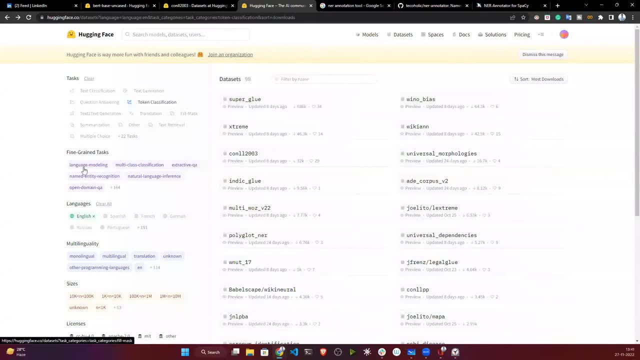 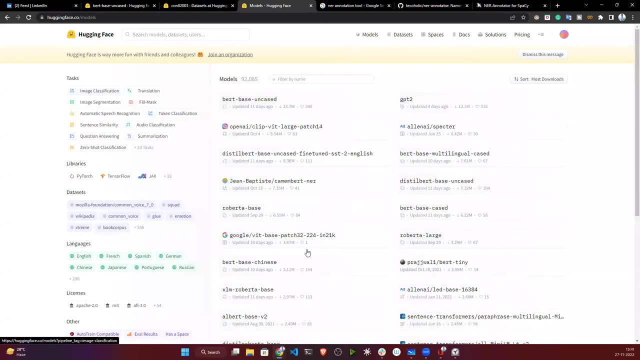 all the data set. i'm not selecting any language, it's only for specific english. okay, i'll be getting all the model i want. okay, birdways, ner, robota. okay, every model transformer based model, i will get. so what i will do? i will just click here. code would be available here. how to. 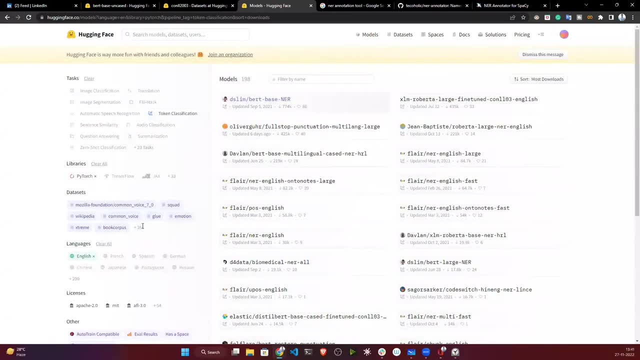 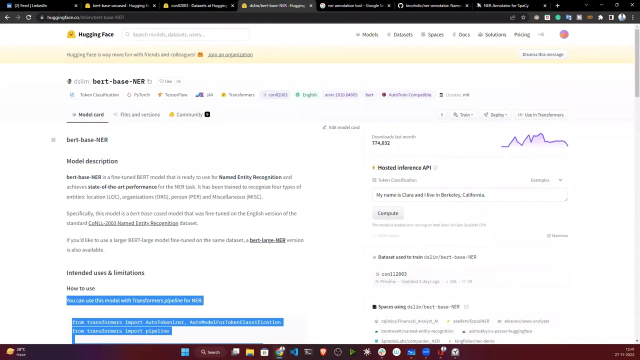 use the code and all everything they have written. okay, tutorial is also there. okay, it is pretty much easy to use one of the like best organization you can talk about. okay, now let's start our task. so, first of all, i'll be creating one notebook. i will share the code. okay, at the last, just try to focus on, like, how i'm doing this one. okay, how. 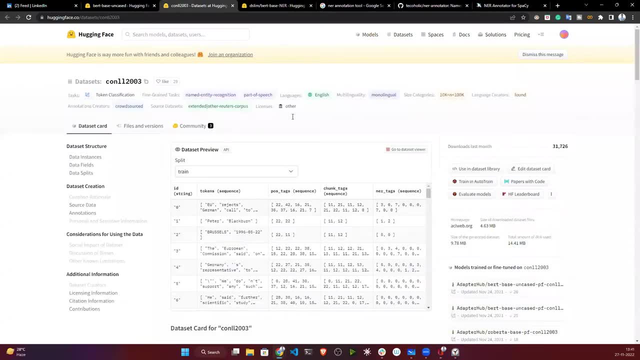 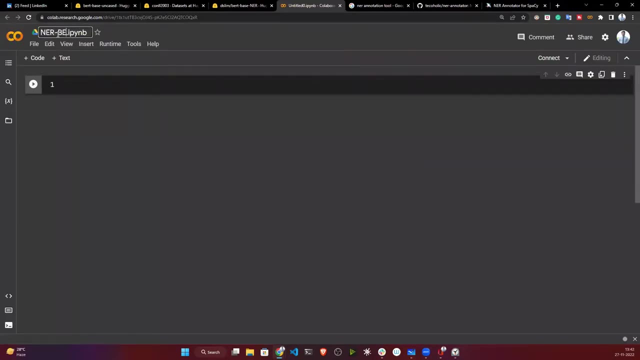 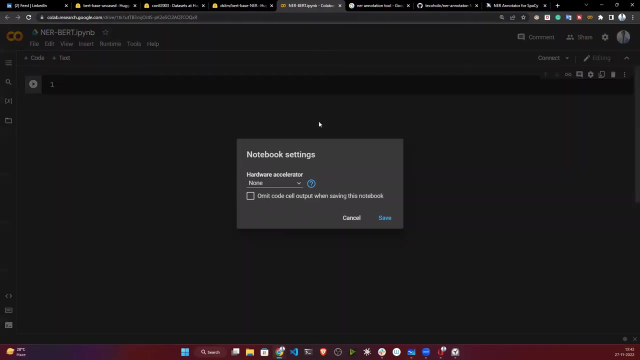 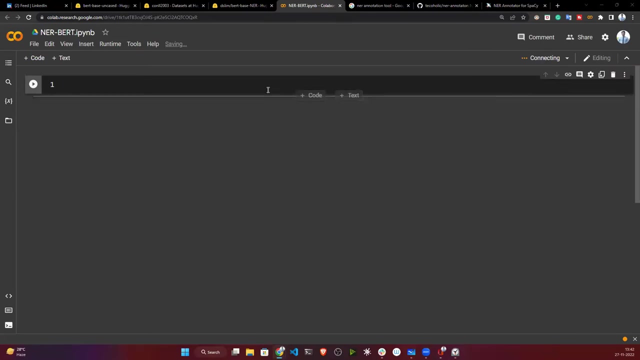 to find in your barter model and how to train your own ner. okay, first of all, try to see that, that one. so let's name it: uh, ner. but okay, so make sure you have selected gpu as runtime and now let's connect the notebook. okay, so here, suppose, suppose. if you want to use hugging face, okay, hugging face, okay. 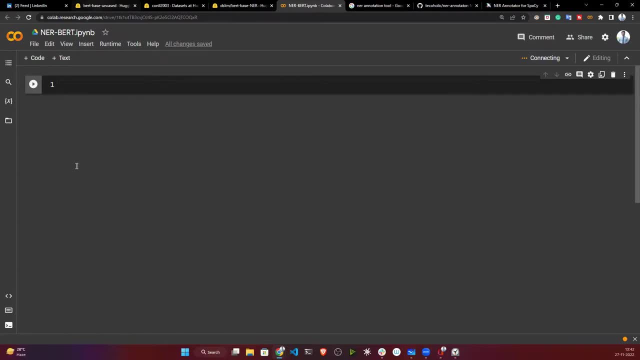 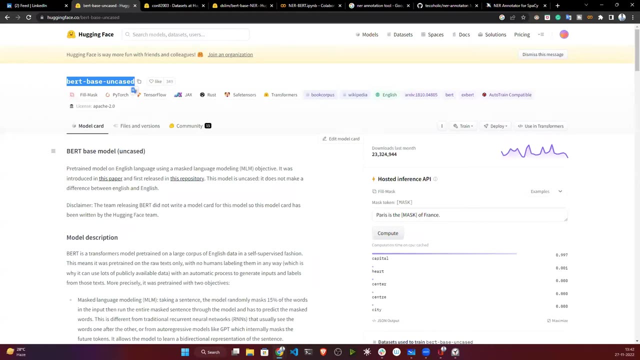 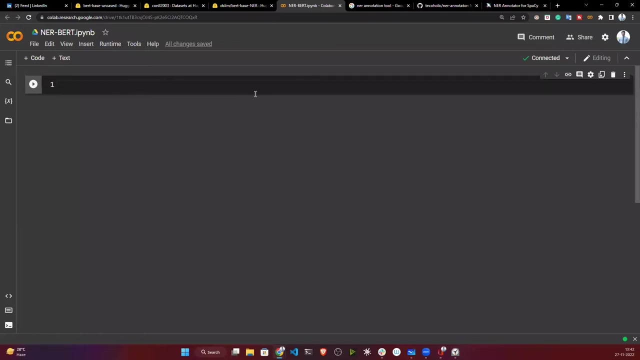 face this API. so you need to install some library. okay, so what are the library unit? so let me copy paste from here, only so this library unit, like unit transformers, unit data sets, unit tokenizers, and you need this egg. well, okay, so these are the packages you need by default to use hugging face API. okay, 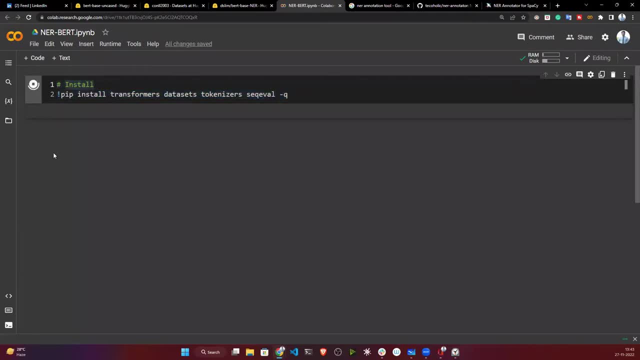 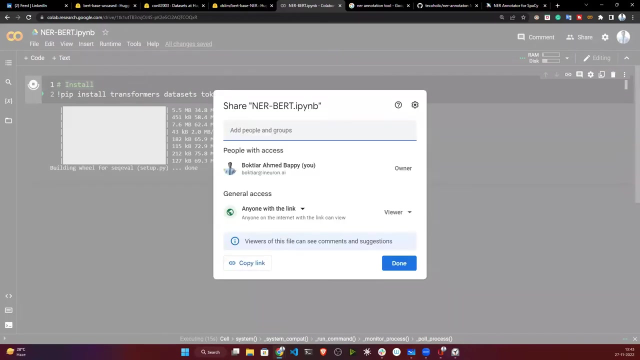 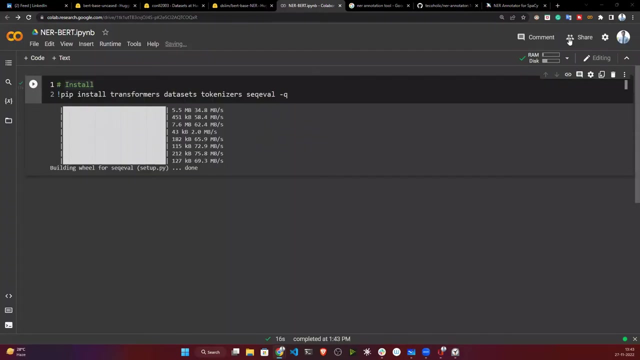 now let's install. yeah, I will share the notebook. okay, I will share the notebook with you, no issue, I'm sharing. even after the session, I will comment each and every line. I will share with you the like detail notebook, one which I have as a reference. okay, you can execute with me. okay, as of now, I think it is accessible, right, guys? 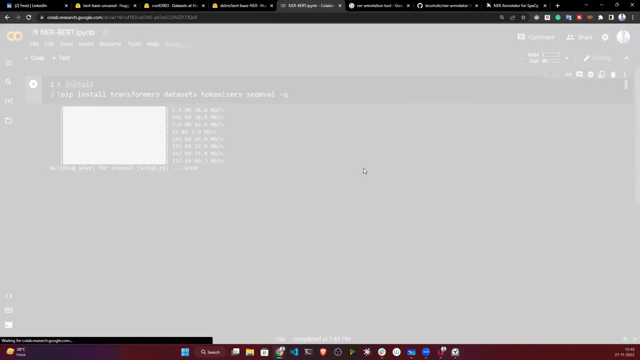 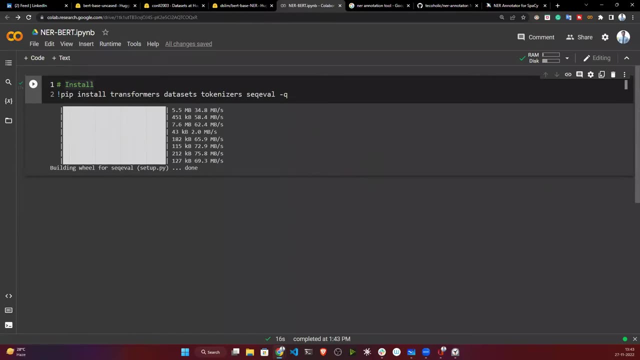 can you open this? you, okay, so this installation is being done, so these are the thing you need. now you need to import some of the libraries, so let's import. so first of all, you need to import the data set number you need from transformer. you are importing, but token. 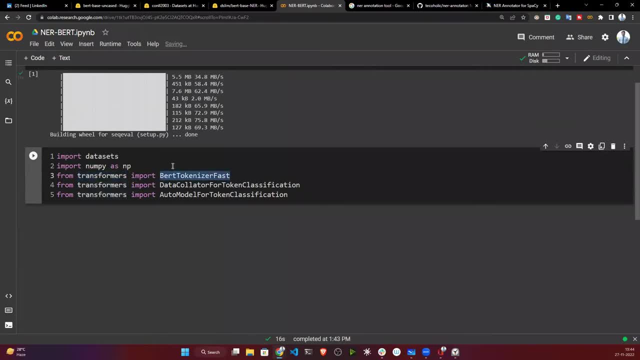 tokenizer, for you need to import the data set number you need from transformer. okay, so this is the device. okay, so the concepts of backstory first. okay, so I think- sorry- has already discussed transformer based module. suppose if you are using any architecture they has that individual tokenizer so you don't have to use some other tokenization. okay, because whether 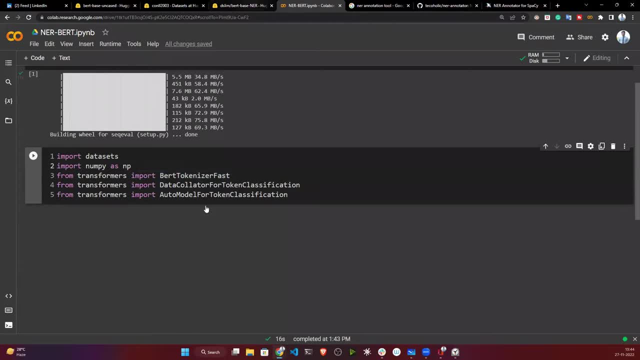 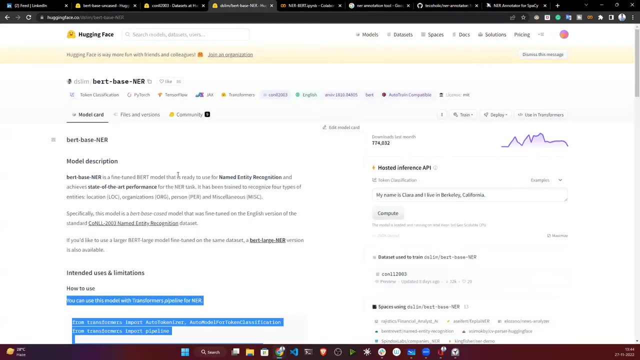 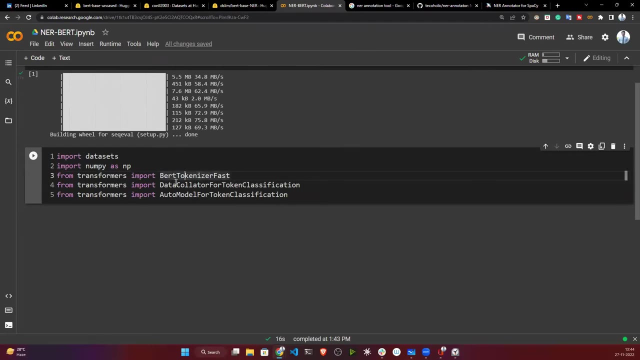 you your body splitted or not, it doesn't matter. if you see this, what is already splitted, it doesn't matter, okay, it is already tokenize, but but has their own tokenization technique, tokenization, okay. so that is why you you always need like which architecture you are using you. 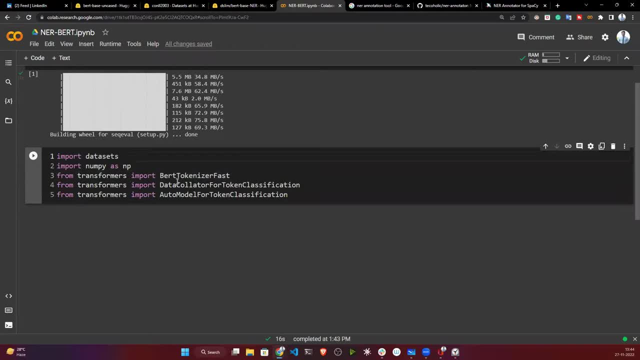 should import their tokenizer. suppose i am using, but so i'm importing but tokenizer, suppose you are using. uh, some other one, suppose robota? okay, at the time you need to import the robot tokenizer. okay, so every architecture has their own tokenizer. okay, then, what i'm importing? i'm importing data. 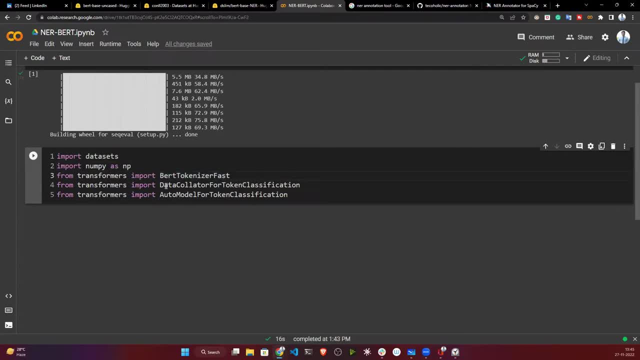 collector for tokenization, token classification- okay, so data collator for token classification. this is the library i need because, uh, whenever you will be training your model, at that time you need to pass this as objects. so what it will do? it will apply some of the augmentation technique. 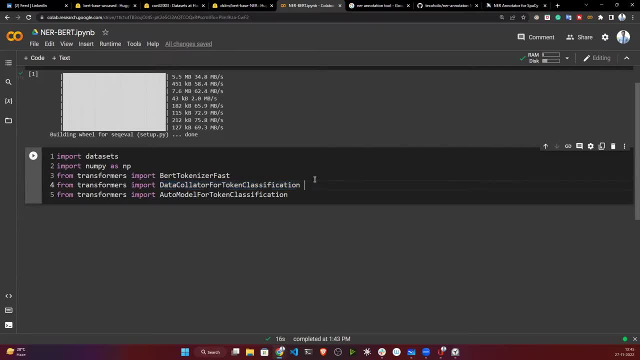 okay, in the runtime. suppose you did image classification or, uh, object detection, so there actually it was applying some of the augmentation in the runtime. guys, can you remember like you are doing sharing operation, you are rotating the image right, so in nlp also you can do it okay using this, this class, actually okay. 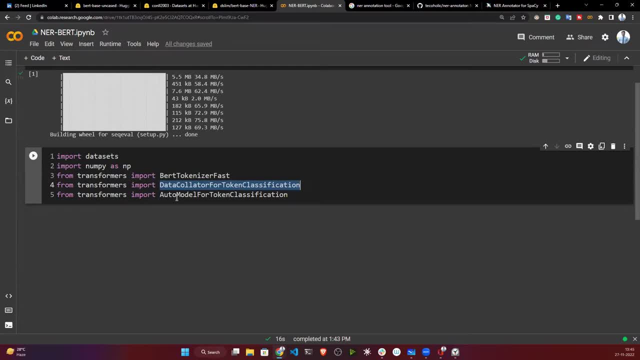 now auto model for uh, for tokenization. this is this api actually, this class actually responsive for for load my model. okay to my memory. okay, so i will show you like how to call it. now let's import all the library. okay, it's done. okay, so now let's download our data. 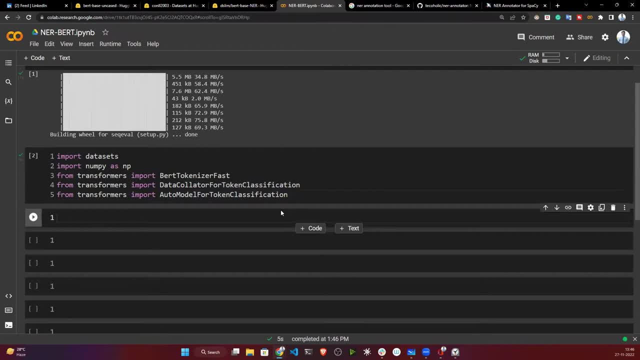 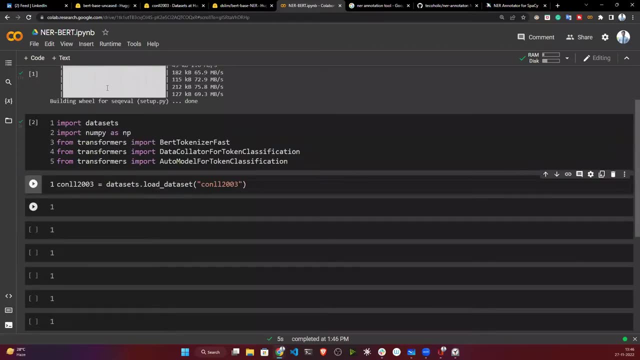 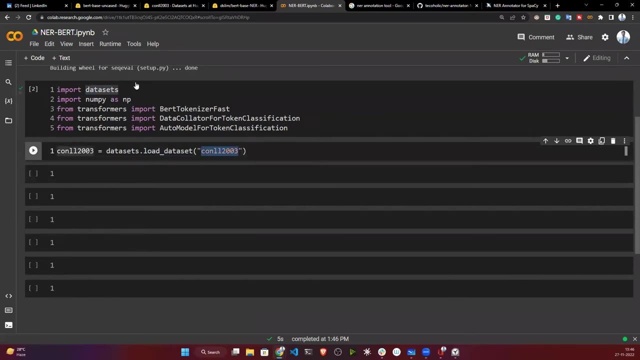 so this is the code to download the data. so what i'm calling? i'm calling data set dot load and i'm passing my like data set name. so what is the data set name? this is my data set name. okay, con ll 2003. just copy the name and paste it here. okay, any name, suppose, if you are. 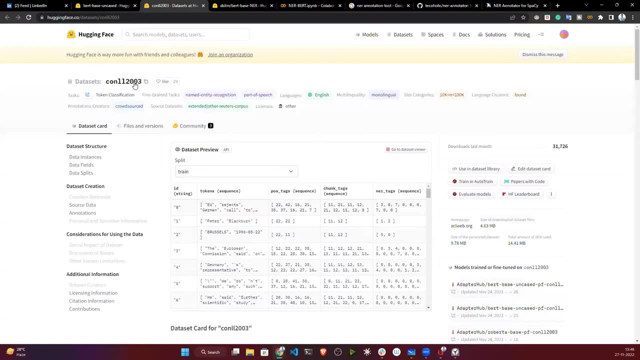 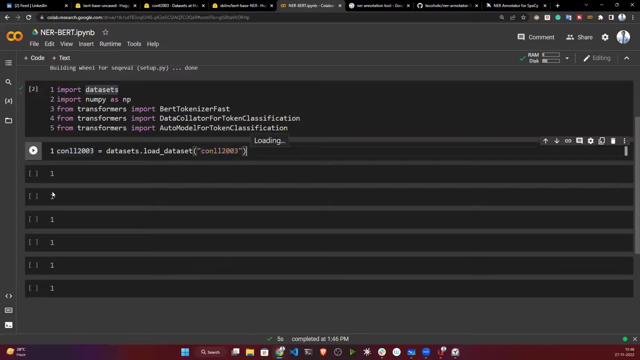 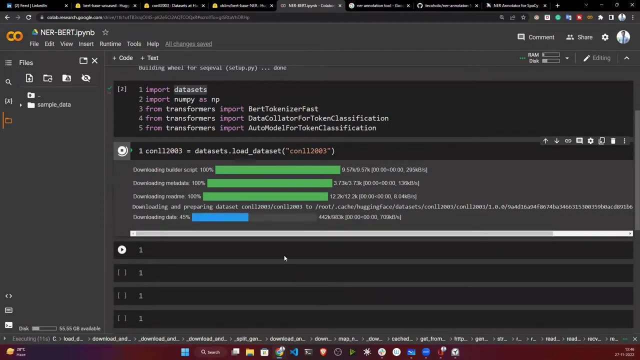 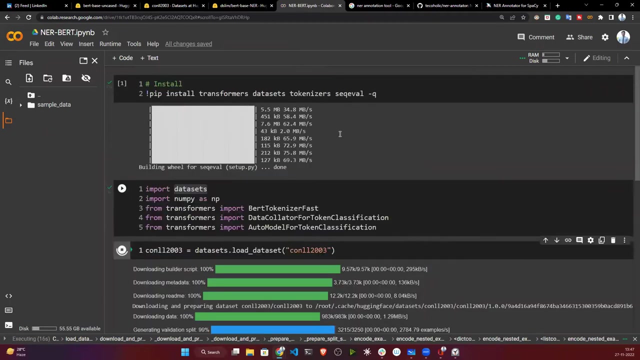 using any data from hugging face. just copy the name and paste it inside this load data set. it will download. okay, now let's execute. data collator will help you to do the like augmentation- okay, like runtime augmentation- and it will also help you to load it as a batch images. you can talk about that later on, so let's. 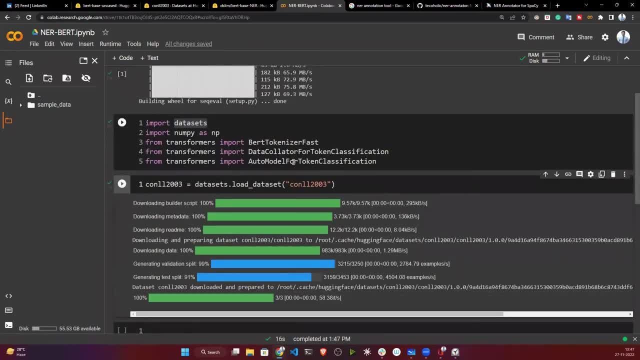 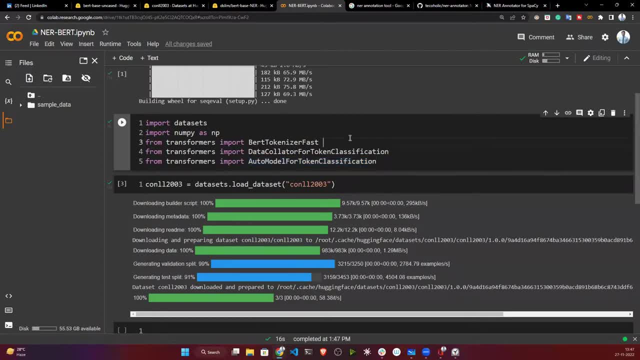 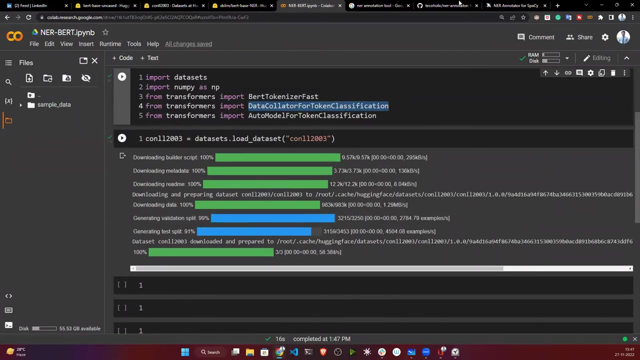 actually you need to apply some of the augmentation. it was happening in the runtime: opposed, rotating the image, sharing the image, copying the image a little bit. okay. the same thing you can apply in nlp also using this data collator for token classification. okay, okay, augmentation you can talk about, like some random flipping would be there. suppose this is one. 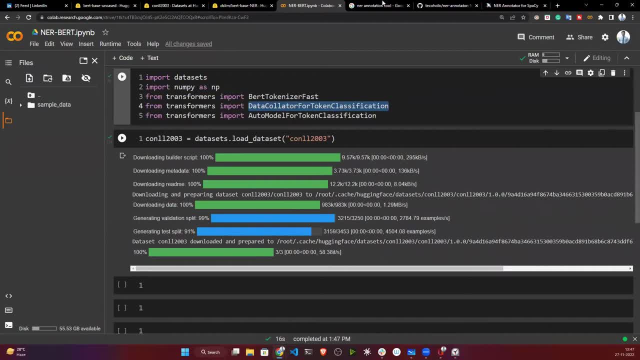 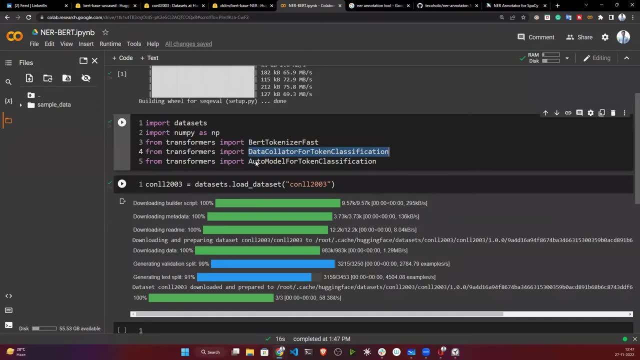 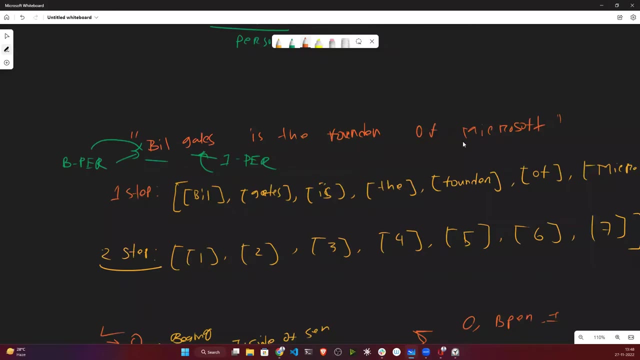 uh, suppose. there i think i showed one example: bill gates is the founder of microsoft. so what it will? it will flip some of the words. suppose, uh gates, bill is the founder of microsoft. okay, that's kinds of like augmentation you can talk about. okay, yeah, so data is been, it is downloaded. now let's see like it will give you one. uh, you. 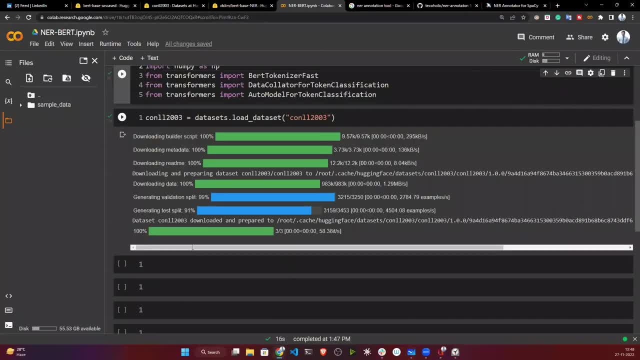 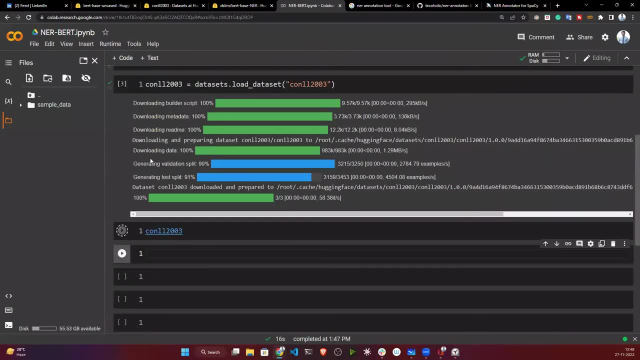 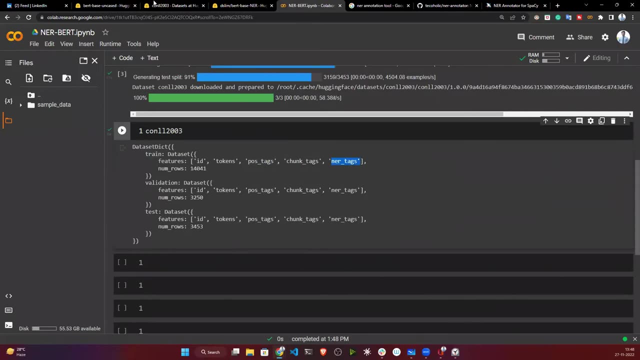 can say: dictionary data set, dictionary- okay. so here three like data partition. you have one is your training, okay, training data set. so inside training data set you have id tokens, parts of speech, tagging, chunks, tags, any attacks- okay, the same example you will. you can see here: okay, okay, now your testing data is already separated, see this. 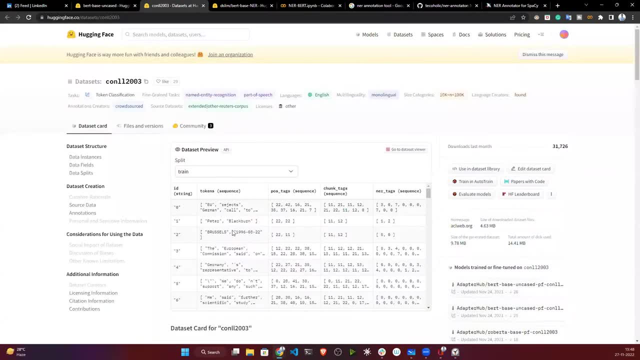 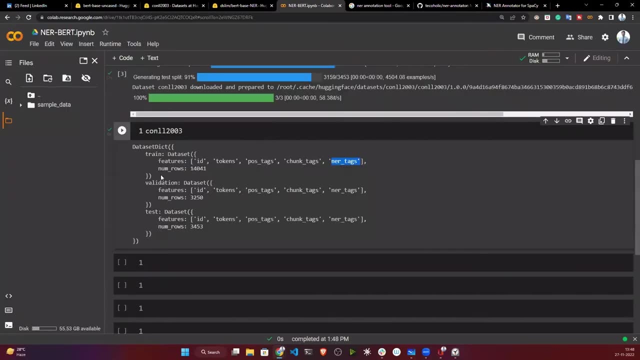 is the validation. okay, again, you have and how many examples you have. it is also will show you okay. so this is the format of like uh hugging face, like they have, like uh output the data like that as a dictionary format and you can take the data from the dictionary. okay, how to take, i will show you. okay. now this is the test. 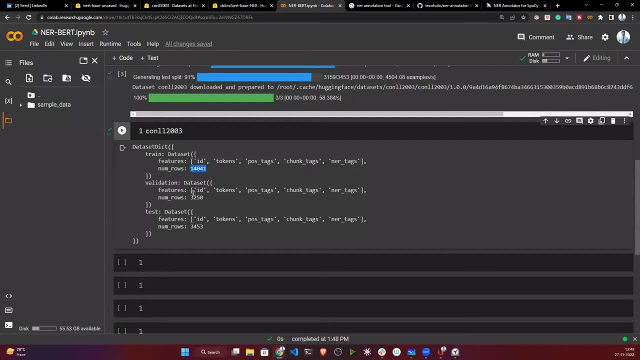 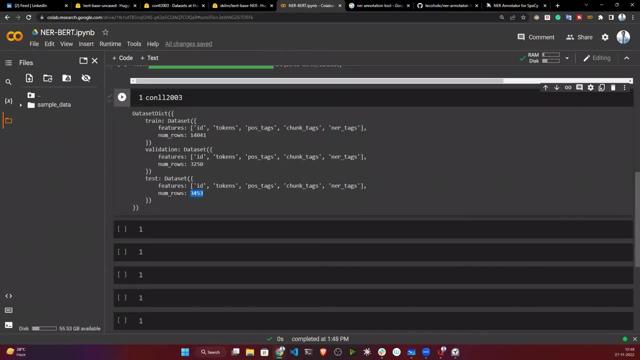 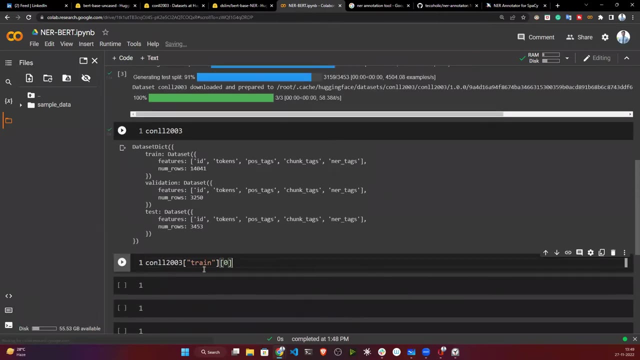 and inside test. you have that many of example. okay, now, if you want to see your train data how it looks like, uh, so you just apply this one. your suppose this is one dictionary- and if i want to take the train key, so i will call the train. okay, so what it will return? it will return all my 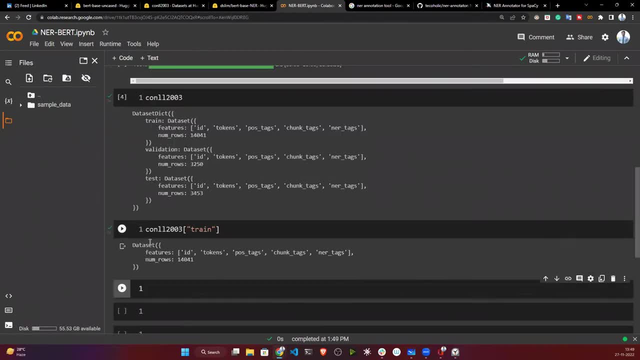 training data guys, okay, but i i want to see the first one, first example, because, again, it don't show all the data, because, again, if it loads, okay, then your memory will full. so this is one of the best thing they have done, unless and until you are not not. 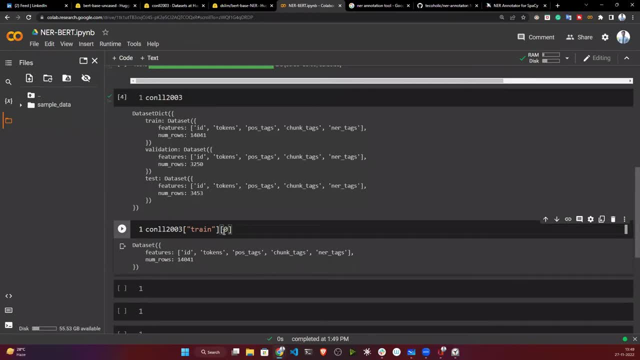 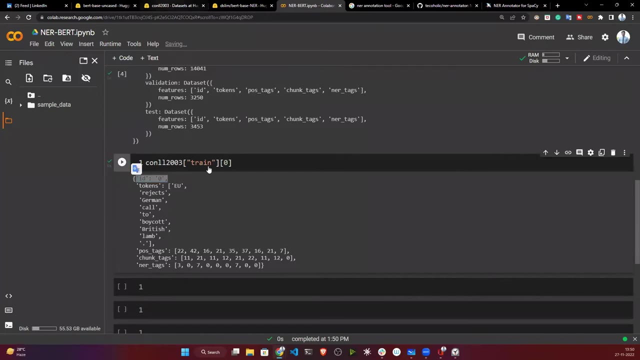 calling with their index. okay, it don't show the data, so now let's provide zero. that means i want to see the first example. okay, now, if i execute, now you can see the data. guys, this is id number zero. if you just compare with that id number zero, okay, uh, what is the tokens? token was: 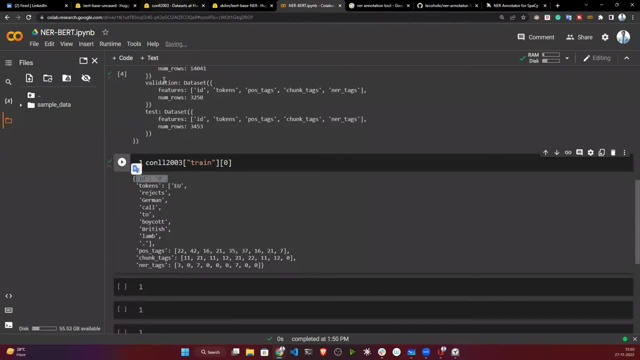 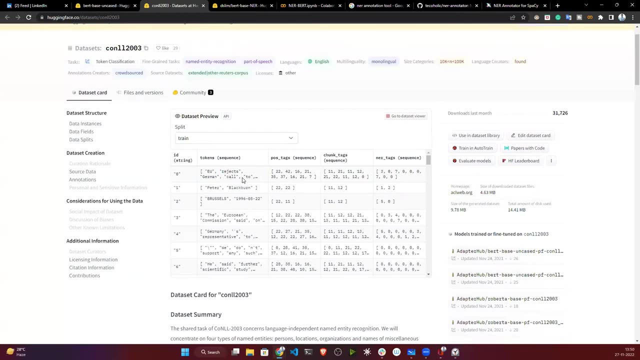 you reject german call to boycott? see here. okay, you reject german call to boycott. then you have what po pos tags. pos tax is also there. then chang's tag. okay, chang's tag is also there. basically it is represented as dictionary. okay, chang tax is also there. and at the last you have: 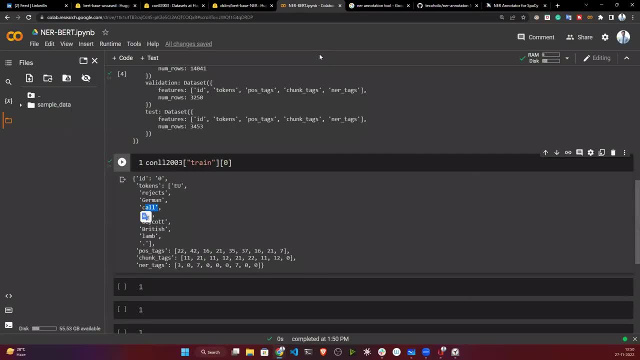 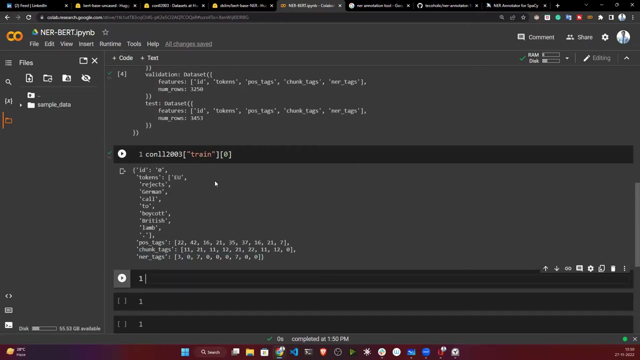 any attacks? okay, any attacks. got it. guys. how to call the data? how to see the data? okay, instead of loading all the things in a memory, i can load one by one. okay, and i can see as a dictionary output. suppose you want to see your test data, just provide the text. 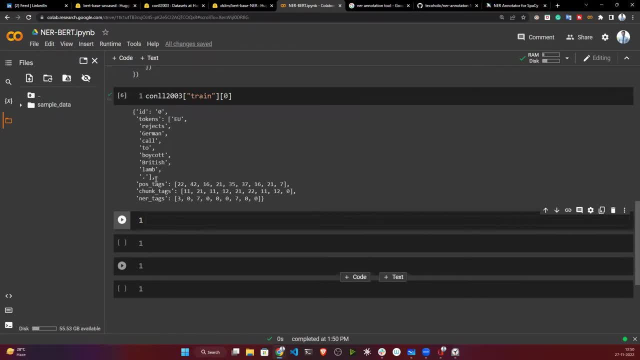 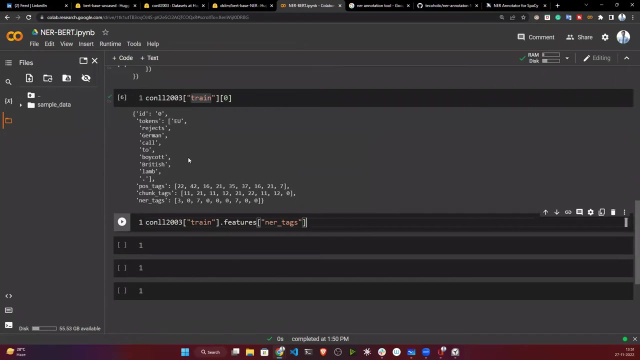 like key name: okay, test key name validation. key name: you will be able to see. now, if you want to see like what are the tags are available. so there is a code also just write: okay, i'm calling my train and there is a attribute code. call features: okay, inside features: just provide any attacks. okay, you want to see your any attack. 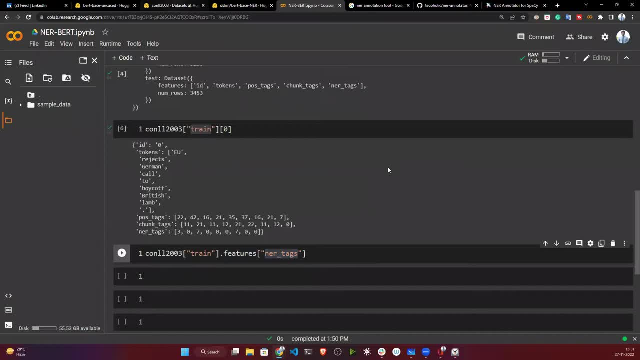 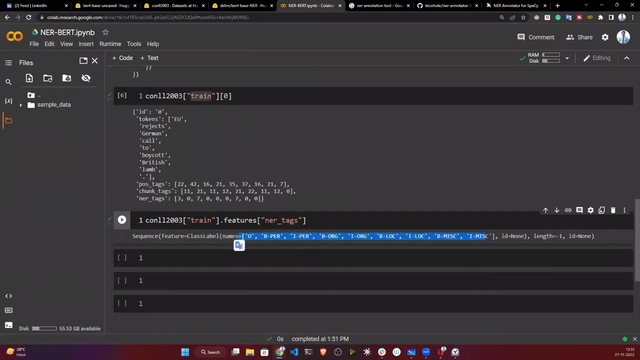 suppose this is one. any attacks i have, okay, and i want to see all the name. just execute, so you will see all the in-ear tags. okay, objects b person i person b organization. okay, all the near tags you will be able to see. okay, now, if you want to see the description of the data, it is also possible. 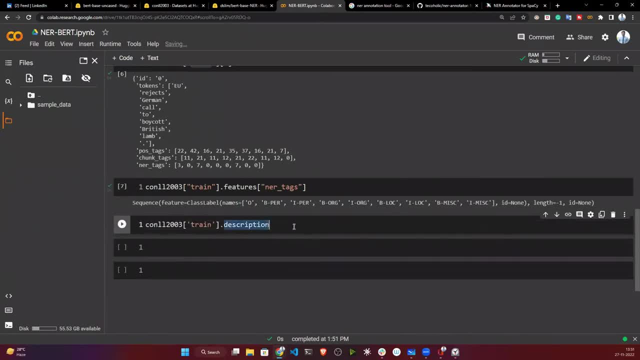 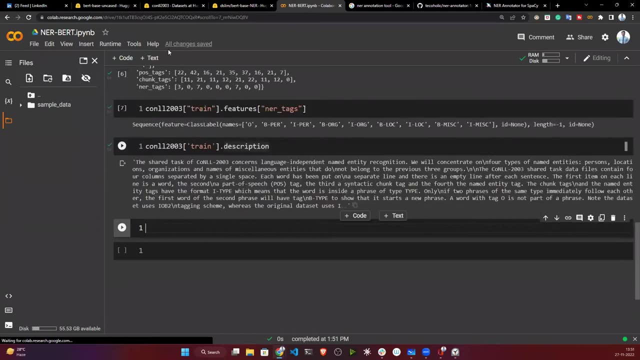 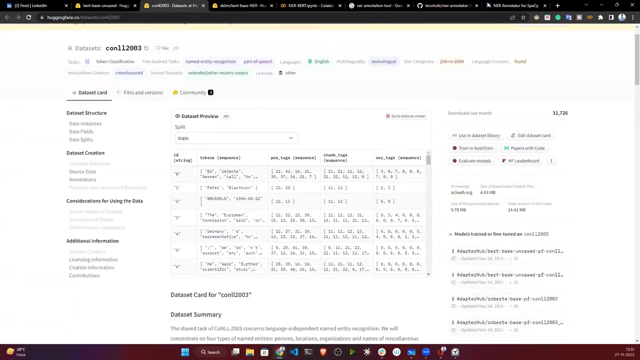 just call the description attribute, run it. you can see the data description is all about like, what are the things they have written here? okay, briefly, it will tell you what this data is representing and all okay. now i think you are pretty much like good with the data. any questions, or it is clear guys? 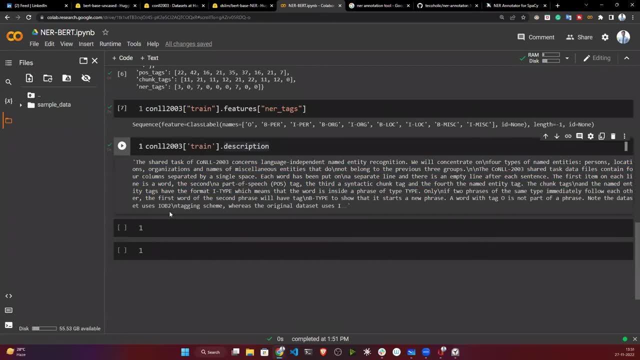 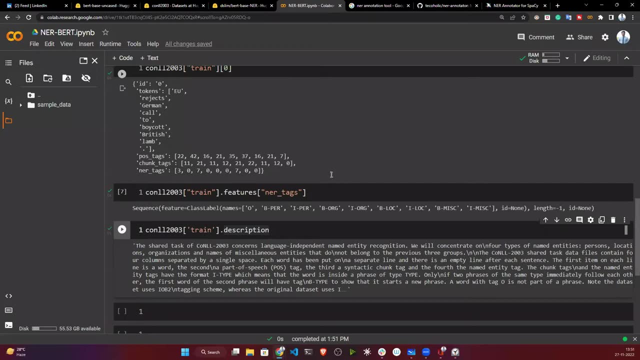 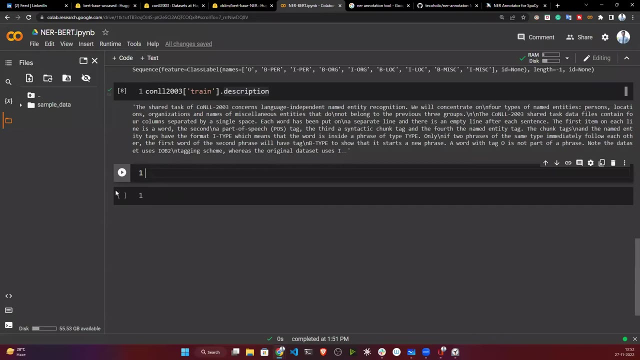 clear. okay, now just always remember some of these steps. whenever you are writing a test, you are using uh transformers- or you can talk about your uh hugging face. so after importing, always you need to initialize your tokenizer. okay, because i told you each and every algorithm or each. 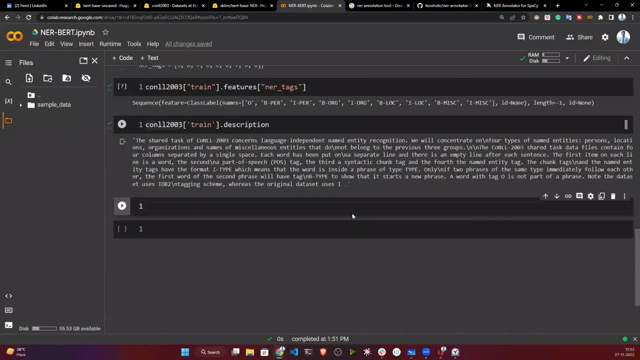 and every architecture has own tokenizer. suppose here i am using but based unkissed model. so this is the uh like hugging face model. okay, if you just go to the model. okay, suppose here, just click on the model and starts here like i want to use. but 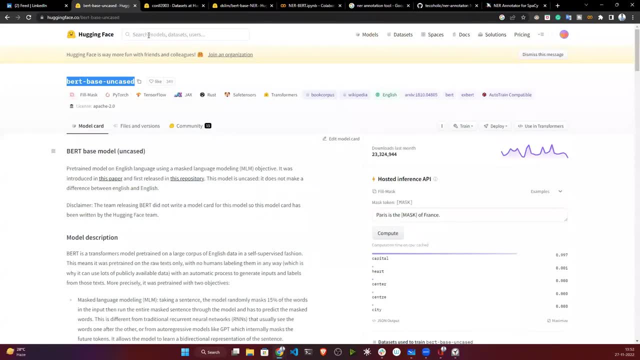 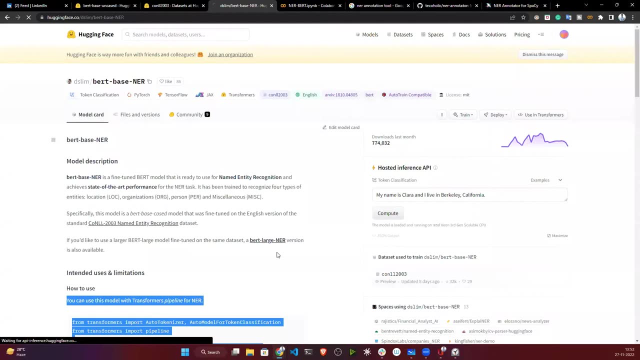 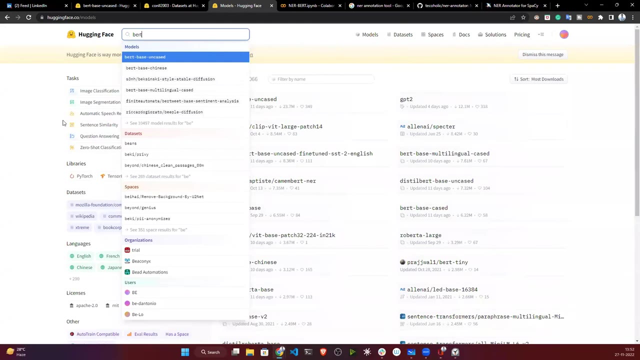 uh, base unkissed just starts here, so this is the link you will get. okay, so this is the model actually, but but this unkissed model, okay, so this is one of the like transformer based model. okay, so it has like like too many variant also, but with unkissed is there, but large unkiss is there. 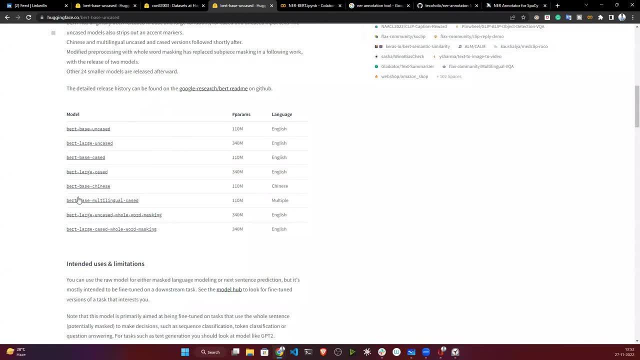 then small, large, then multi. okay, like it has like many variants, but i am using the first one which has, uh like 110 million parameter and the linguist language supported is english. okay, so, with your choice, suppose you want to use this model, just click here. okay, you will see the name of the model, so just copy the name and just paste it here. okay, and 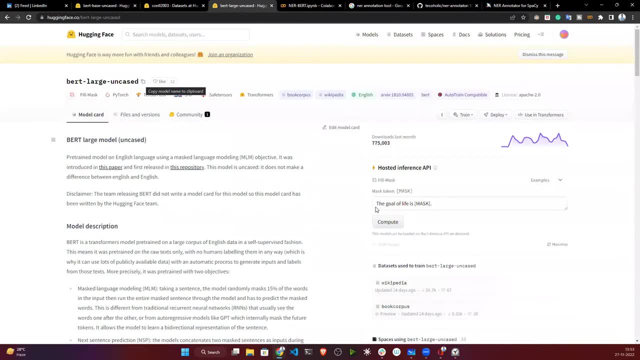 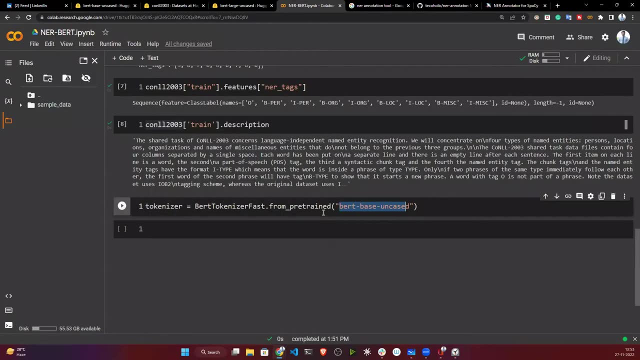 the same name you are passing as a, like you can say your model. okay, the same name. you can pass your tokenizer also, because i am using the same tokenizer from the same model, okay, so what i'm calling? i'm calling my bot tokenizer first. i think you know i have imported here, okay. 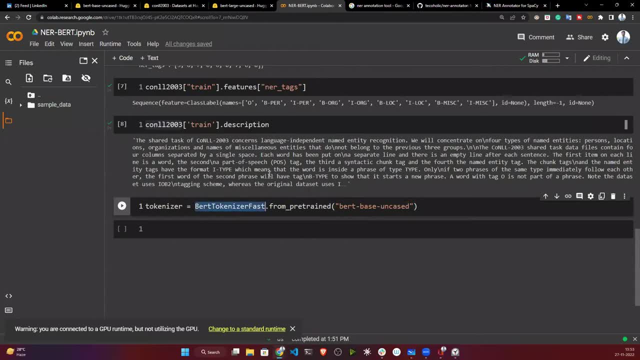 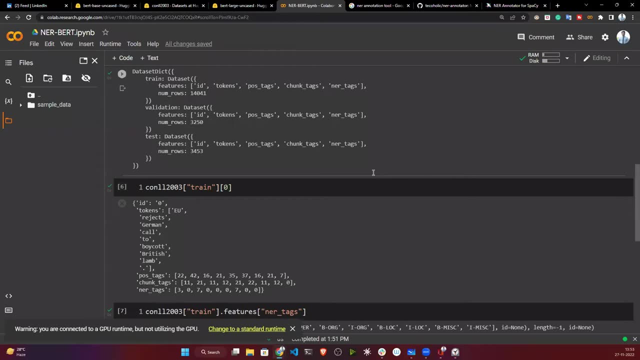 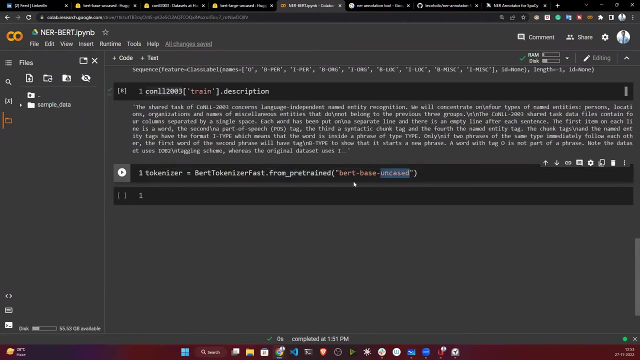 and there is one uh like method. you will get called from pretend: okay, because i'm using pretend model. okay, and i'm passing my model name, which model i want to use, okay, as my tokenizer. so i am defining, i'm using but best but based unkissed model. okay, so i'm defining the name. 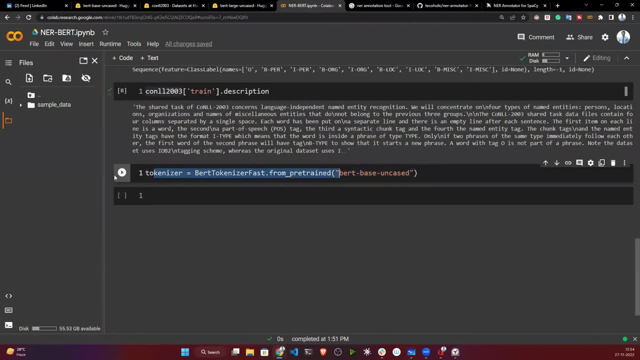 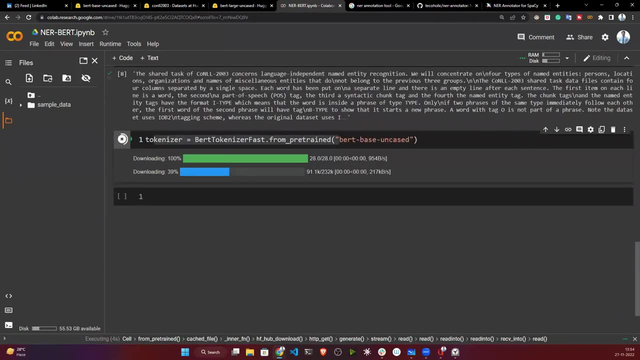 and i'm initializing my tokenizer. okay, now, let's run it. okay now, let's run it. okay now. just remember one thing: transformers are often pretend with the sub server tokenizer, like meaning: uh, suppose, if your input is like already splitted, it doesn't matter, but it will apply some of the like tokenization technique, suppose, how, suppose, sometimes, if it is. 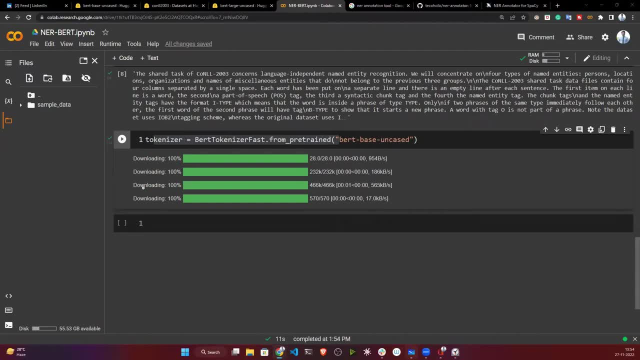 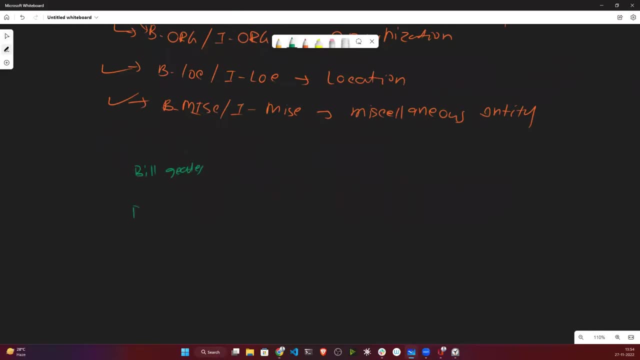 not able to understand the words. so what it will do. suppose there is one words, let me write. suppose bill gates, it is already no. bill gets, it is already no. okay, but if i pass my name, okay. so how it will tokenize? suppose it it, it might tokenize as a subword. suppose b app, it will keep one and it will assign hash. 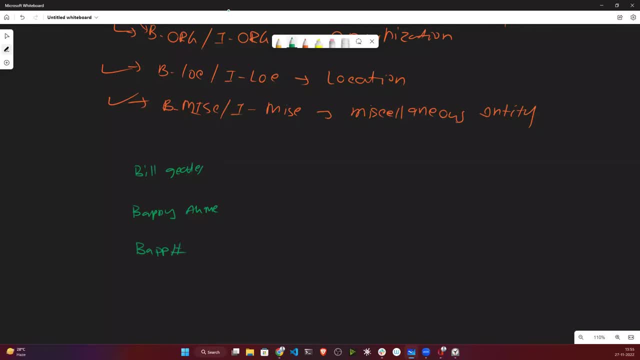 okay, like why was remaining? it will give probably ganne, so we will use how it will Sicherheit. what is the river right now ends, it will assign hash again. it will do hash, hash, hash, y then ahmed. okay, that's how actually it will like break down as a sub word. okay, just one word. you can see it has converted to two, two words. 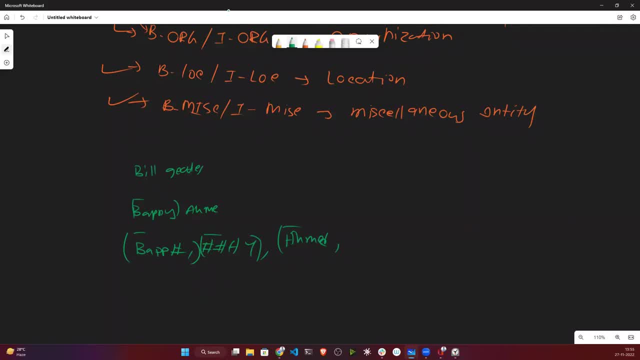 now, okay, by assigning some of the hashtags- that's actually- it can perform some sour tokenization because it is already trained. okay, so you don't have to worry about. it will automatically understand. okay. so that that means whenever you are initializing this one, that means it is all. 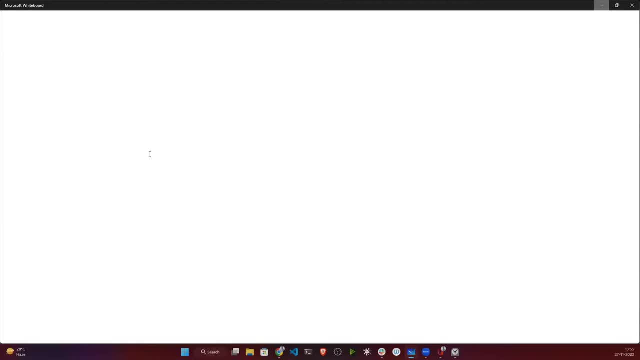 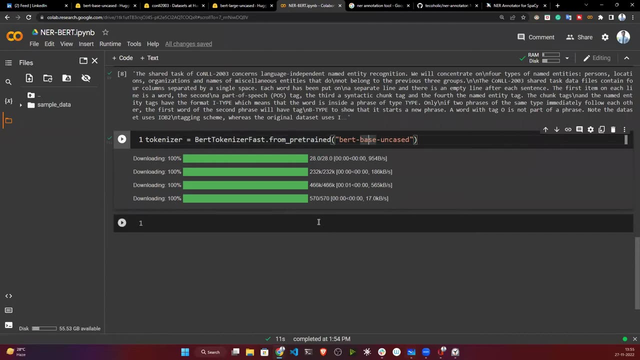 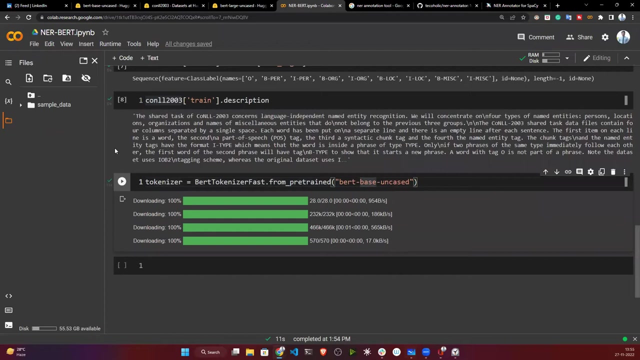 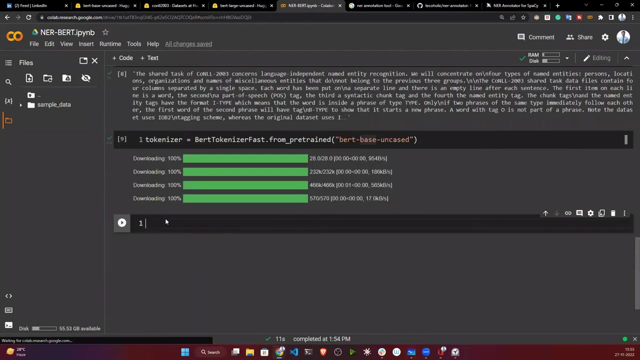 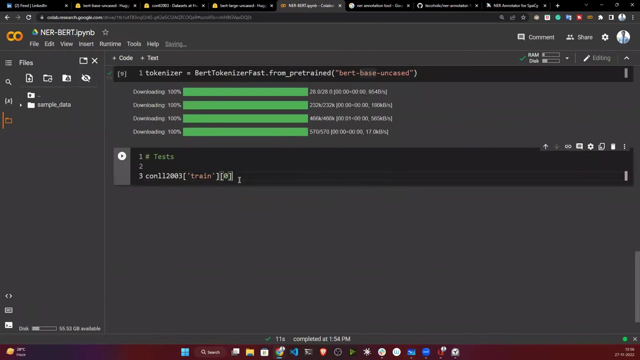 it might also apply the forward tokenizer if it is not able to understand. the text is all about okay. so now let's like apply one testing. okay, here, let's test how tokenizer is working. let's test just one rows and test. so i will pick up one rows, okay, from my model, so from my data set. so this is the first rows. 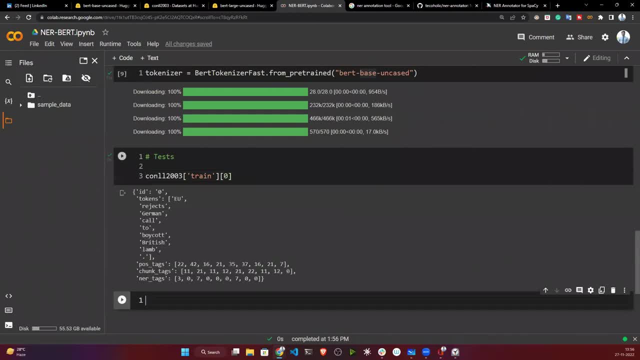 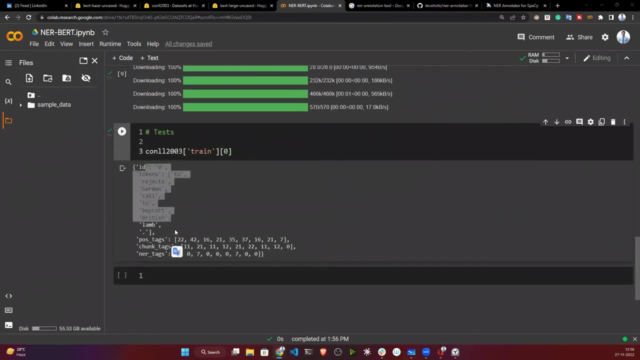 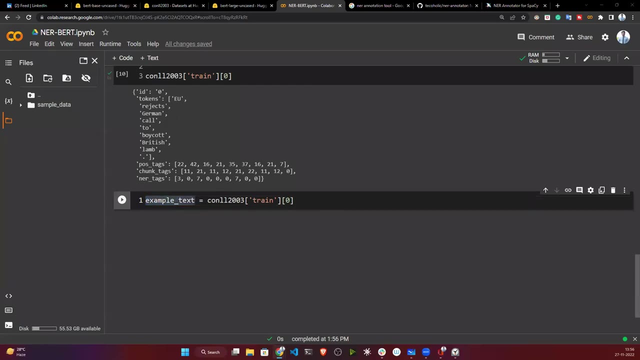 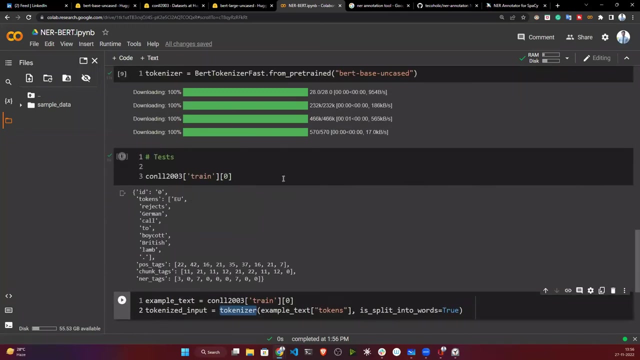 i am taking. okay, now, how to apply tokenize. let's do it. first of all, i'm storing this data in one variable called example text. now you need to call your tokenizer. so this is the code. so what i'm doing, i'm initializing my tokenizer here. okay, i'm calling my tokenizer inside tokenizer, i'm passing my example data, which is nothing but. 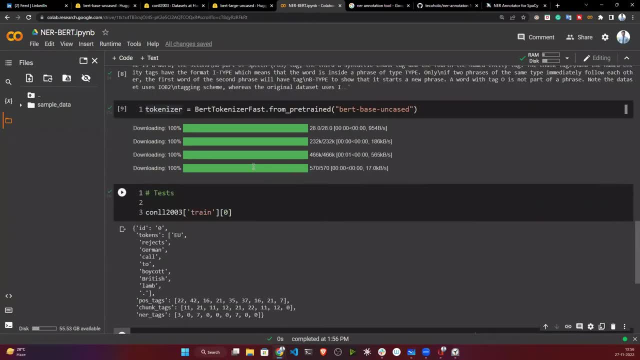 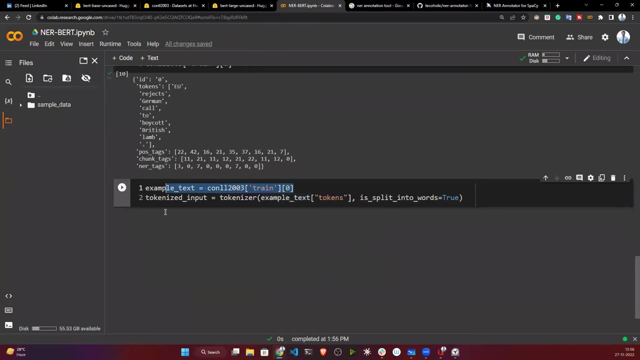 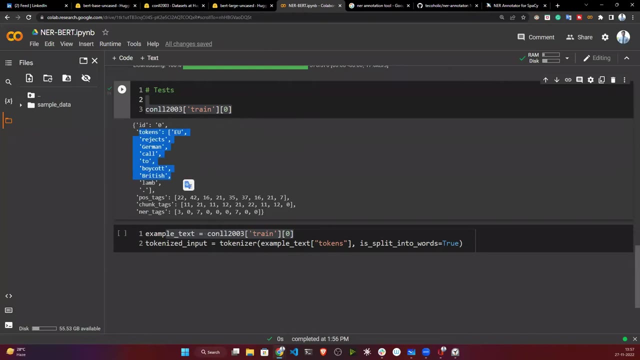 this one. okay, from the example data, what you have first of all, see here i have printed my example data here you have id tokenizer, p, o, stack chunks in here, but which, like which keys actually want to apply the tokenization here? guys, just tell me which is your text like raw text here? okay, it is tokens, right, guys? 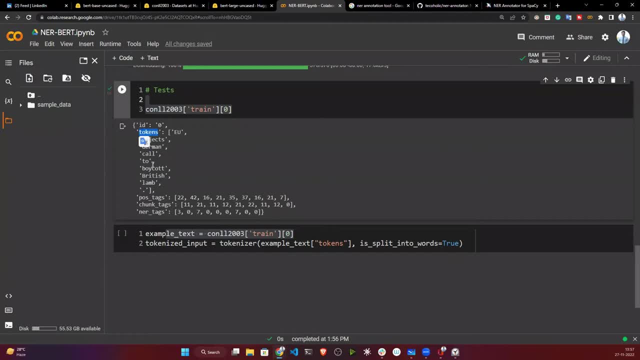 i'm not supposed to text other other things. okay, so that is why i'm calling tokens, okay, key from my example text. because example text is a lot of your tokenized text, so i'm just gonna let you take this, so i will call the other things one by one. i will call my tokenized one here. this is my example text. okay, so this is your tokenized one. so that is why i'm calling tokens: okay, key from my example text. because example text is called tokens. 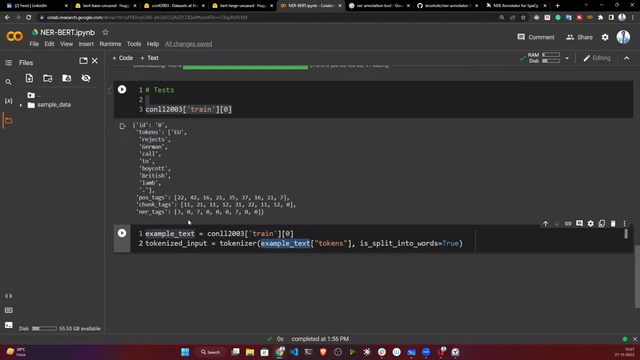 will contain all the information of my data, but i only want to apply on my tokens. that is why i'm calling tokens here, and there is one parameter. you need to make it as true, which is nothing but e split into words: okay, true. now, after that one, what you need to do? you need to call this one. 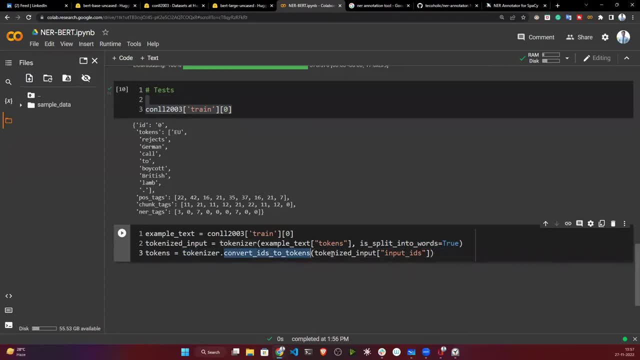 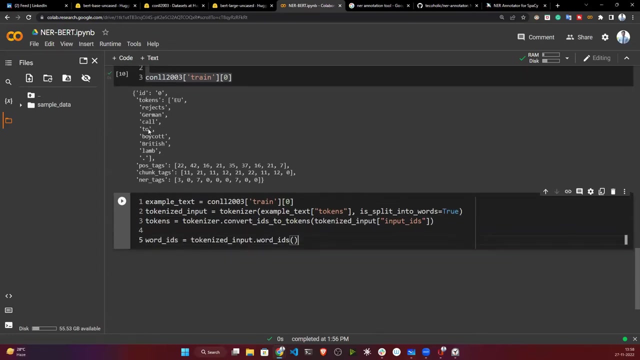 so tokenizer, convert um ids to tokens- okay, and you need to pass: tokenize input and input ids- okay. so these are like some common steps, like you need to perform everywhere every time. okay, now again, you can call this one okay word index if you want to see like each and every words will. 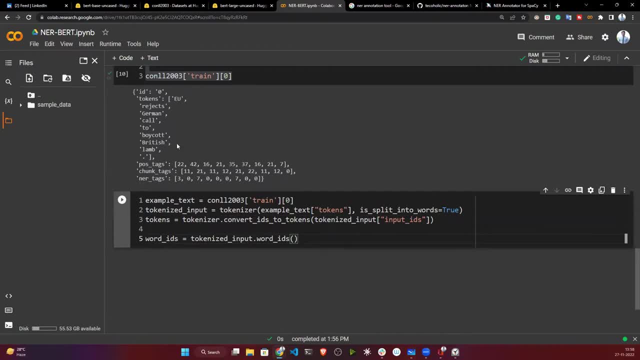 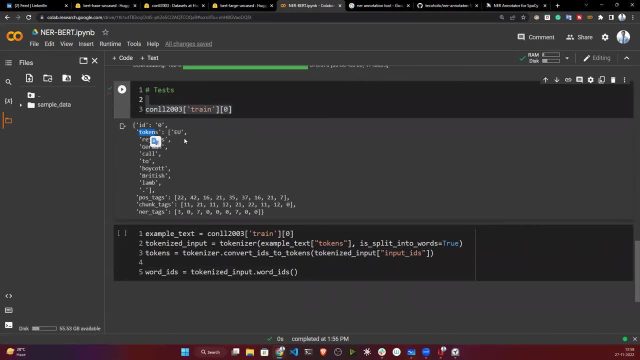 be attaining one unique id, right, guys? i already told you, suppose, whenever you are applying tokenization, first of all, what will happen: each and every words will assign one unique id. then that id will be the result of tokenization, right? so talk about that first. we will talk about tokenization. 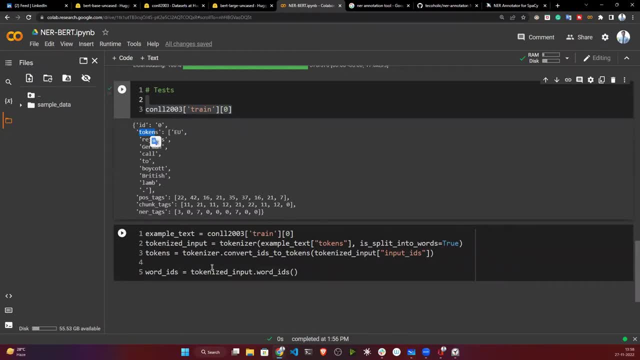 and we will talk about tokenization now. so let's talk about some common steps that we need to will be passed to your tokenization, then it will be assigning some of the tokens. okay, let me print it, then i think you will be able to get it what i'm trying to say. let's print the word id. 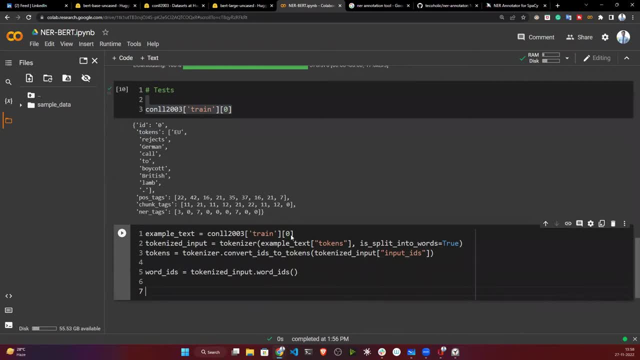 okay, so see, this is your word id. so what? it is nothing. but your? u has been represented as zero. rejects has been represented as one. okay, german has been represented as two. that's how each and every words has been represented with unique, unique id, and you can see none here. okay, what? 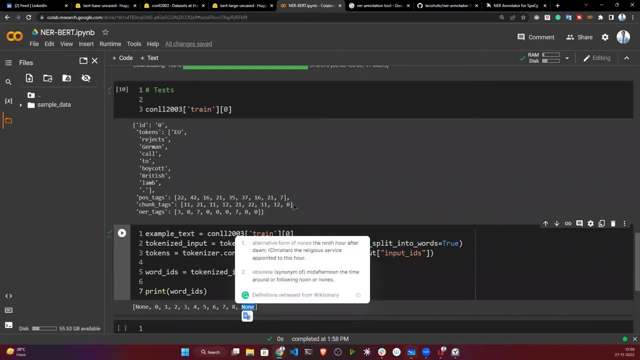 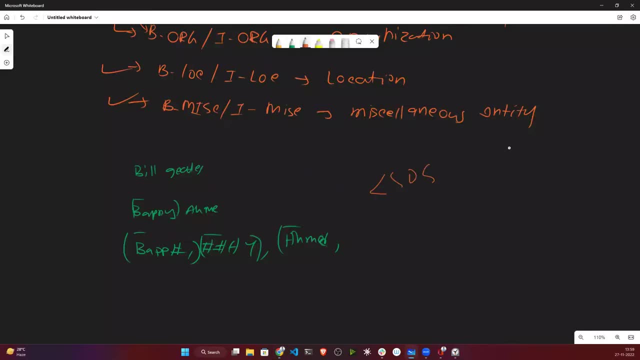 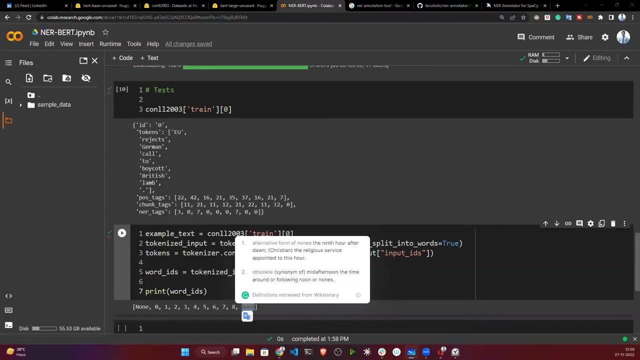 does it mean of none? can anybody remember the concept of sos and eos, eos. anybody remember? i start out the sentence and end of the sentence? okay, so you can talk about, but in what model? actually, we can't define as, uh, you can say sos and eos. okay, what we define. 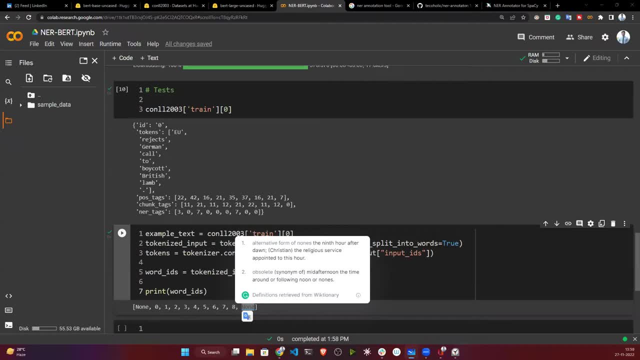 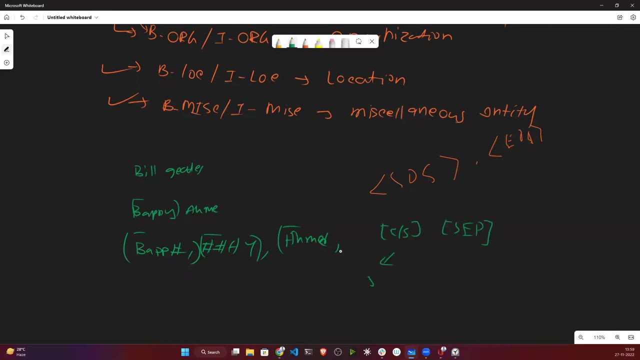 in, but actually it is represented as nothing but cls and acp. these two. that means uh, cls, that means this is your start of the sentence, and acp means your separator. that means end on the sentence. okay, okay, so you do not know that hasode. okay, guys got it. what is? 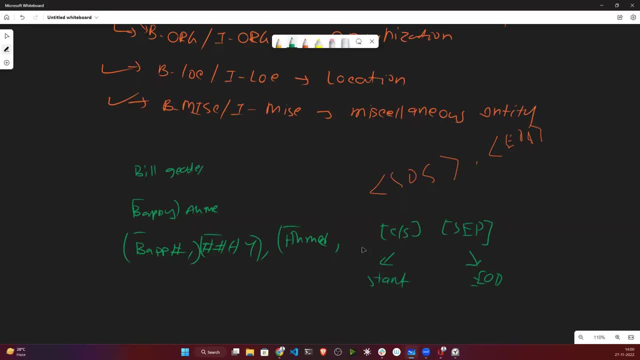 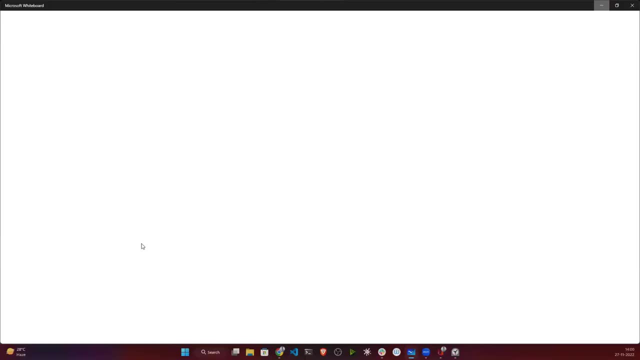 Lок hear ان marginal and what is acp? okay, so that is why here, why it is providing none, because it hasn't defined any, anything here. okay, that's why initially it would be none. that means this is your start of the sentence. this is the end of the sentence. that is, this is your cls and this is your acp. 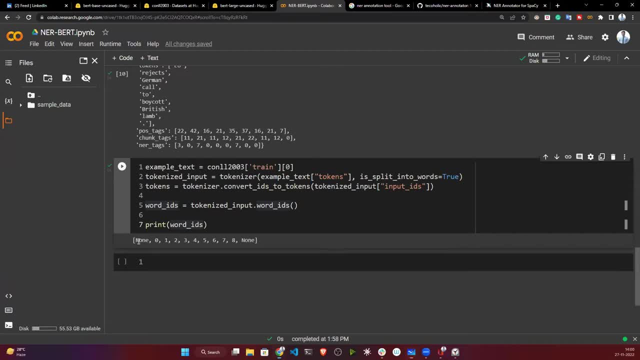 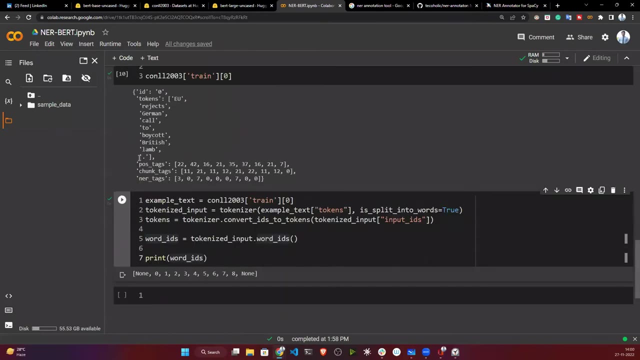 correct, okay, so this is the end. okay, and inside that you have your all the words. if you see, just count, there are nine words: one, two, three, four, five, six, seven, eight, nine, zero, zero, two, eight, that means nine, okay, if you just count from here. also: one, two, three, four, five, six, seven, eight, nine, that is full. stop is also there, so it. 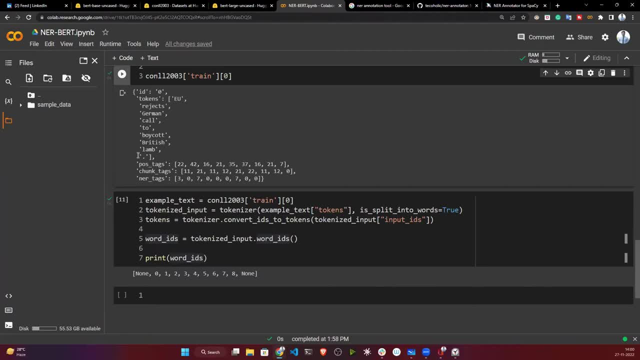 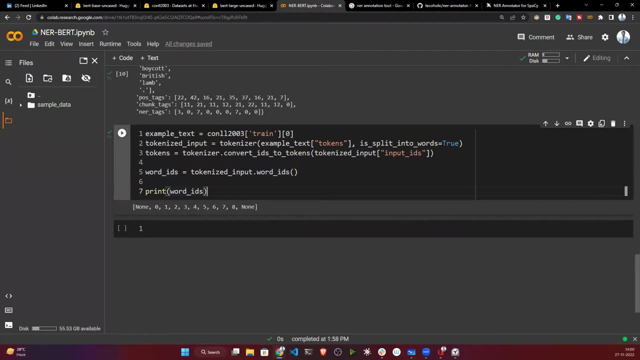 is also counting as word. okay, that's actually in the back end. actually, your tokenizer tokenizer is working. okay. now, if you want to see tokenize output, okay, tokenize output. what is the tokenize? like input, like it has given the final tokenization. you can see it, just call, call this one. 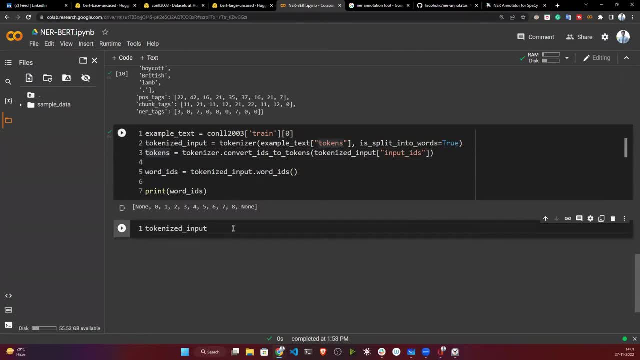 tokenizing input. okay now, if i execute now, this is your final tokenization. okay, so how you did the tokenization? now? if you see nine words: one, two, three, four, five, six, seven, eight, nine zero. two, three, four, five, six, seven, one- none has been represented as one zero one. that means this is your cls. okay, and similar wise. 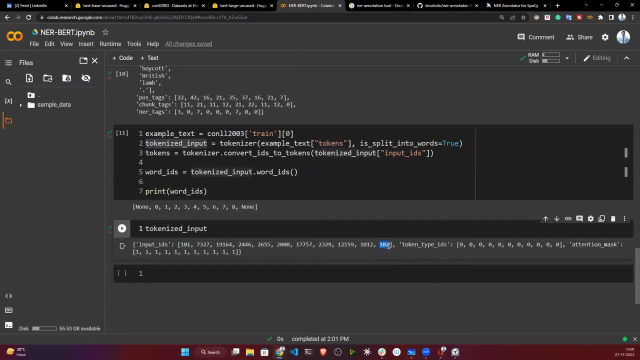 if you see your sap, sap has represented as one zero two. so whenever you are passing this model, passing this data to your model, your model automatically will get to know one zero one means it is representing cls and one zero two means it is representing as sap. okay, and inside you. 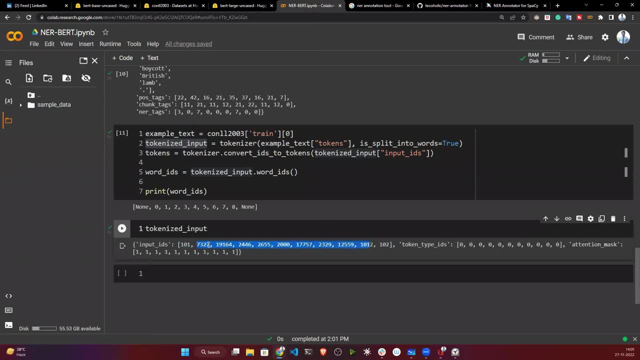 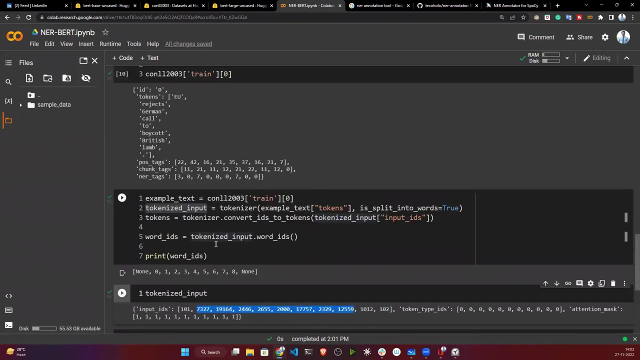 have nine words token. you can see, okay, like seven, three, two, seven, uh, then uh, one, nine, one, six, four, okay, so these are actually your encoding. okay, these are actually your vector. that means this text is represented by this number. how they are doing, because bart has their big dictionary, okay, dictionary, they are mapping the. 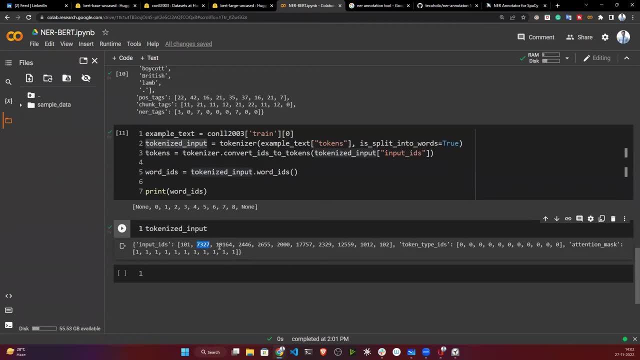 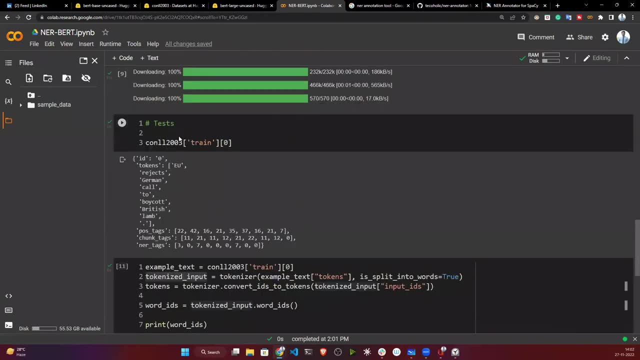 word, so in the. but if you see it is already huge data. they have, like already trained inside that actually this rejects is already already there. there's already a lot of data already in there. so german is already there, call is already there and it has some mapping number. so that number, 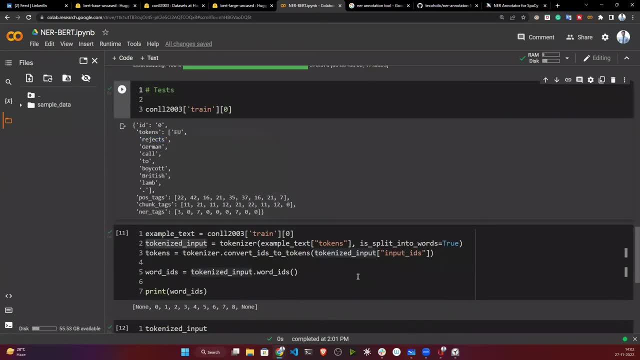 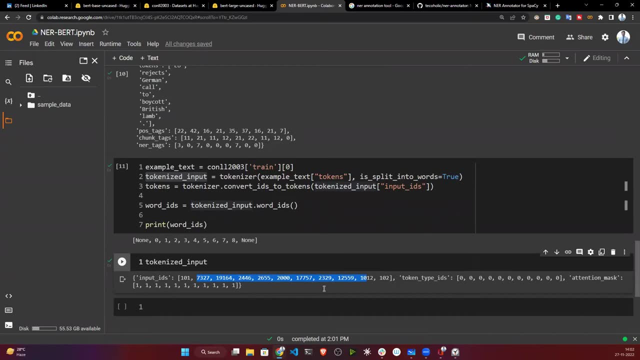 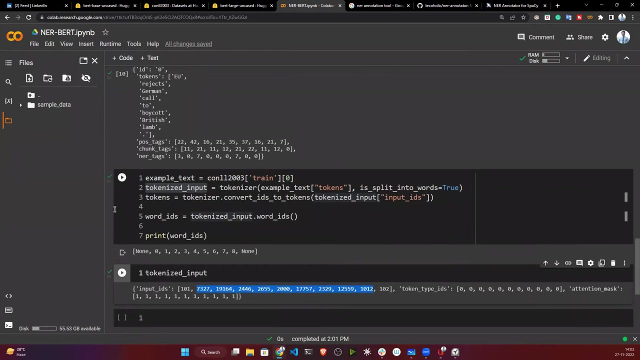 actually it is giving. got it, guys, how it is doing the tokenization clear or like not clear, so you can talk about: this is your encoding, this is your word embedding you are doing. okay, not anything else. okay, so this word embedding you are doing using the butt, pretend butt model. okay, got it. 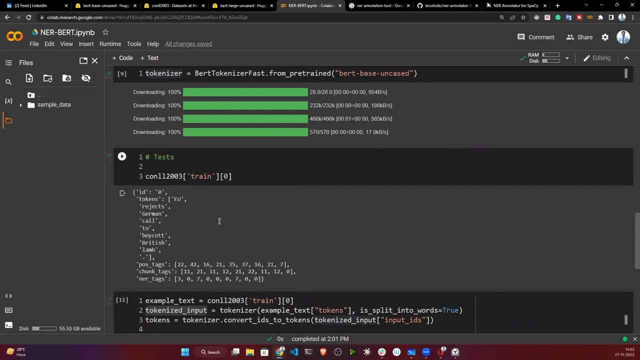 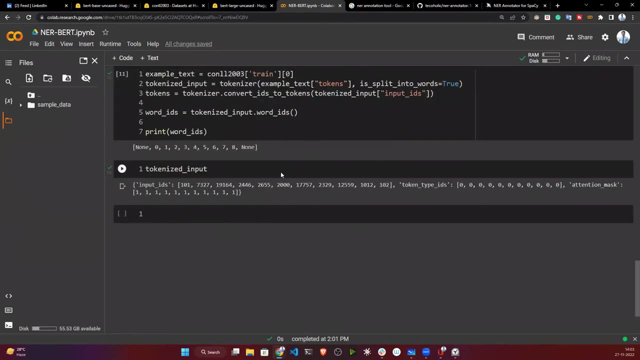 but i showed you example using tf, idf- what to wake that thing. you can perform whenever you are using using machine learning model or any any other model, but whenever you are using transformer, you need to use transformer based word embedding. just write yes or no. is it clear? 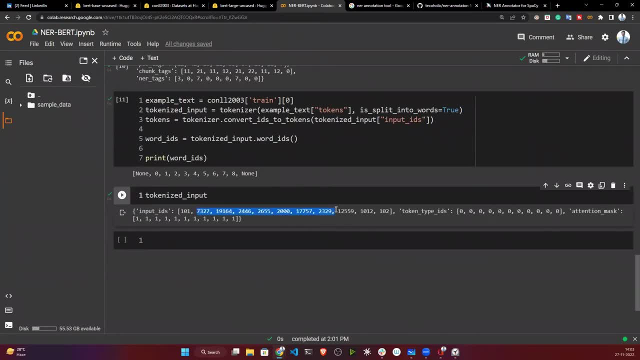 okay, and this two number is your sap. sorry, cls and sap. that means end of the sentence and start off the sentence. okay, it is representing by that, but with respect to that, if you see there are some additional information, it is also given, like token, type ids and attention mask. i think just. 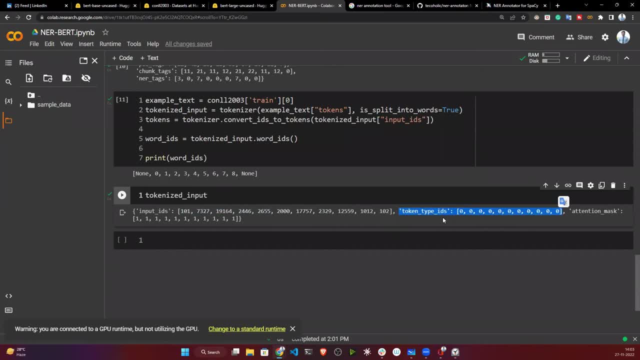 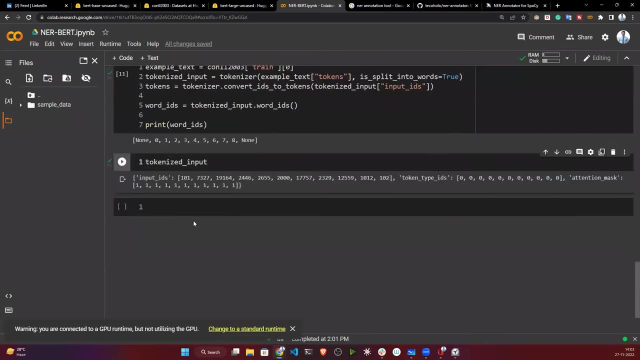 sometimes, before you have learned of about attention mask, you can see that it is also given like token, type ids and attention mask. what is the concept of attention mask, guys? it will provide some of the attention on some of the words, right, guys, suppose. if i give this example, bill gates is the founder of microsoft. 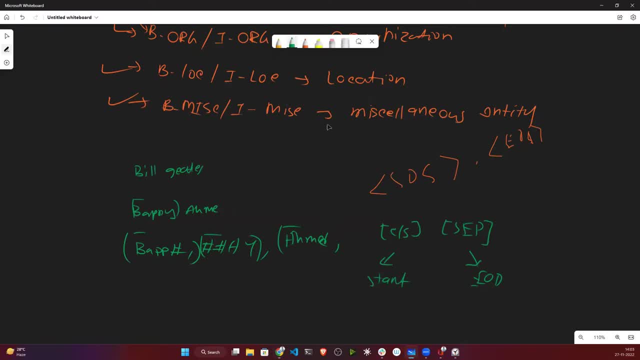 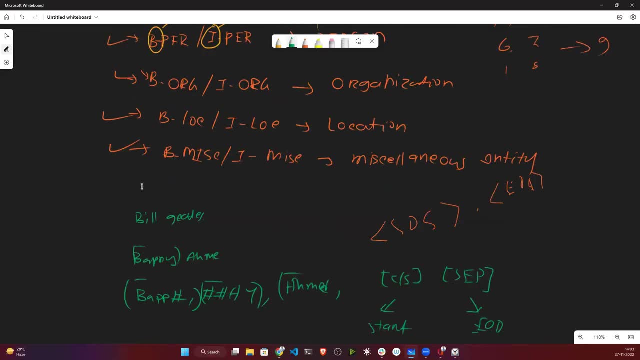 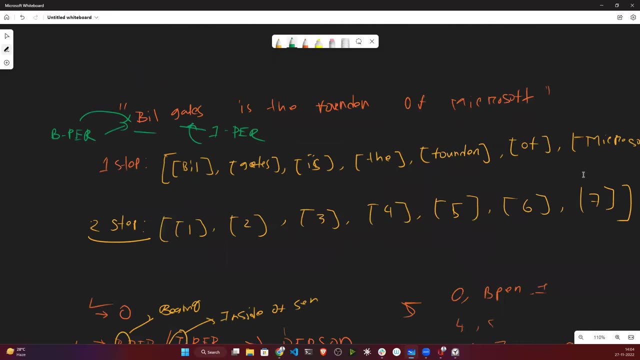 so whenever you are giving this one, so in the backend it will assign some of the attention with some of the words. okay, so this is your attention mask. actually it is providing, but first of all it is providing one, one, one, one like that. okay, it is like optional. you can provide the attention mask. either you can remove the. 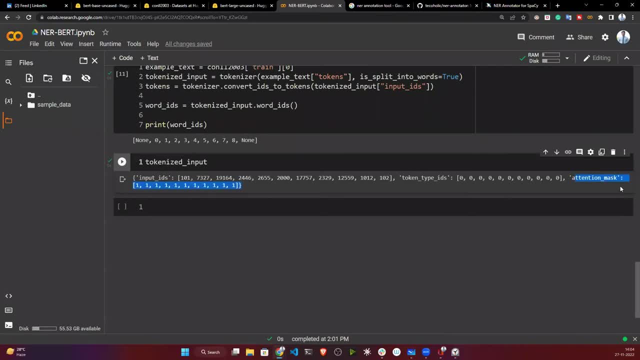 attention mask. okay, it's up to you, but most of majority of the time i saw like they're using attention mask also. okay, so these are like this: is this is your like, important, important things, and these two, actually your butt model takes actually as a, as an input. 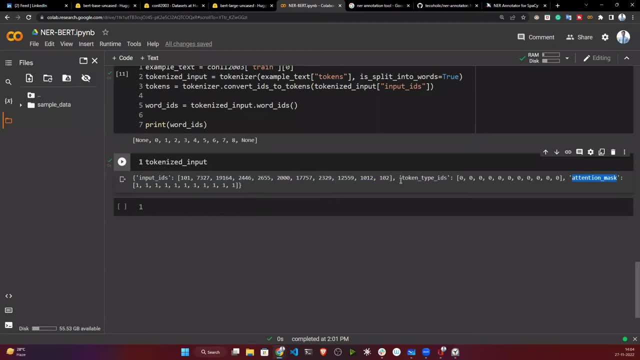 you need to provide dollars, you don't have to worry about it, will automatically generate it whenever you are doing the tokenization. okay, now if you want to see, like how it did the tokenized- actually actual word tokenized- now you can see. just copy this code: okay, and paste it here like tokenizer: convert ids to tokens. 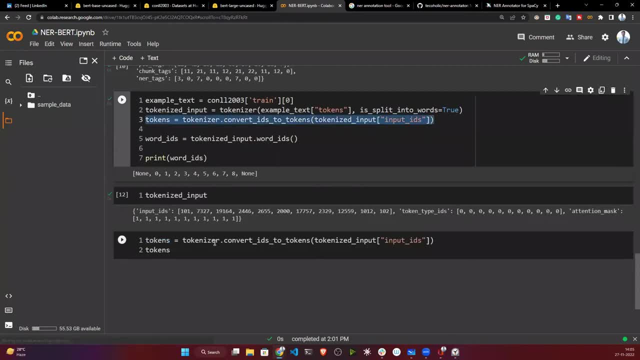 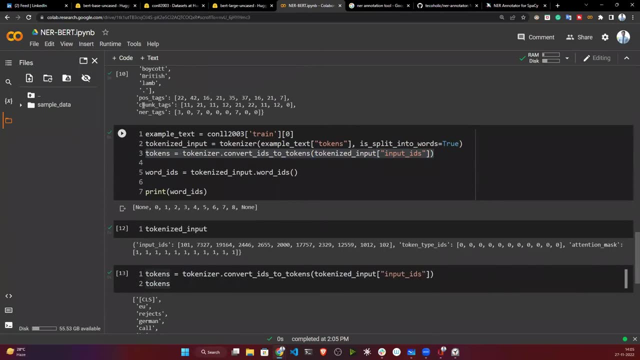 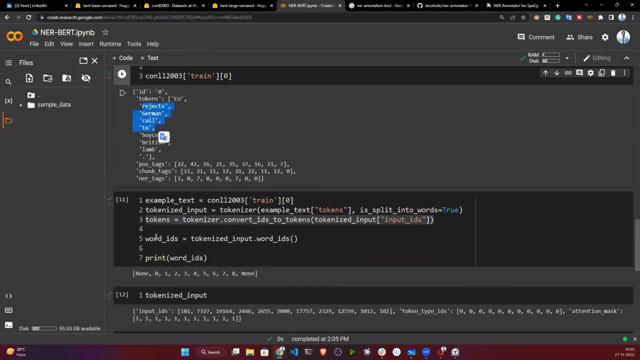 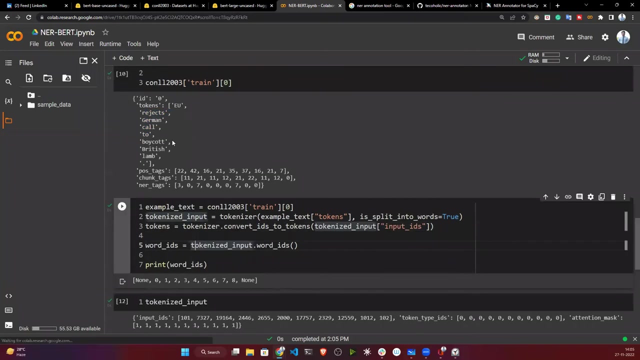 and just provide your token type inputs. and now, if i print it now, you can see this was my all my words. see first of all what is happening whenever you are providing the words. first of all, it will do integer encoding entities are encoding nothing, but it will assign some of the 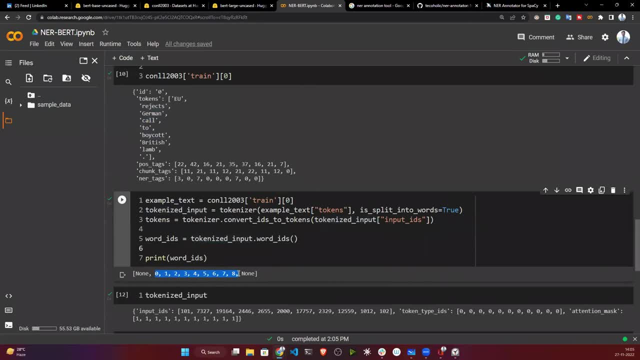 id: unique id: 0, 1, 2, 3, 4, 5, 6, 7, 8. i think i showed you this example whenever i was doing lstm, example, how to do integer encoding. umesh, did you join the session? those who attended that session. actually, it would be very clear in their mind. 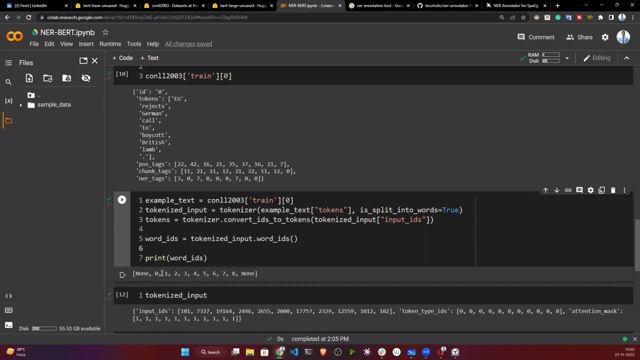 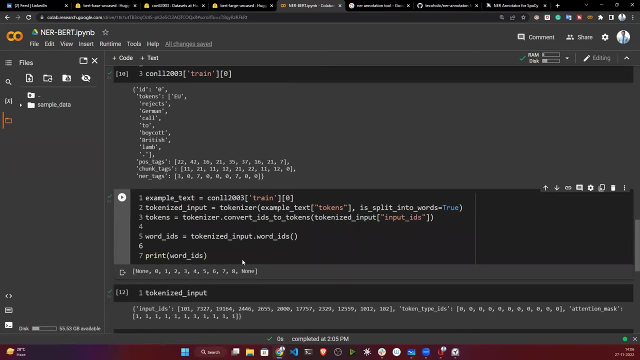 guys, just tell me yes or no. first of all, you are applying integer encoding, okay, and whenever you are in assigning integer encoding, by default your cls and sap would be none. okay, you are not assigning anything. but whenever you are applying actual tokenization, at that time it will convert to 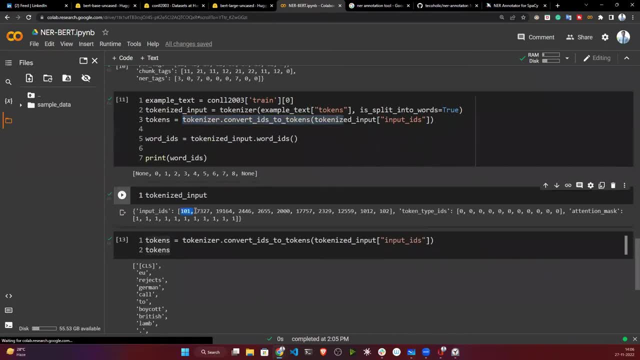 one zero one and one zero two. one zero one means cls and 102 means sap. okay, and inside that you are applying your put tokenizer. that means, but what embedding you are applying? okay, just remember, whenever you are assigning integer encoding, at that time it would be none, and whenever you are applying actual tokenizer, you are converting to the word name. at that time it will, none would be represented, and like your because, see, for example, oxygen and bad embeddoing would beito. the bad will be represented as and like your. because, see, for example, if you are applying an internal tokenizer, you produce some data on a0 to Madrid stir crunch. SAP will not be connected to the model when really the tokenizer is 266 isconverted to the word embedding. at the time it will, none will be represented, and like your. 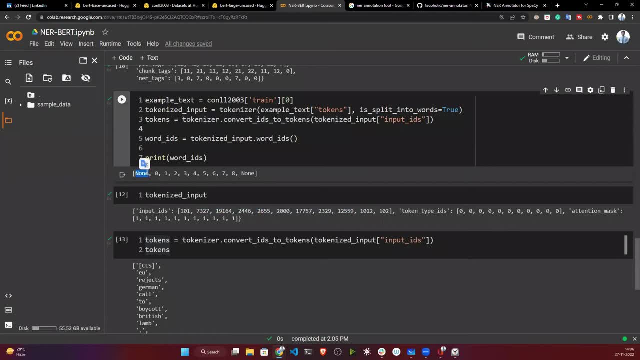 none is what. first one is your cls, okay, and the last one is what? last one is your sap, okay. so that means cls, you are defining 101, sap, you are defining 102. this number, actually, your bat model already knows. if i am able to see 101, that means it is the start of the sentence. 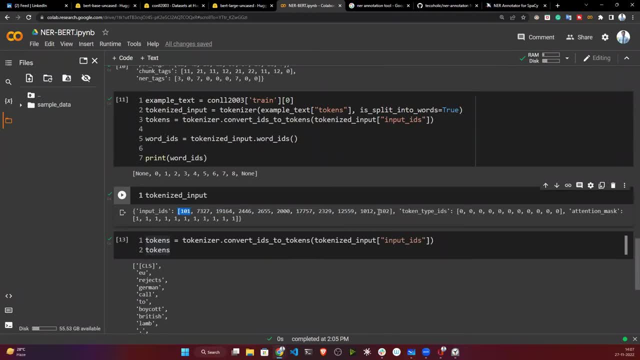 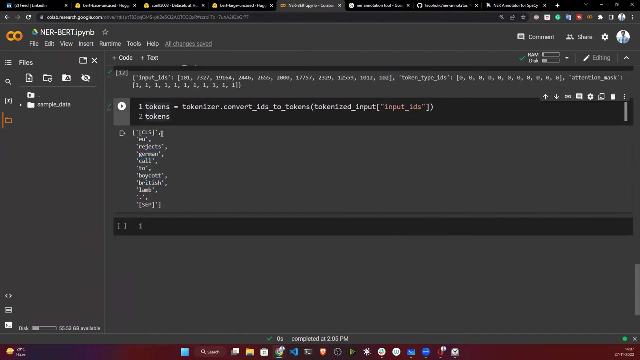 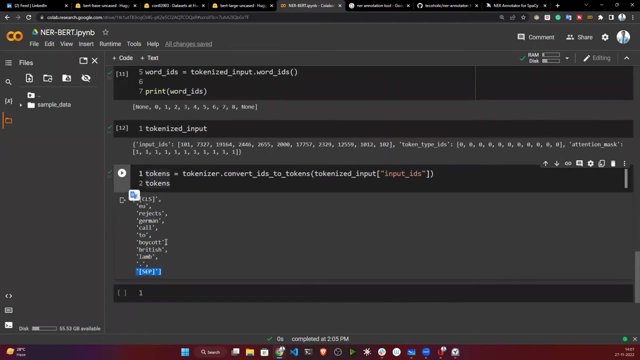 and, if i able to see like 102, it is the end of the sentence. so got it guys. now if you see, yeah, this is this is your actual text and see it is applied- cls and sap at the last, this is just converted to your 101 and 102. okay, if you want to see as a high level overview, okay, 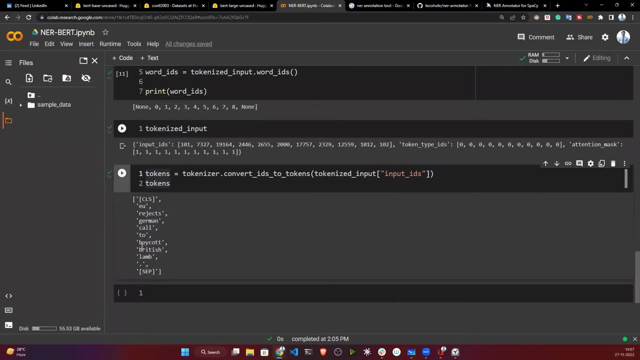 you can see here now there is one problem. can anybody tell me what is the problem? so let me show you the problem first of all, if i uh, yeah, call this one and let's first of all execute. first of all, this is my input data, guys. any confusion here. this is your input data, right? 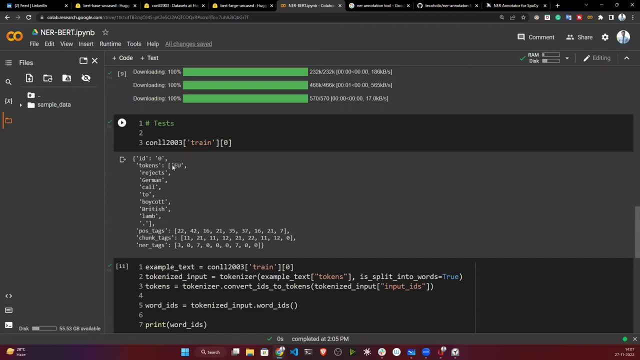 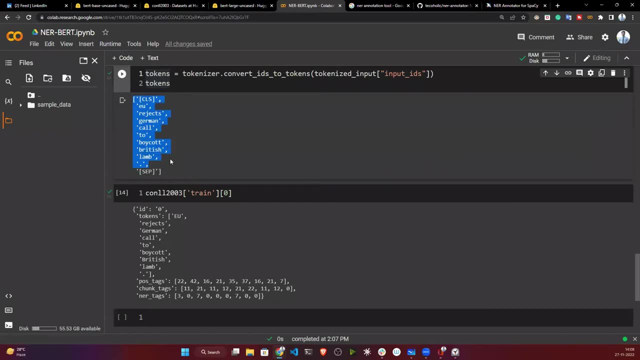 this is your input data. with that, what? what you need to provide as a output? what should be your level here? okay, just see here what should be your level here. from this data, write something. what? what would be your level? any attacks, right? i'm not considering anything. 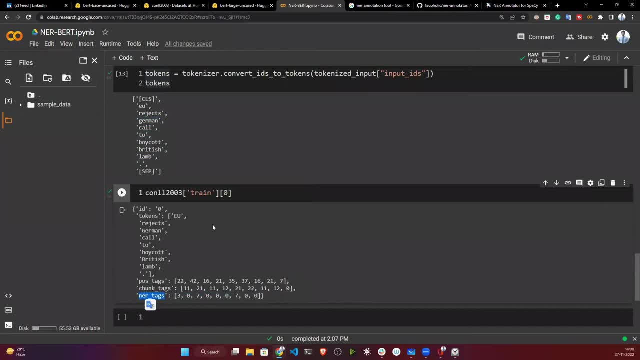 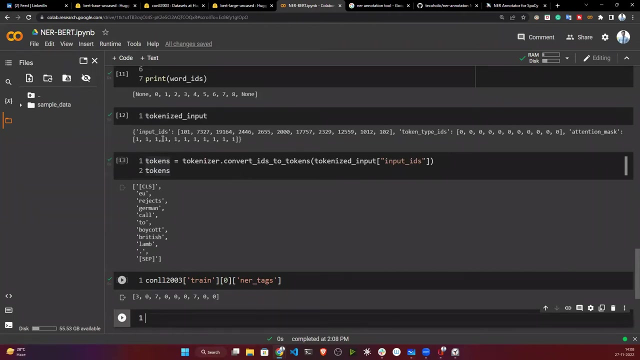 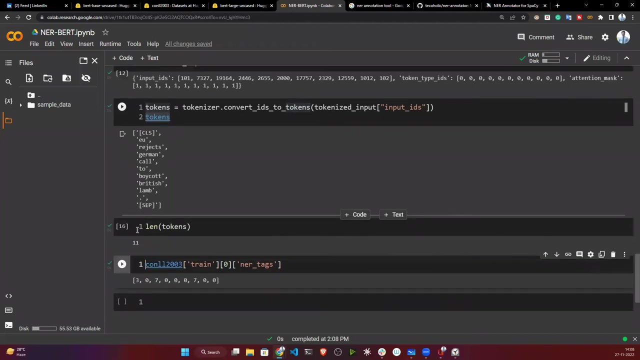 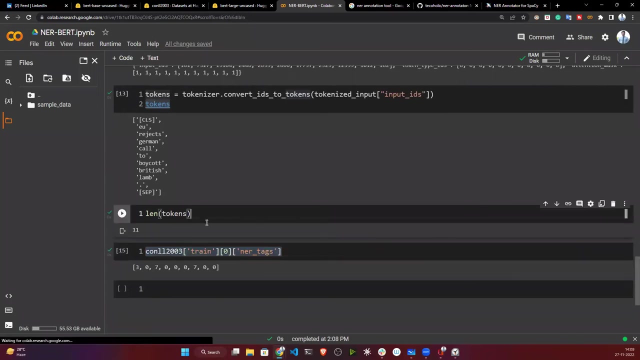 i'm just only considering any attacks. let's call any attacks. this is your linear tags now count. okay, let's see your length of the token. first of all. what is the length of the token? it is 11. now let's count off your level. what is the count? it's 9.. now can i give this input to my model or not? 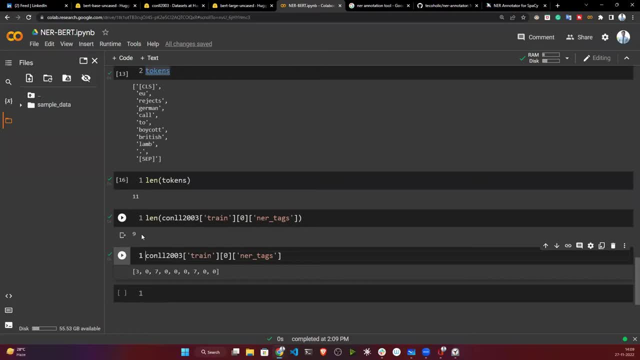 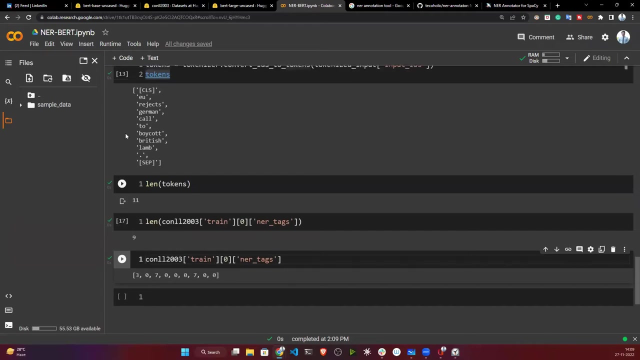 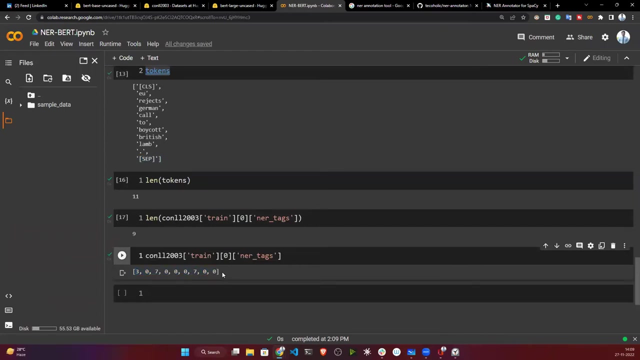 anybody tell me if you are doing token wise classification. is it possible, because dimension is different? okay, yes, start. see, it is not counting cls and sap. okay, it is not counting cls and sap. okay, in your level there is no cls and sap. it is assigned, so i need to write our own like custom. 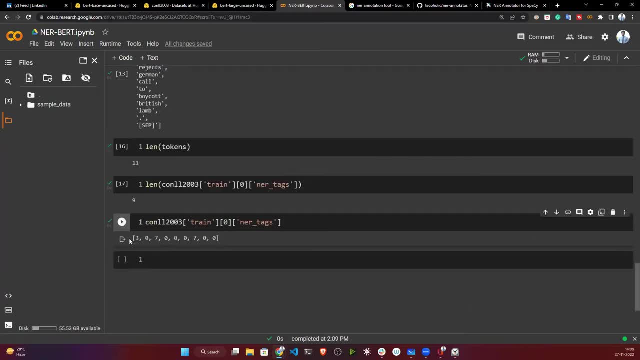 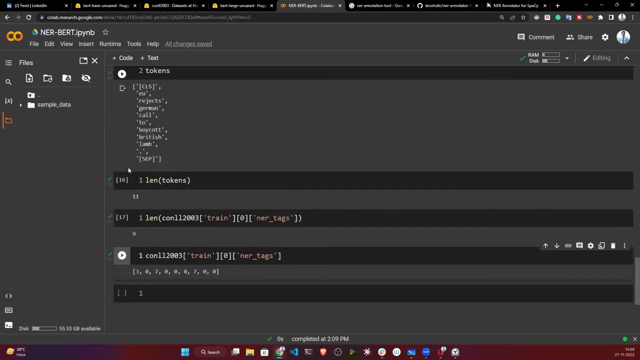 function okay. so what it will do, it will assign something at the first and at the last. okay, but here cls and sap is not important for my prediction, okay, so what i will do, i will assign minus hundred, okay, of the first and of the last. okay, why am i asking minus hundred? 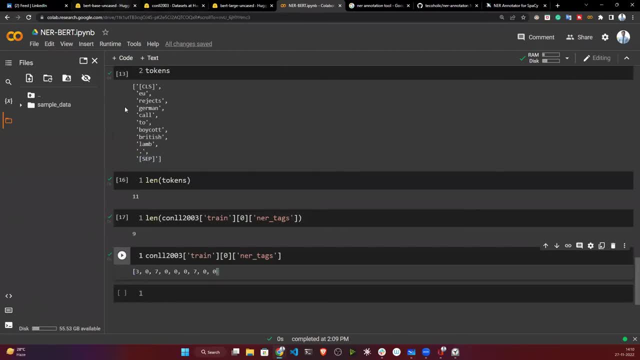 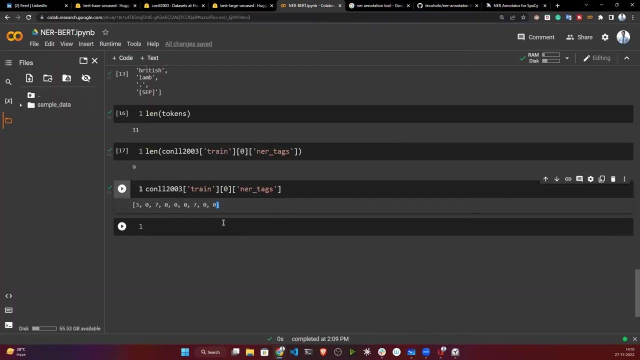 because, if you see, this is the pytor's implementation. okay, the code i'm using here, this uh transformer based in here back end, it is running pytorch. okay, so pytorch actually by default during training. ignore minus 100 numbers. okay, because i'm not supposed to train this one. 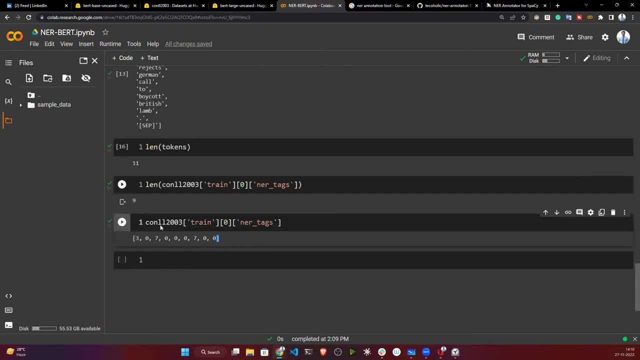 i'm just only considering as a dimension. i need to match my dimension. that is why i need to pass okay. so at the first of the this list, you need to assign minus 100 and at the last of the list, you need to define minus 100. so now your dimension. 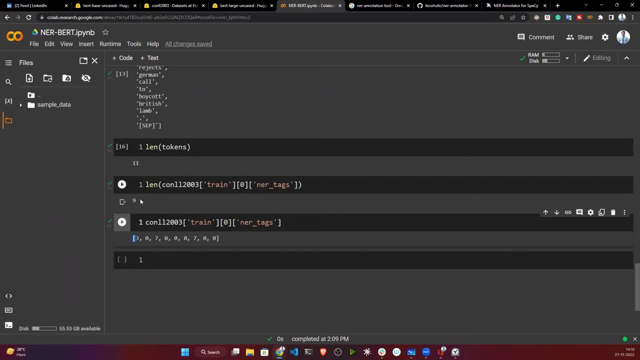 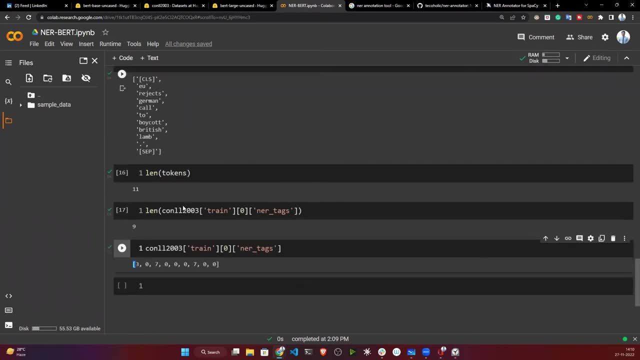 would be 11 guys. okay, but during training you don't consider the minus 100, because it will ignore, because i'm ignoring my cls and sap. i only want to know it is the start of the sentence and end of the sentence. but i'm not supposed to train it, okay, i only supposed to train. these are the 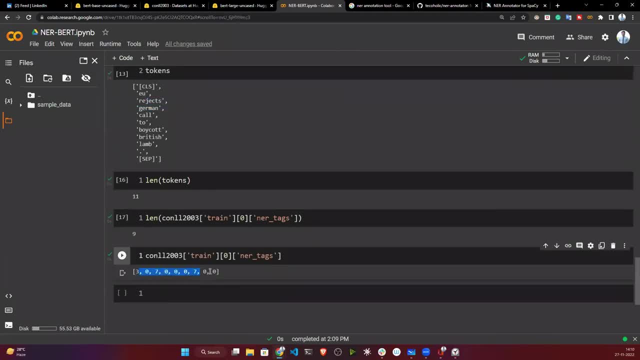 word with respect to these are the labels. this is my requirement. okay, i think it makes sense, guys. only just for the dimension mapping, i will be adding two things. one is 100 minus 100 at the first, minus 100 at the last. okay, if you just map this two list together at the first, if you have. 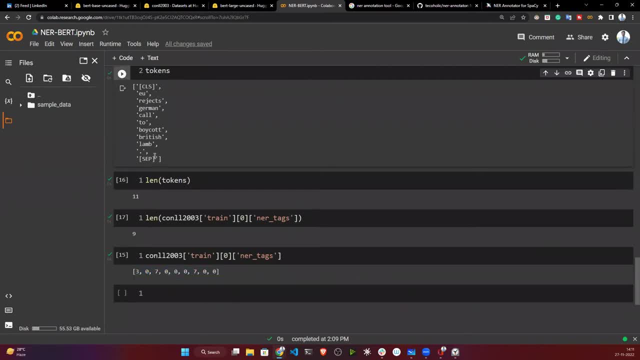 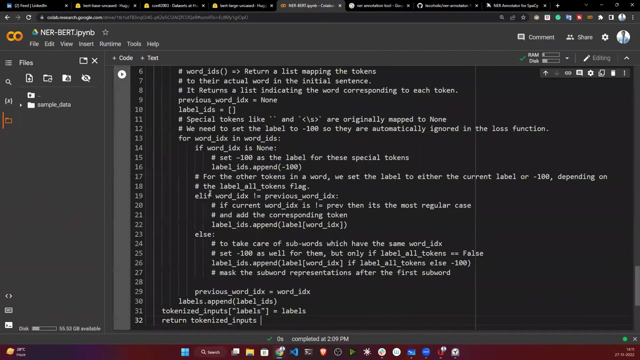 cls: i will add minus 100 as cls sap: i will add minus 100 sap. that's it. okay, so the function i am defining right now. so this is the function it is only responsible for doing, like that. okay, this is the function. this is just a simple python code. i am reading my ner. 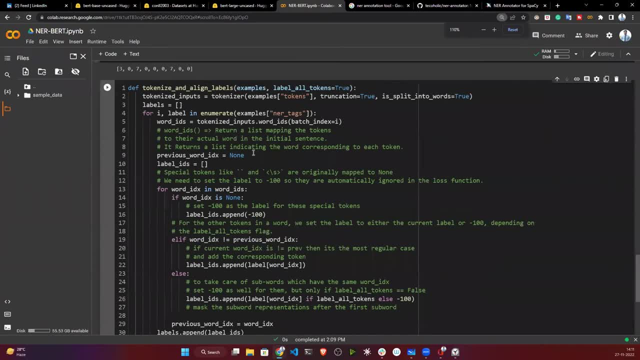 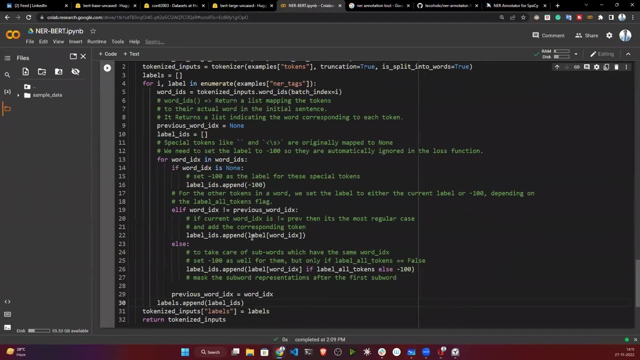 i am counting the words, okay, and at the last, if you see i am adding minus 100. okay, let me zoom a little bit. yeah, minus hundred and that minus hundred again. i'm like labeling: okay, level, i'm defining as label. i'm not keeping as any attacks, i'm defining as label. let me run and 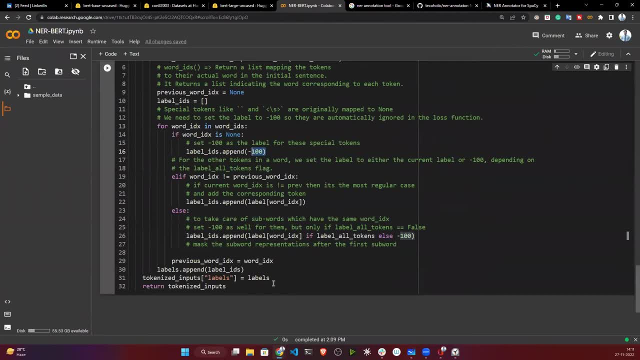 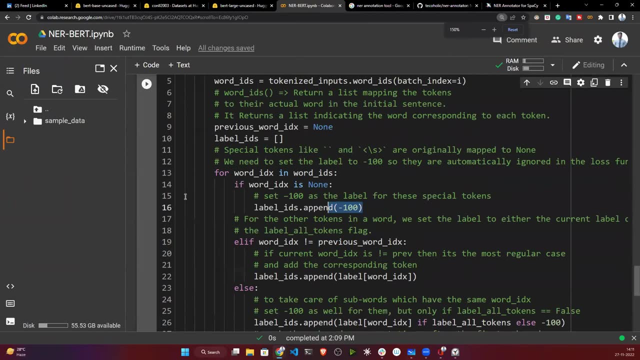 show me one example how it is working. okay, this function is run. so the function name: i kept token nice and align level. okay, so see, as of now i i showed you just one example of tokenization, but in that function i'm doing all of my data. for all of my data, yes, minus 100 will be added to the. 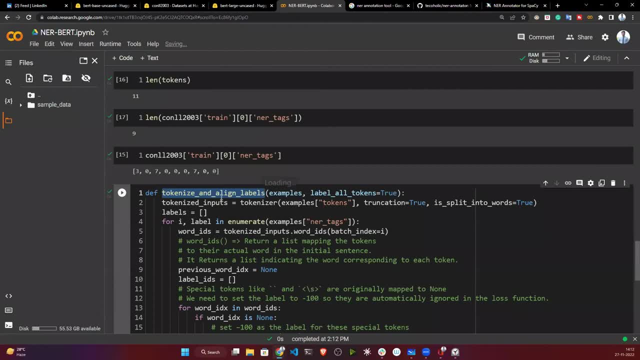 first and the last of the sentence, something okay. so i'm going to add minus 100 to the first and the last of the sentence. so i'm going to add minus 100 to the first and the last of the sentence. okay, and this is your final function. it will do the encoding first of all. that means tokenization. 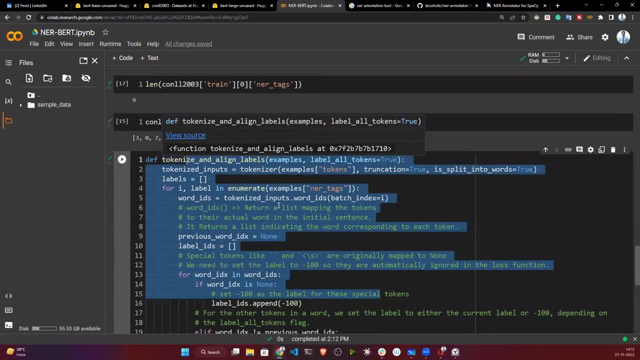 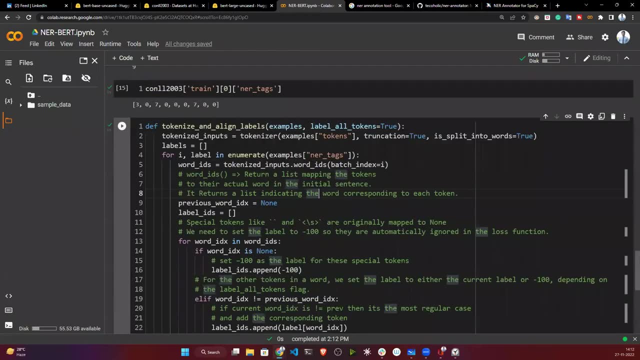 after tokenization, it will add minus 100 at the first and the last, okay, and it will assign one label and it will save as a level. let me show you one example that would be clear in your mind. suppose i'm taking this fourth number of example. okay, i want to apply on this data. 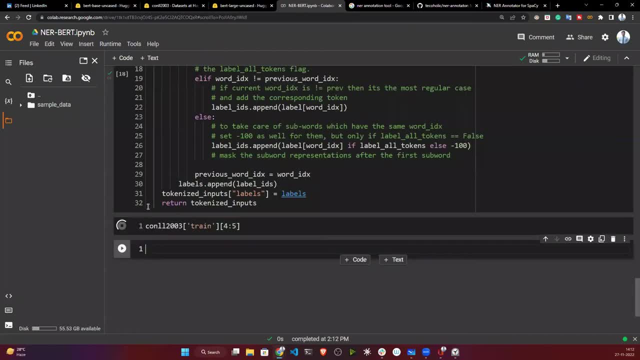 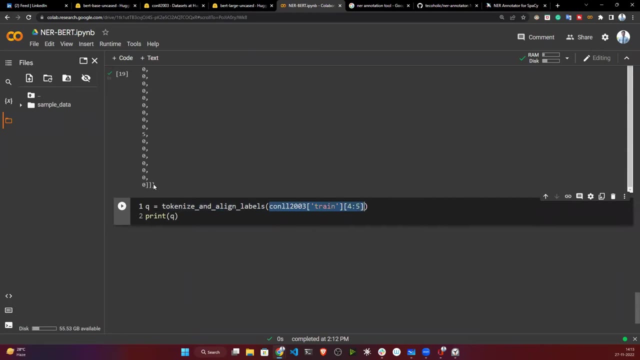 this, this function. okay, now let's see. first of all, see this is this is my raw data. okay, i got. now, if i apply this function, this tokenize align level, and i'm passing this, this rose. okay, that means this, this example i'm passing: okay, now, if i run and if i print the queue, you is your. 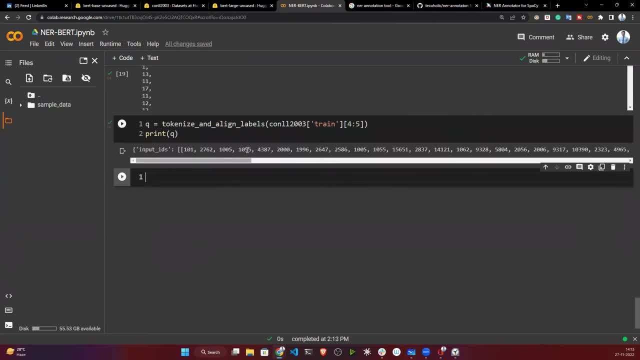 nothing but its output. now, if you see, this is your input ids, it is, it is clear. okay, now what you have here. you have token type ids. it is also clear. i used to got right attention mask. it is also clear. and instead of uh, any attacks, what i named, i left. named is as label. okay, i replace the name. 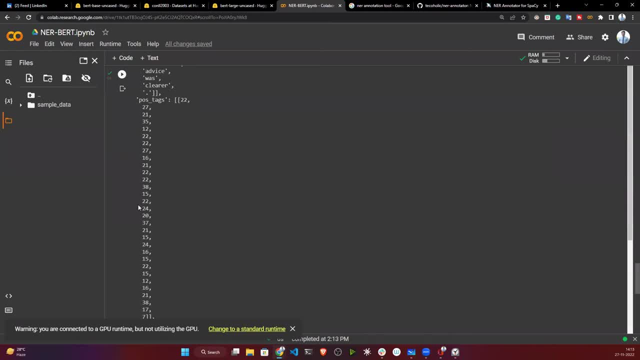 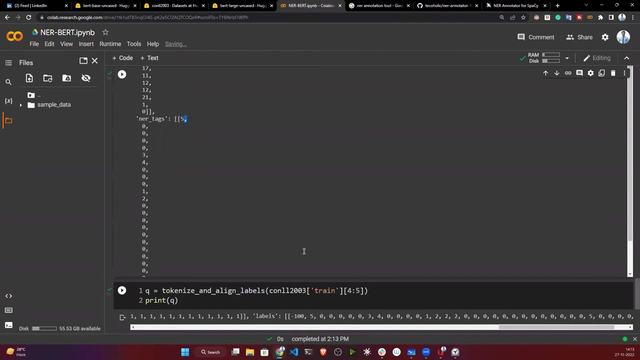 okay, now label. this is my label, this is my raw label. guys, if you see, if i show you any attacks: zero, zero, zero. okay, it is starting from five c: five, zero, zero, zero, zero. but before five it is assigned minus hundred and at the last of the list, if you see, it is also assigned minus hundred. 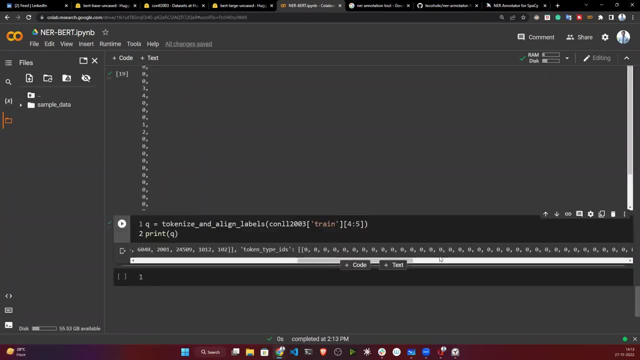 i think it should be clear now how this function is working. now i have my input data, that means my input ids- and i have my output also. that means my levels. now i can pass to my model. clear yes or no? you guys just do response yes, okay. 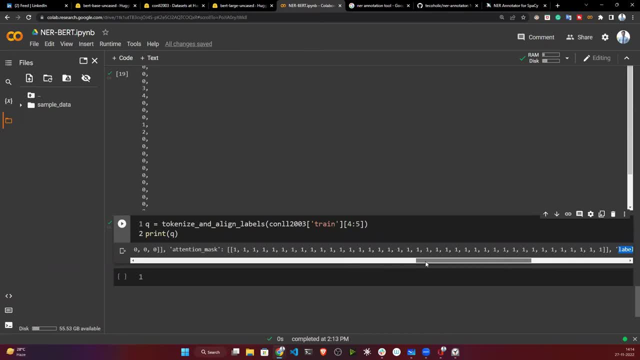 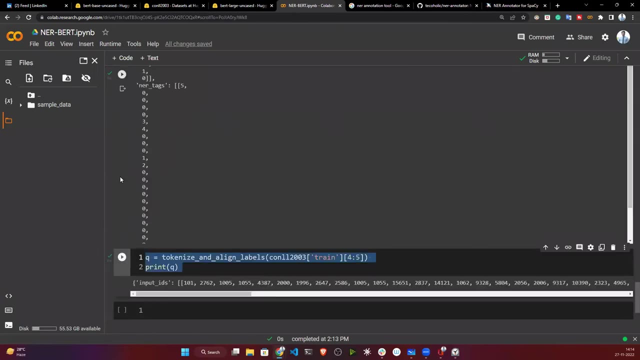 okay, now, this is one example i showed, but what i need to do? i i have my entire data. that means nothing but your uh, this one, uh, con ll 2003. okay, this is your entire data, but i showed you on just one example, just for testing. now let's apply. 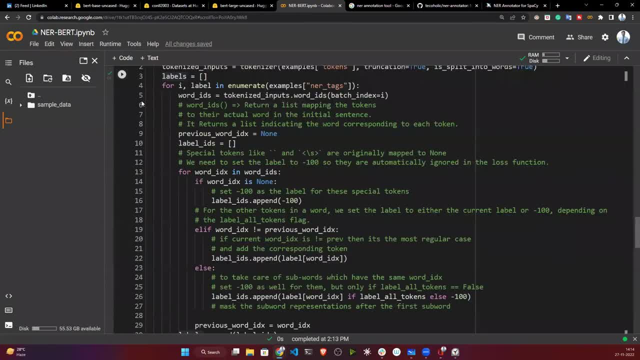 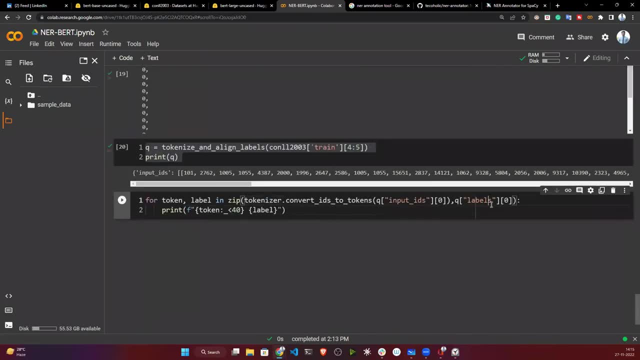 this one. okay, this is your entire data, but i showed you, on just one example, just for testing, on my entire data, okay, but before that, how it is representing. if you want to see, i can also show you. this is the code. so what i am doing, i'm converting and i'm calling my labels, okay, well, this i am. 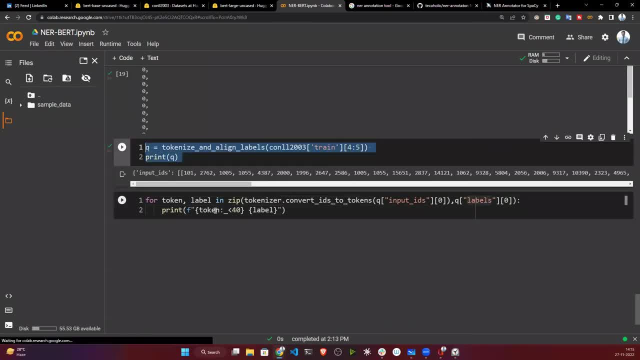 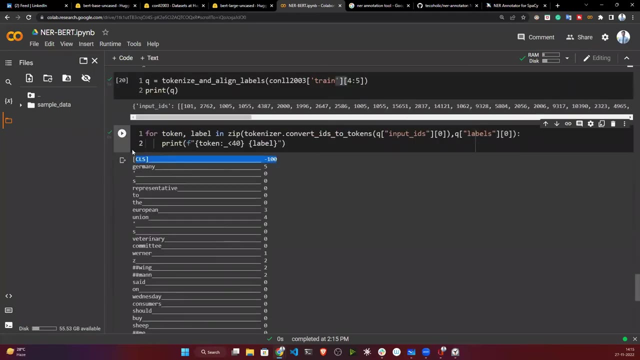 calling my levels and i am: just let me run, i think you will get it. see, now cls is ascending with minus hundred. then germany it is representing as five, because if you see the level was five, any attacks, and if you see germany was the first one inside tokens germany. okay, this representation is fine, but before that i'm it was cls, so it is. 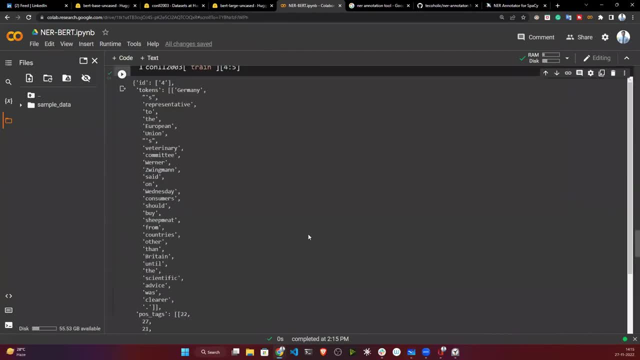 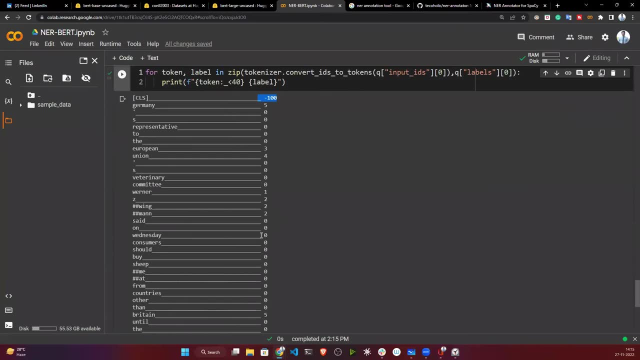 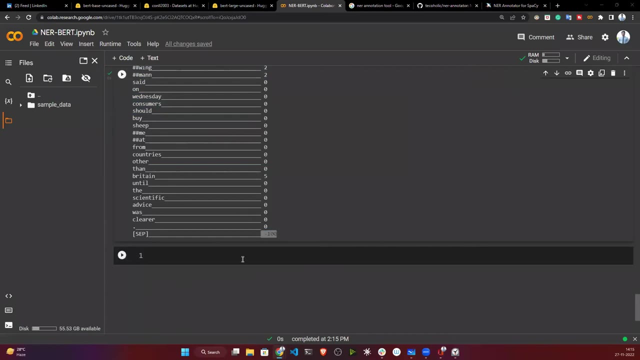 representing as minus hundred and all the words it is representing with their corresponding levels. at the last, if you see, sap is also representing as minus hundred. okay, just for visual understanding. i showed you this one. okay, so now let's apply on top of my entire data. okay, because i just show you one example. so inside this data set, you have one um. 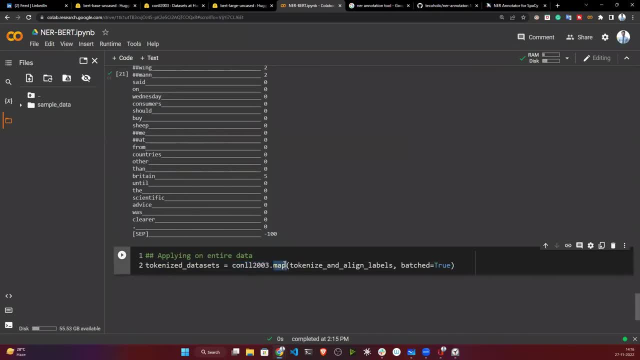 method called map. i think you already familiar with the map in python. okay, so it will actually map up this tokenized align function. okay, in the entire data. okay, and batch is equal to true. i'm defining, now, let's execute. okay, now this is your tokenized data actually, but initially it was. 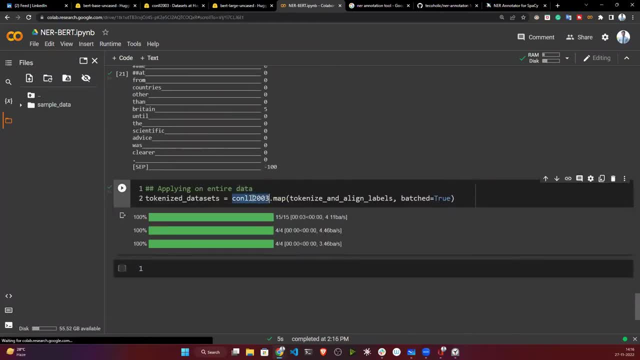 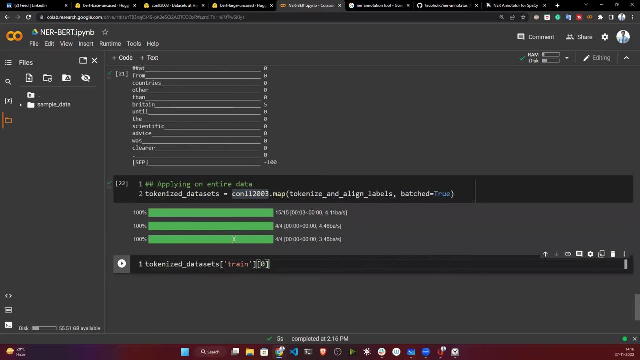 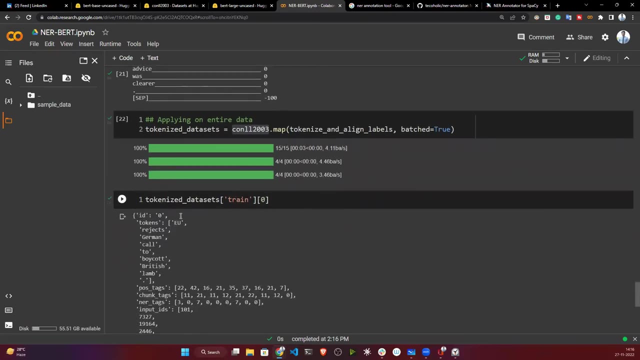 my uh, this con uh 2000. this is my raw data now it is tokenized data. now, if i show you one example from this tokenized data, the same thing i'm calling, i'm want to see the first information now if i print, now, if you see this is already tokenized uh here, if you see this is my input. 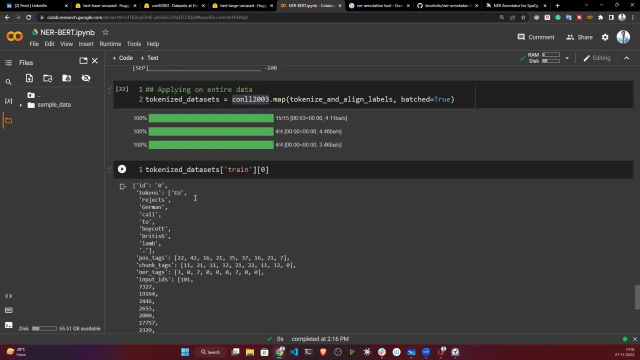 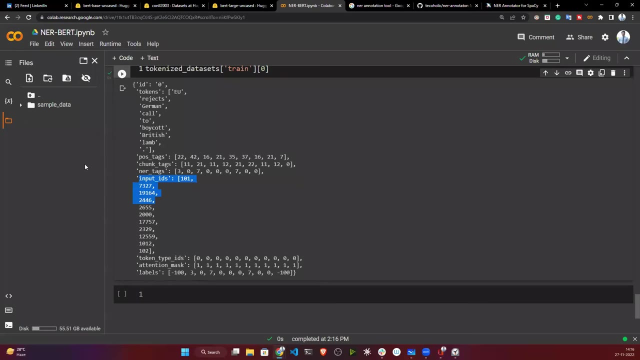 ids and all. okay, this is your token attention mask and this is your level, but i don't need information, pos, text chunks and ear tags. okay, i will remove it later on. okay, so this is. this is your pre-processed data. okay, now your data pre-processing is done. okay, data preparation. 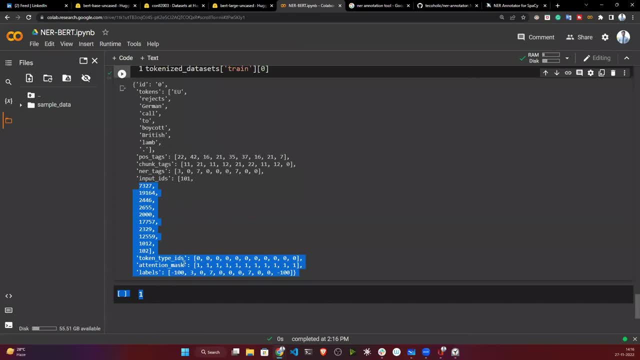 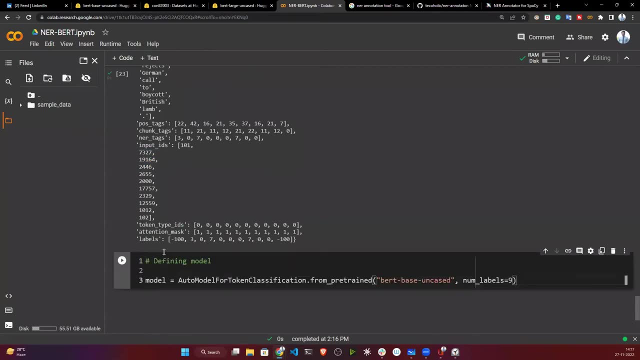 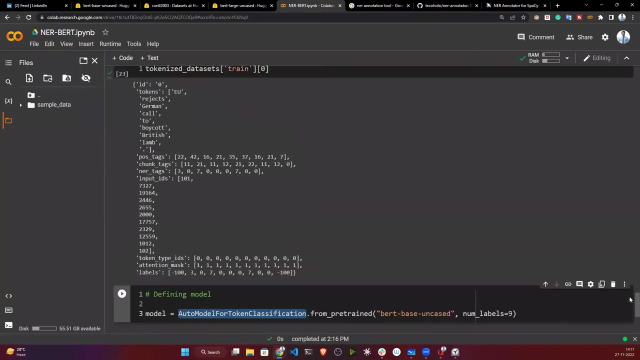 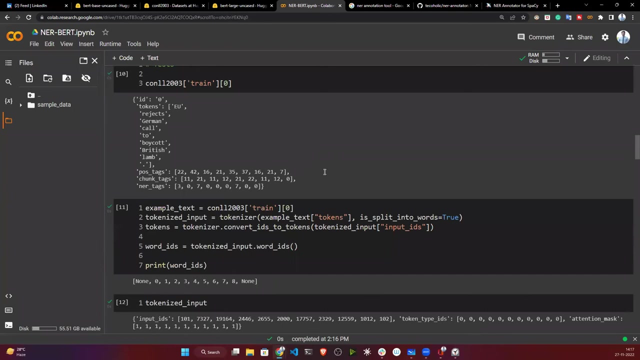 is done. okay, now you can define your model. okay, so this is the defining of the models i'm calling auto model for tokenization. i think you remember i imported one library class here, this one. okay, so this class actually is responsible to initialize your model. here again you have a method, call from pretend. here you will be naming. 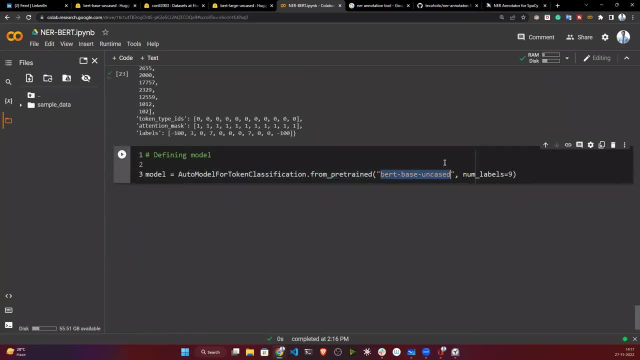 your model. okay, which model you want to use? i am using bart based unkeys model. i'm just defining as a string and i am defining my label is equal to nine. why i'm defining level is equal to nine. just write in the chat. if you have cleared with the concepts, i think you would be able to answer. 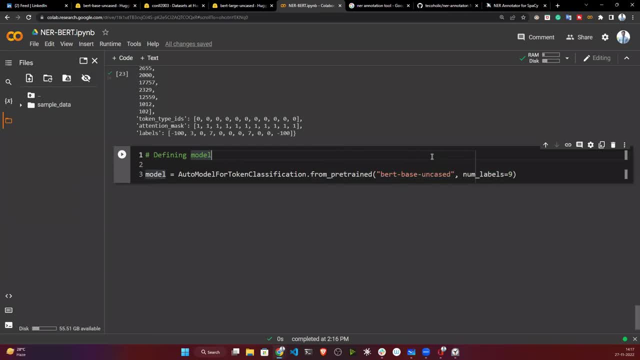 i think i already discussed in my whiteboard: okay, yes, nine, nine letter there. okay, i person b person. okay, i, organization b organization got it. so that's why, how many levels you have, you can define here. now just let's, let's run, it will download the model and it will. 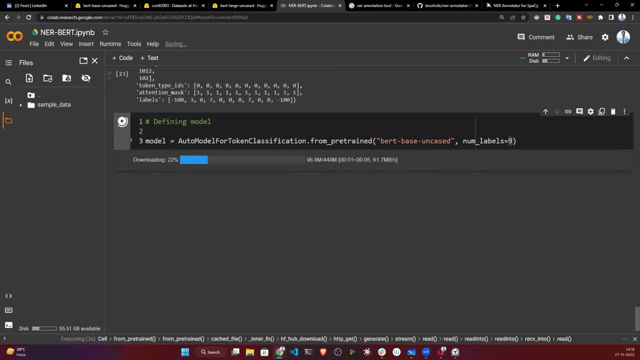 initialize, see, using hugging face api. it's like very easy here. you don't need to write any codes, you just call their high level api, just pass the input. okay, that's it now. model initializer legalization is done. but i need to do do some configuration to my model, because here i'm doing 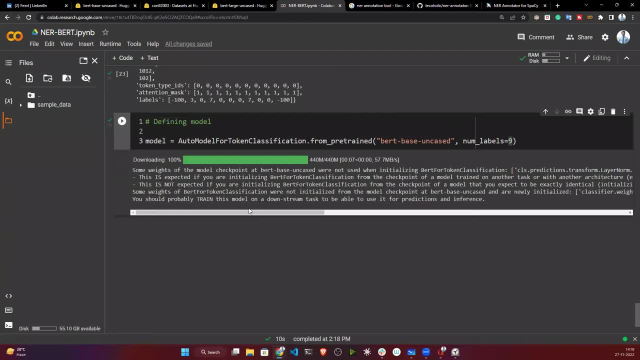 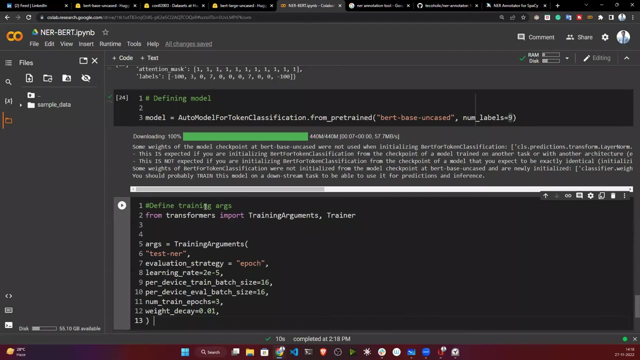 my custom training right. i'm fine tuning the butt model, so for that i need to set some of the arguments. okay, so again from the transformer, i am calling training arguments and trainer these two things and training arguments. inside i'm passing the name, okay, the name of project name you are passing. i'm giving test in here, so what it will. 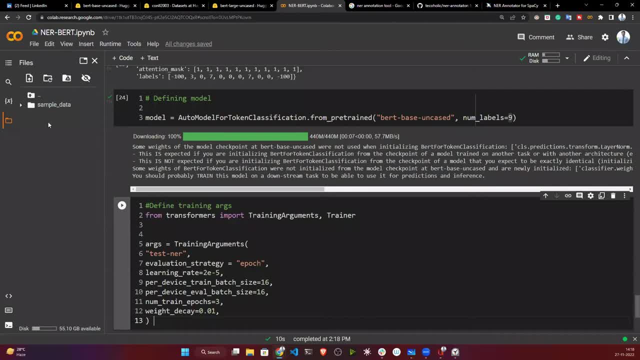 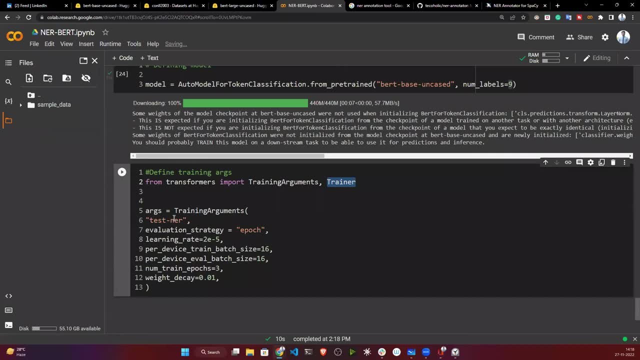 do whenever you will start the training. it will create one folder here. inside that folder it will all the logs, all the checkpoints. okay, you can give any name here. i have given test any year evaluation strategy. it is epox. you need to define as by default learning net. it is already by. 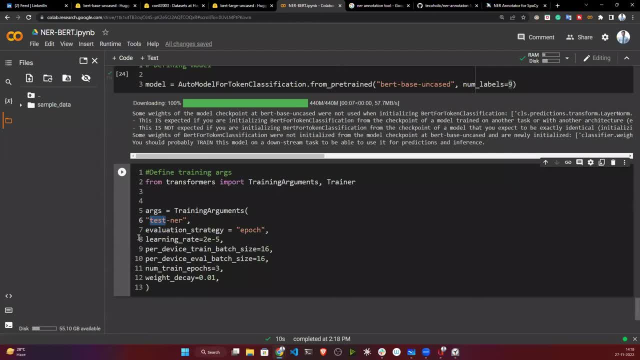 default. you can play with that. it is hyper parameter tuning, batch device training batch. you are defining 16. i am using free collapse, so that's why i'm keeping a 16. you can increase the size. a number of training epochs i'm defining as three, okay, but here you will see uh in training. 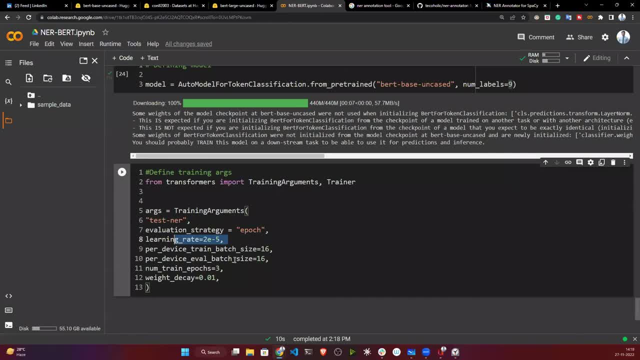 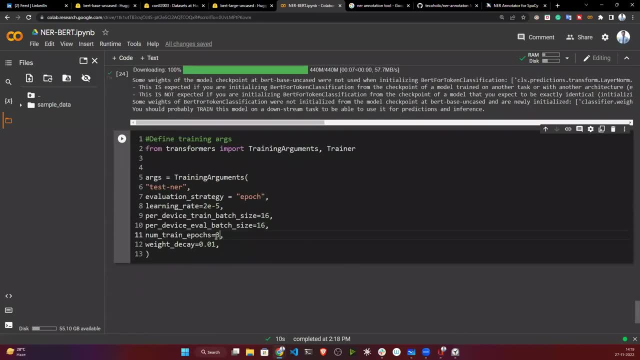 up, but likely it will take a lot of time. okay, let's decrease the epochs. let's keep it as one. okay, again, it will take time. that's why i'm keeping just one. but for your case, just increase the epoch size. okay, i trained three epochs last night. it was giving me almost good results because 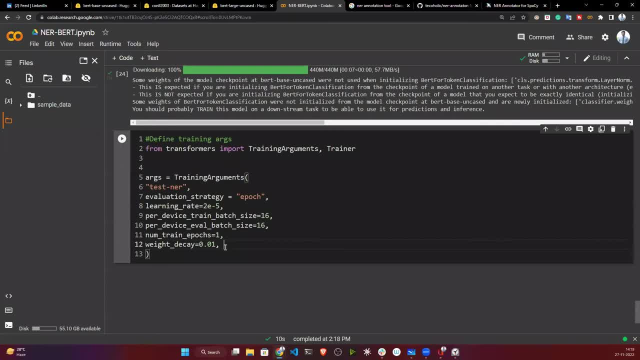 it is one of the bigger model- okay now, where decay just keep that- different settings only. okay, now let's execute. so these are the arguments actually you need to provide before initializing your training. now i will call my data collator. i think you remember this is the data collator. i. 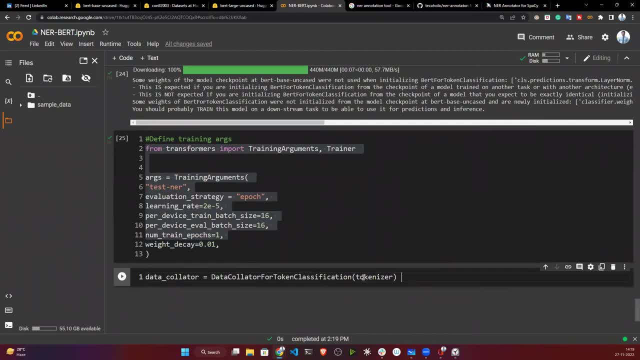 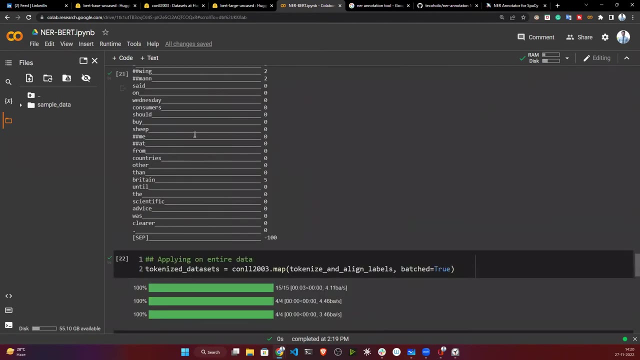 defined and it will take your tokenizer- tokenizer as a input. okay, i defined my tokenizer, i initialized. i think you remember tokenizer. see, this is my tokenizer i initialized. okay, so that is what i am passing here and this is a data collator objects you are creating. let's run. 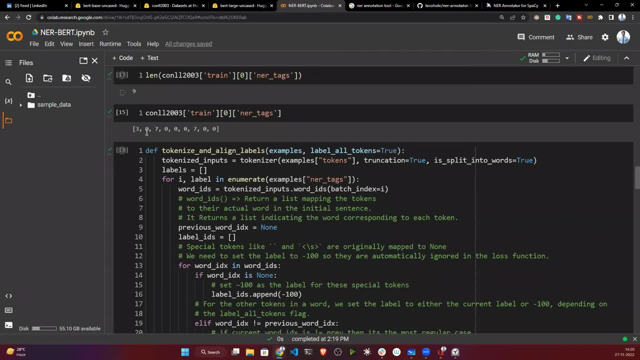 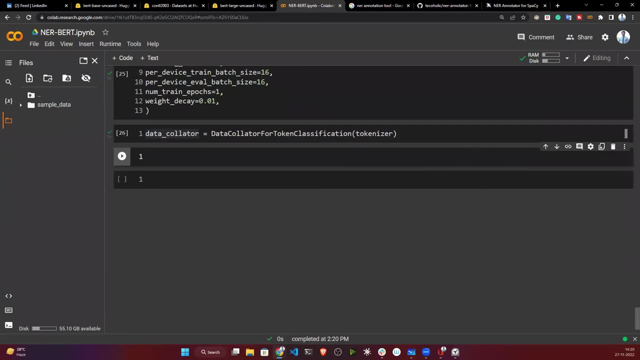 it. so what you need? you need some metrics, like to cal, to see, like, how your model is performing so inside. but if you want to do any year, uh, and for any year, actually there is one matrix we use frequently which is nothing but uh, sake, evil. okay, this is one of the metrics. okay, sake, evil. 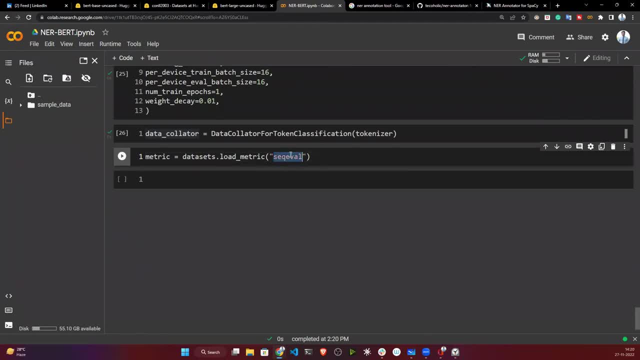 if you want, if you want to learn more, just search about sake evil, you will get. but i will suggest, just try to understand as a like high level, so what it will return. it will return your pre-seasoned recall, all the score actually. okay, i will show you. let's, let's test on one example. okay, 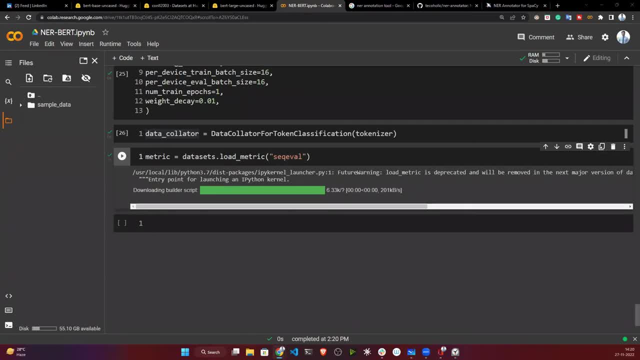 how this matrix is working. so let's take one example. so i will take one example for this train. then what i am doing here. i am first of all listing out all my level name. yes, it is specific for any year. like token token level classification. it is only specific token level classification. okay, like token classification you can talk about. 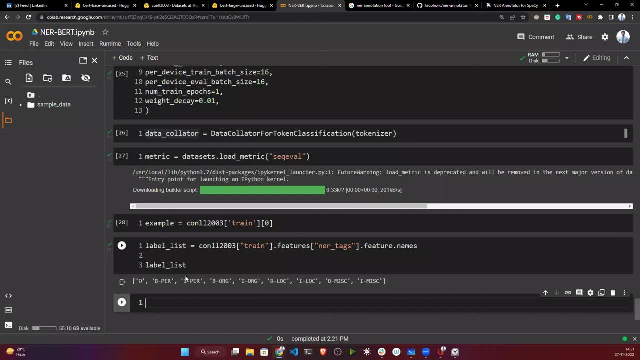 okay now, if you see these are my all my levels. okay now, and what is my example tokens? this is my data, any attacks if i want to print. so this is my index. okay, this is my index id. now, if i provide the index id to this list, it will give me the name. 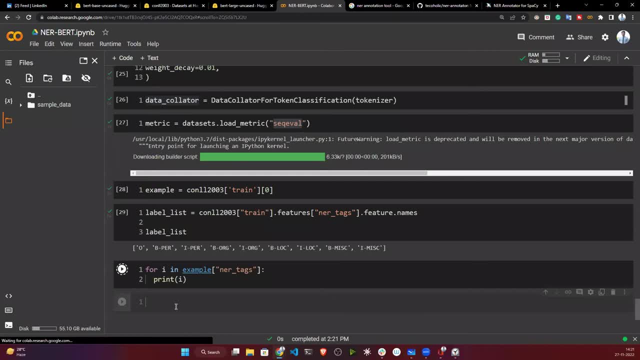 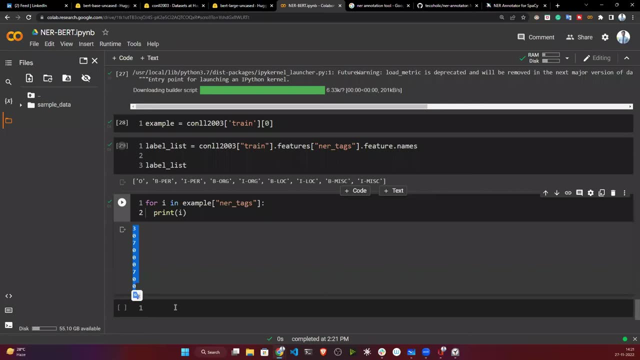 okay, let's take it also. so this is the code for that. now i have all my uh, you can say level name. okay, this is the first example i'm taking. okay with that, my level name i have now, if, if you want to compute the matrix. so this is the code. 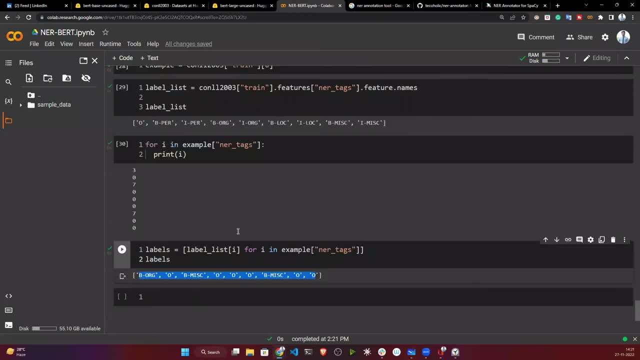 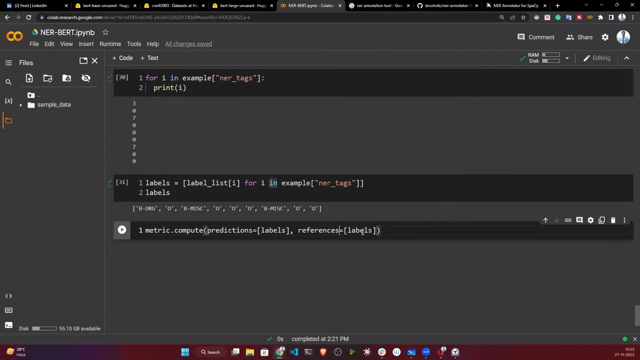 so here you need to pass three, two things. one is your prediction, the prediction level you will get from your model, and the reference. that means your actual one, but here, just for the testing purpose, i'm giving this this thing twice. okay, here also, here also. so it will give me 100 results, guys, if i, if i run it, you will see, it will give me 100. 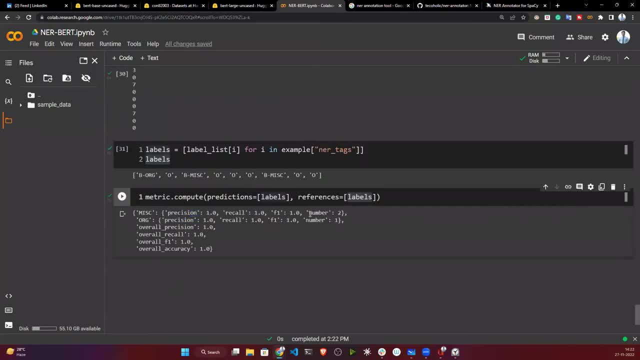 percent result: position: 1.0 equal 1.0. f1: 1.0. okay, it is giving 100 results. because? why? because it is true already. if you see this, this level, i have passed twice. okay again if i print it. so all the. 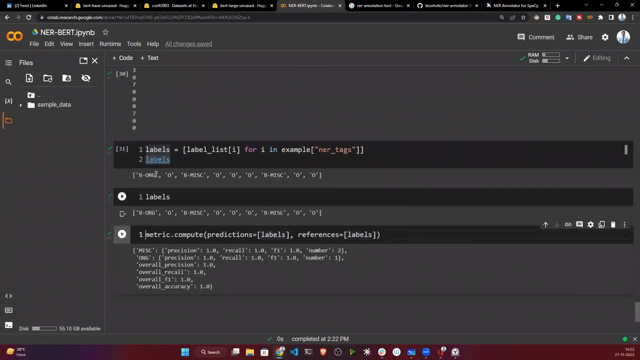 labels is matching. see it just like i think you know. classification like accuracy, score how it works it. see like whether this two is matching or not. okay, that's actually it's working. but whenever i will be training, it will be coming from the prediction and here i'll be providing. 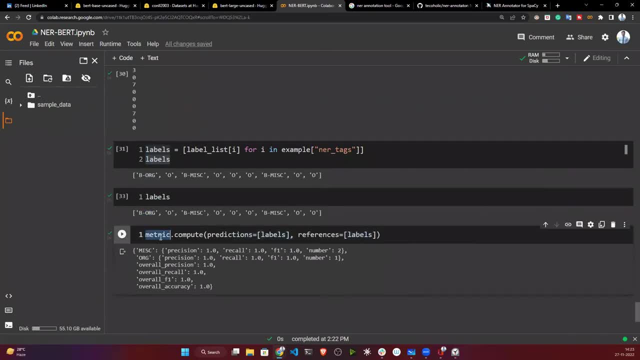 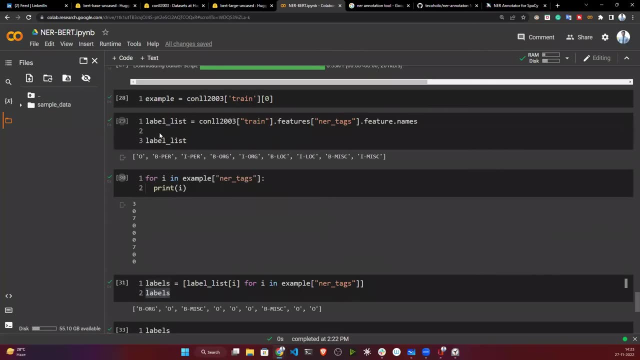 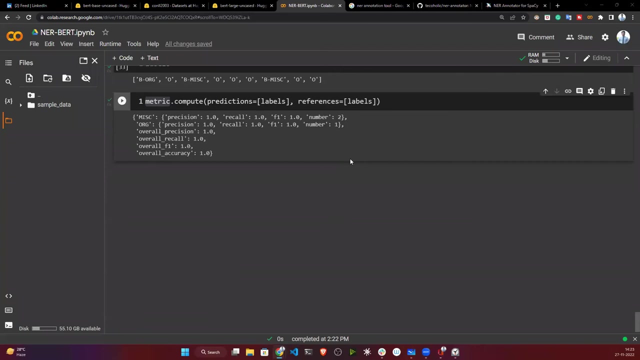 my actual levels. okay, that's actually your matrix. works this, your uh, this matrix? actually? segwell is working? okay, it will give you. these are the score, actually precision recall f1 score and all okay, now let's define our compute matrix function for my model. so this is the function. okay, just keep it as template. so here, first of all, i'm calculating. 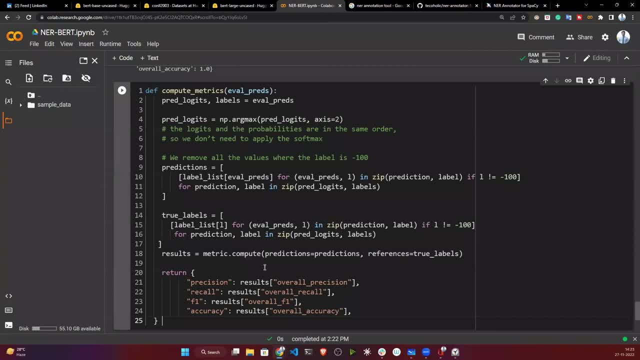 my prediction, my true level, and inside that i'm passing, see prediction. i'm passing as my prediction and reference and passing my true levels. okay, then, at the last i'm returning some of the information: precision, recall, f1 score and accuracy score. okay, now let's execute. 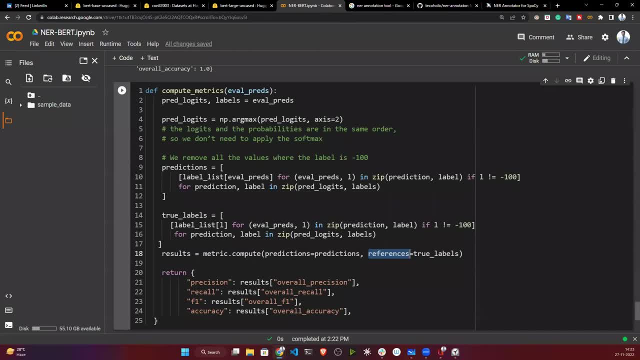 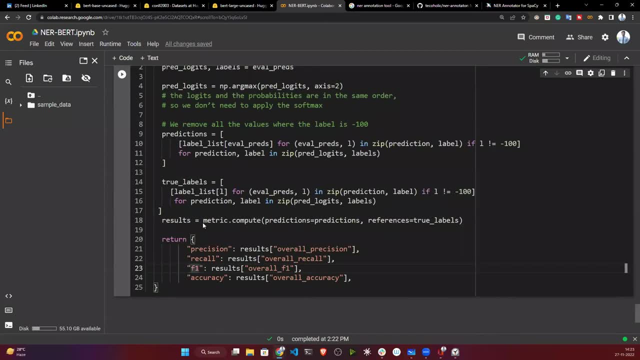 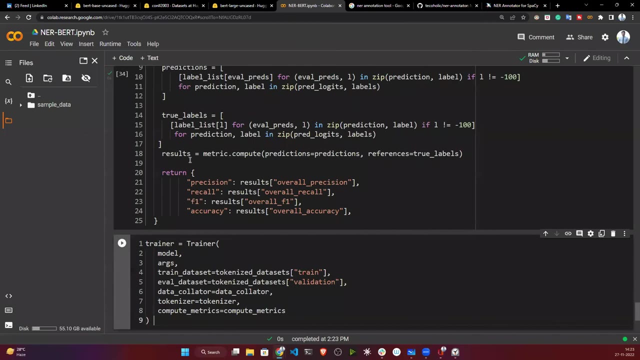 now we can start our training. so this is the training code. so here i am, defined trainer, i think you remember i initialized trainer here. okay, trainer. so inside trainer, you need to pass all the thing, whichever you have initialized. so i have initialized my model. i think you remember arguments i also initialized, i think you remember, here. 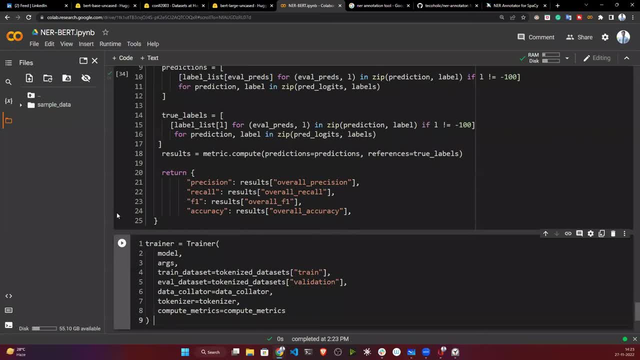 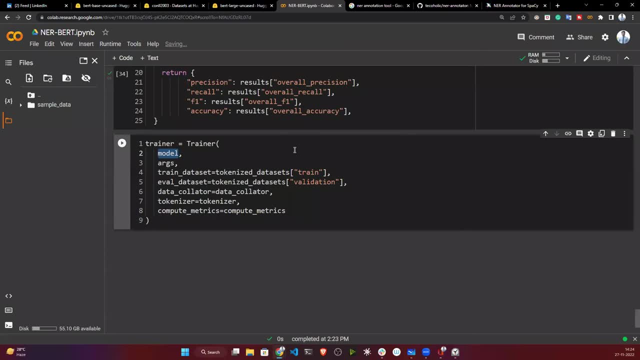 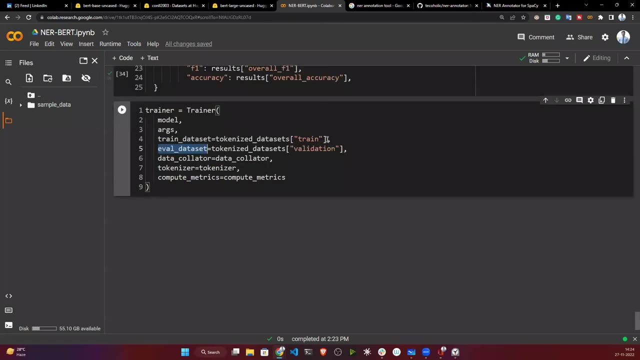 arguments. then i need to pass my train data set, that is, my tokenized data set train. i need to provide my evaluation data set. uh, tokenized data set validation. you are calling because if you see what is token tokenized data here, if you see tokenized data, if you print here you have three things like train validation and 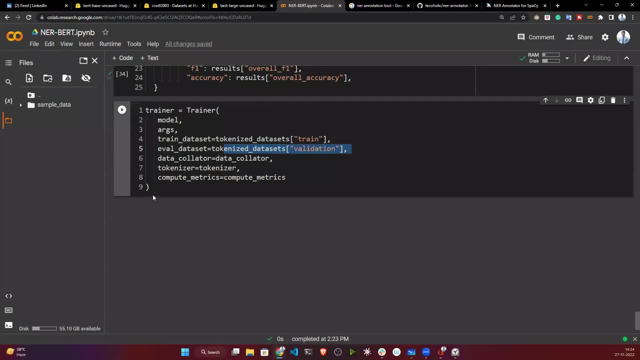 test right. i'm keeping these two things okay because it is already tokenized for me and i'm providing my data collator. i think you remember i also defined data collator here. this is the data collator. it will apply some augmentation, it will define the batch and all. 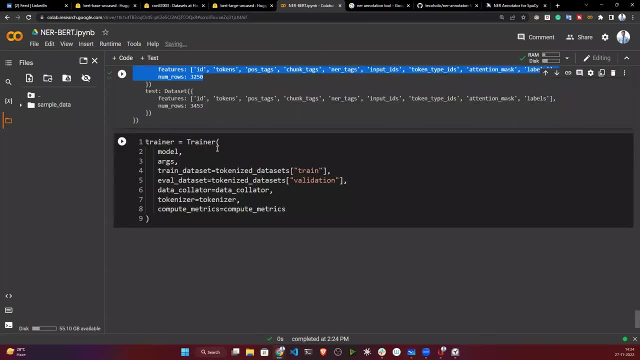 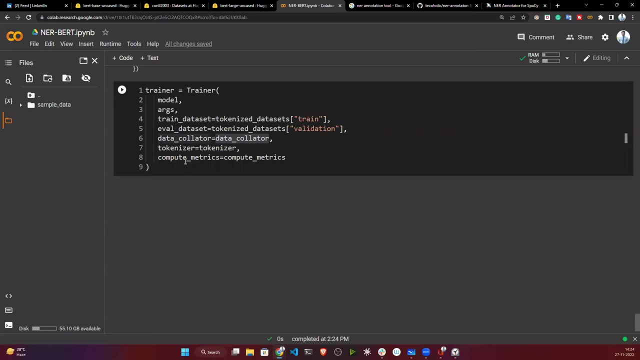 tokenizer i already defined. i am passing my tokenizer compute matrix, compute matrix. this function i am passing okay. so these are the argument you need to pass okay before initialize the before starting the training. now it is initialized, now i can start the training. so to start the training, there is just one function you need to call, which is nothing. 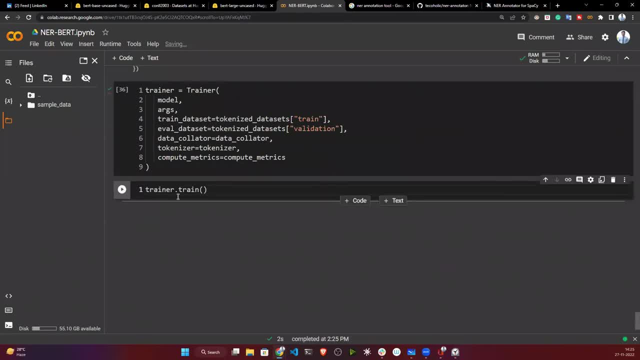 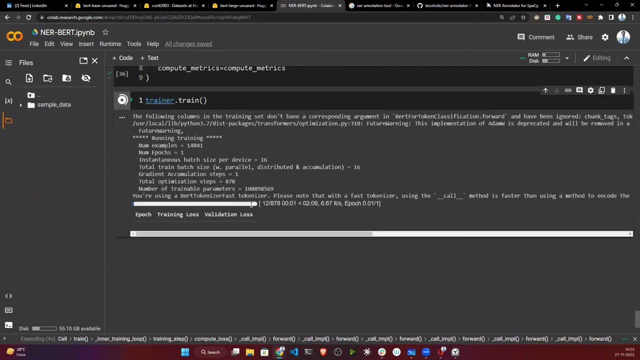 but dot train. okay, now, let's click here. now you will see it will start the training. see, now see the training is started. now you will see it will start the training. now see the time you can see. although i'm training one epochs again, it's taking time. 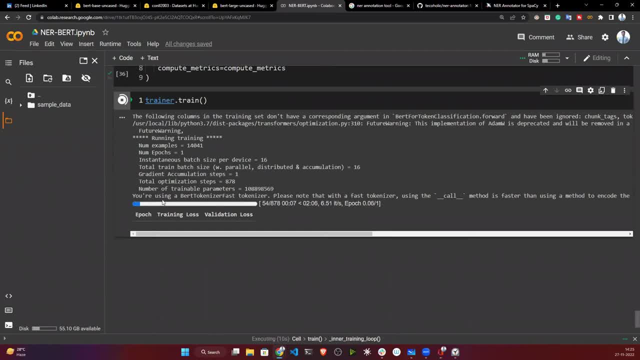 okay, and after each and every epochs you will see the epochs training loss, validation loss and at the accuracy score the logging is very good. this hugging face guy has done like everything you can track from here. only see number of example, number of epochs, everything you can see here. 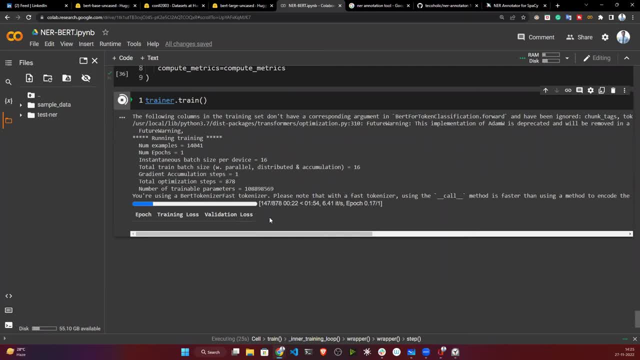 number of trainable parameters. see that that many of parameters you are training currently okay. so now let's see how big this model is. that's why i told you creating training pipeline in nlp it's like very difficult. so always we try to train our model first, then we try to create the web application and all. 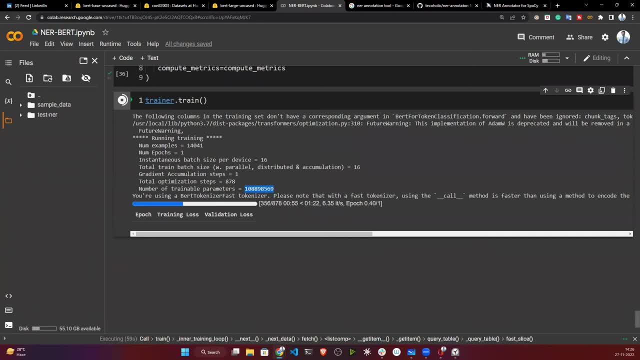 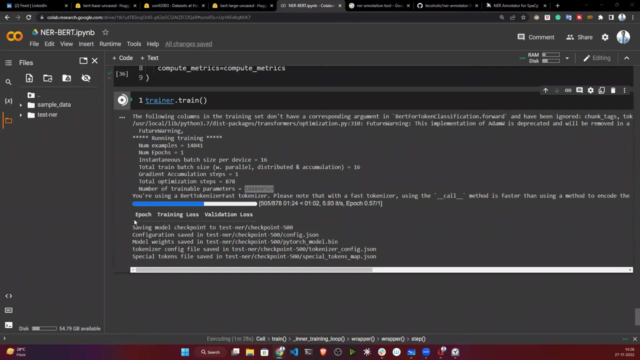 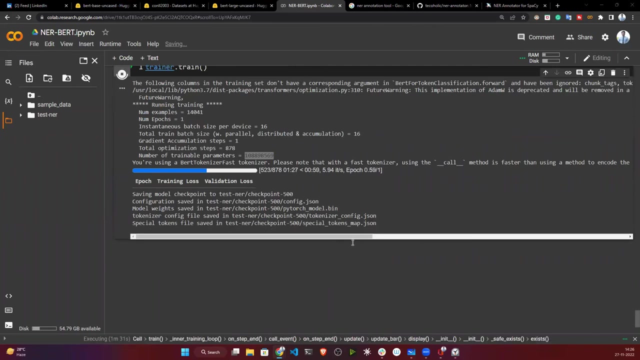 i think, till this point, everything is clear. guys, just tell me yes or no. it is understandable everything. it is understandable everything. right, something, yes or no, guys? okay, let's wait for the training, okay, okay now, if you refresh here, you will see test engineer has been created. now, if you expand. 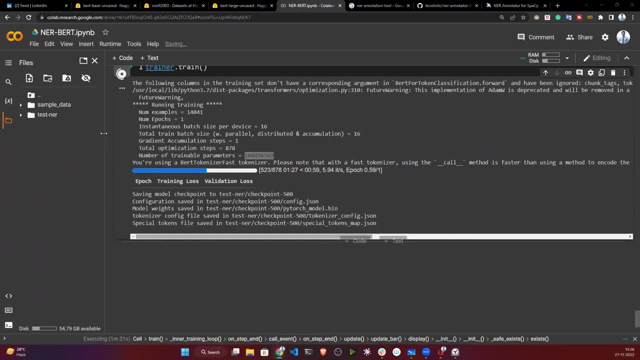 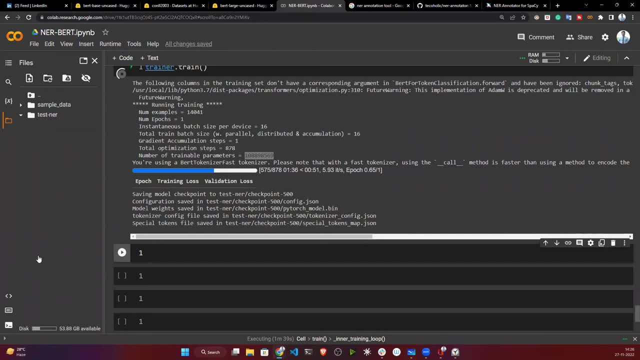 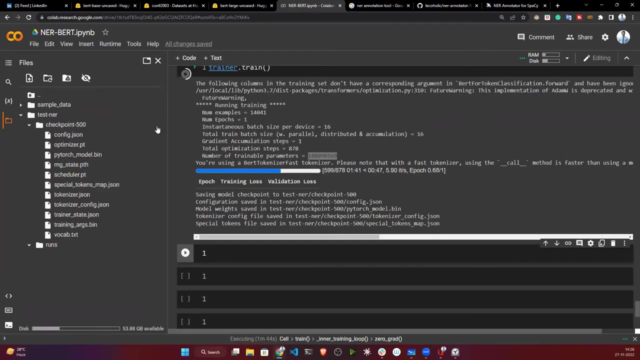 you will see all the checkpoints it will save. okay, inside runs. it will save the metadata. see, it is also logging the date and the month i ran this code, all the metadata it will everything. it will save here. okay, if you want to see the configuration, everything it will say. 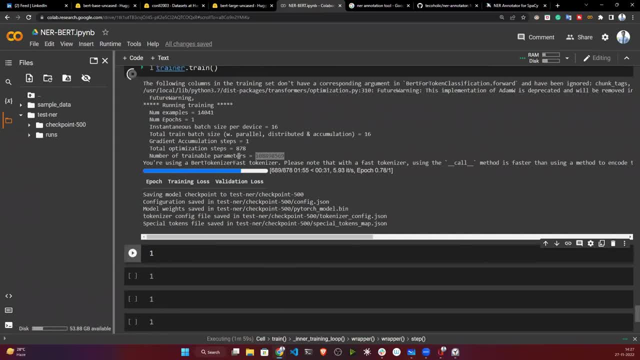 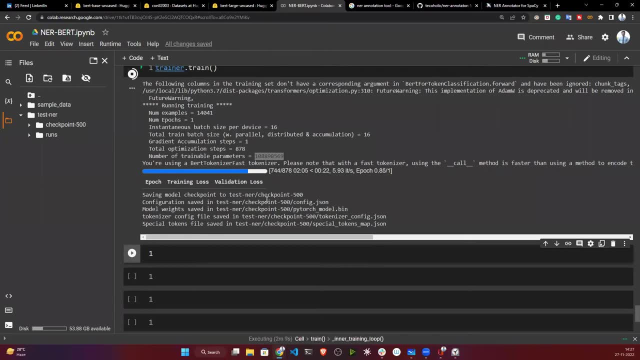 so i will show you how to save the model and how to load the model and how to train it. this is the custom data set i am training guys. it's not like i'm using any, just here. it is already labeled. if you see, it is already annotated. okay, and i showed you how to annotate. 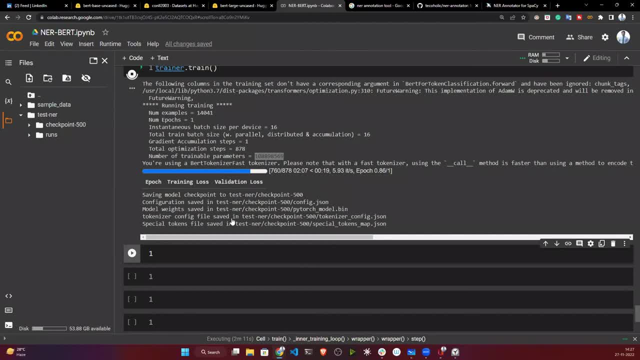 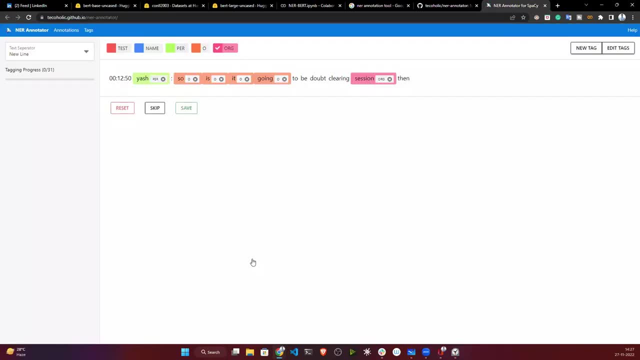 the data using this tool, because nlp annotation is like very time taking. i can't annotate all the data, okay, so here you need to always download the data as an annotated format and you can pass it. this is your code. custom data only got it. i showed you each and every things: how i pre-processed it, how i tokenized it. 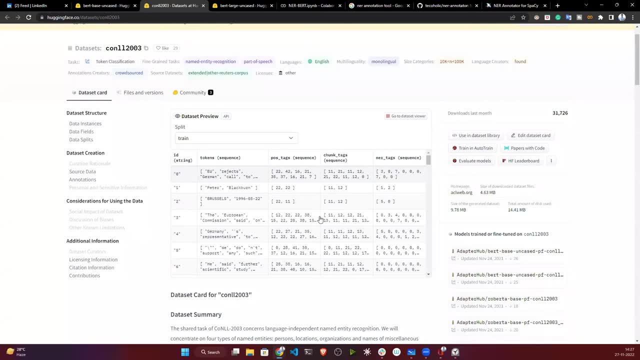 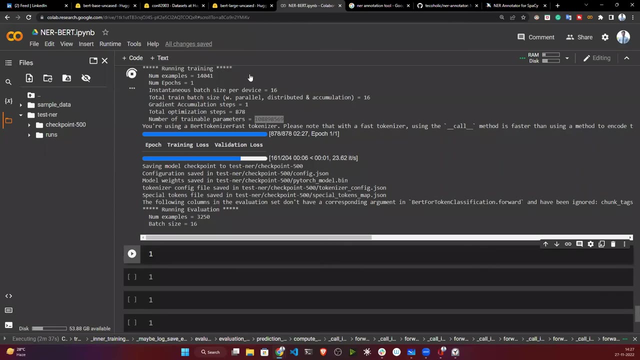 how it came. actually, i showed everything, yes, row by row. here suppose this is one example. you have first of all how it was okay, it was like a text. only what you did, you first of all tokenized, tokenized. then you have all the list, then each and every list you have annotated, like one by one, 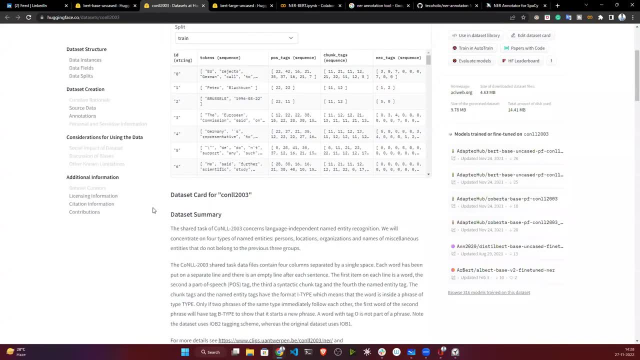 yes, i will show you after training how to load the model and all. just wait. okay, now see, training is done here. if you see pox, training loss, validation, loss, position recall, f1 score and accuracy: see, i just given just one training. the accuracy i'm getting 0.98. 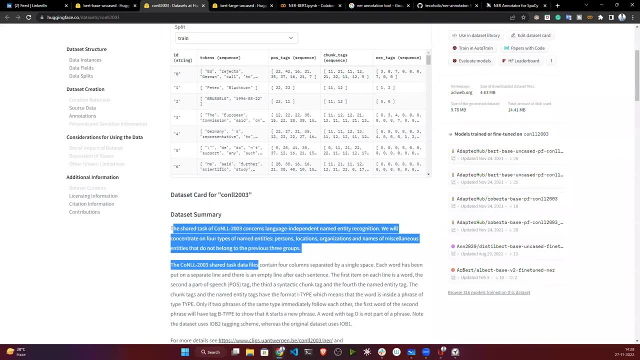 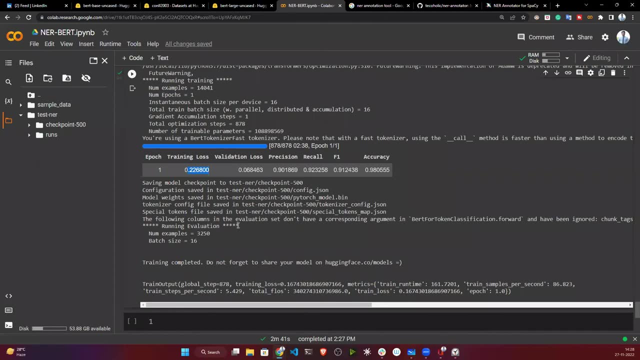 okay, now let's see how to save the model. so to save the model, just write this code: modelfap- pretend, name them. name like: provide the name you want, any name you can give. okay, i'm giving any year model now. like, if i execute now, if you refresh here, any model is there, okay, inside you. 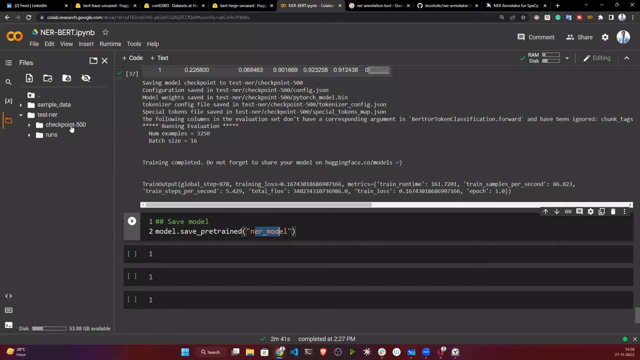 have. this is your model pytorch model bin and, with respect to that, you have one configjson file. here you have all the model configuration. okay, what are the weight decay, landing rate? everything you have selected, everything is there. okay, now, again, with that, you need to save your tokenizer also. 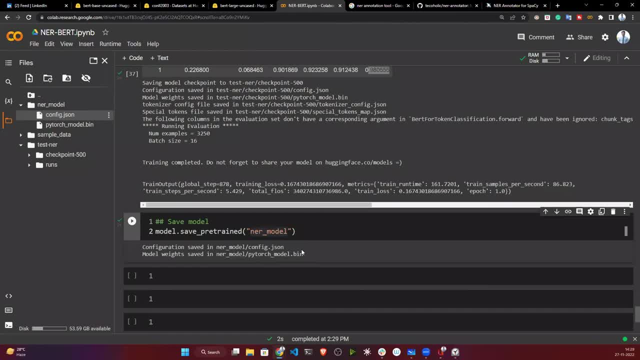 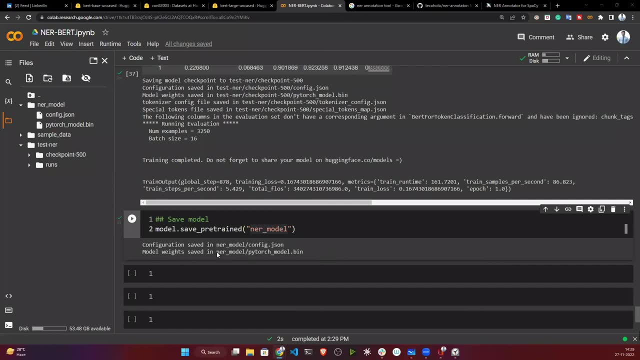 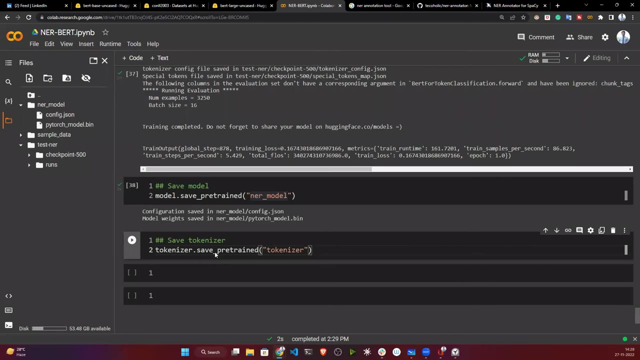 because i'm if i'm providing any uh test data, so first of all it should be tokenized right, as the tokenized id didn't did my training, so for that i need to also save my tokenizer. this is the code for tokenizer. now let's also refresh here. so this is the tokenizer instead. 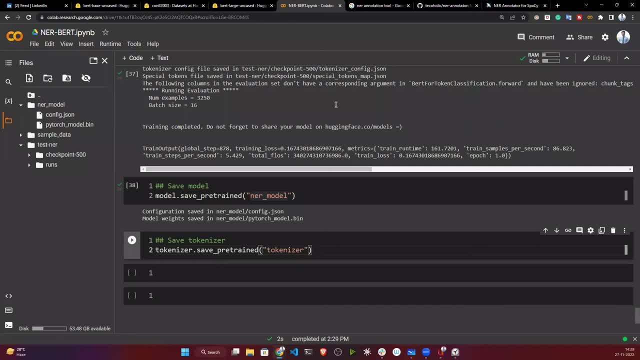 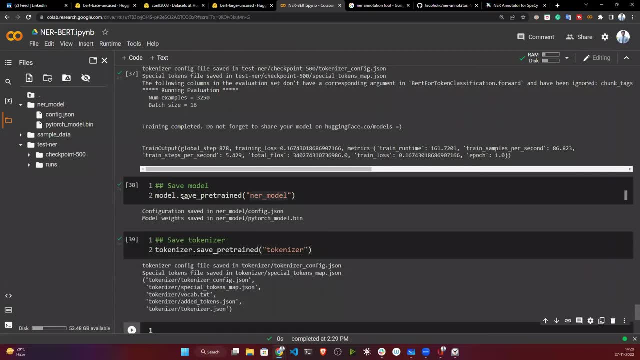 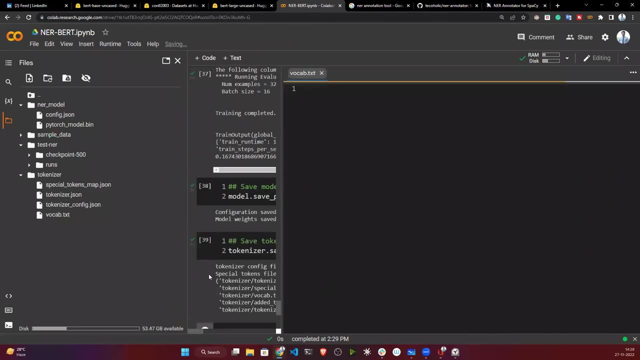 see you have all the vocabulary list and everything. okay, the required files and everything you have. so these are the thing actually you need to save. now, what you need to do, you need to define two things. one is your uh, label- id to label and label to id. okay, because this is. 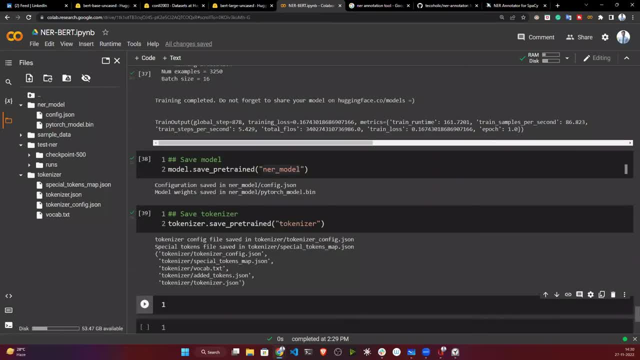 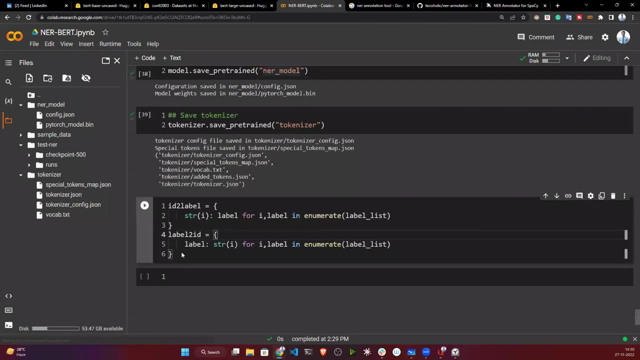 important to pass to your configuration. okay, see, first of all, i am converting id to label. that means this is my id and this is my label. i'm providing some id as a dictionary. okay, then the same thing i'm doing as just opposite. okay, if i show you label to id. 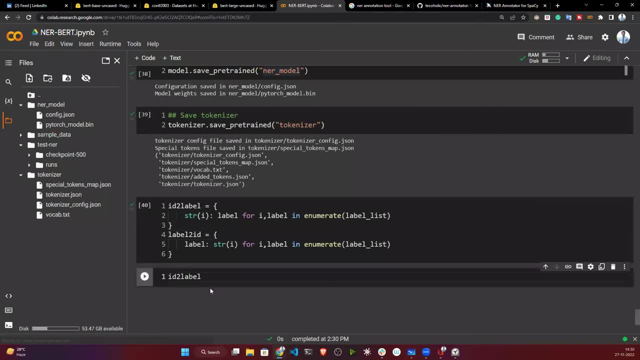 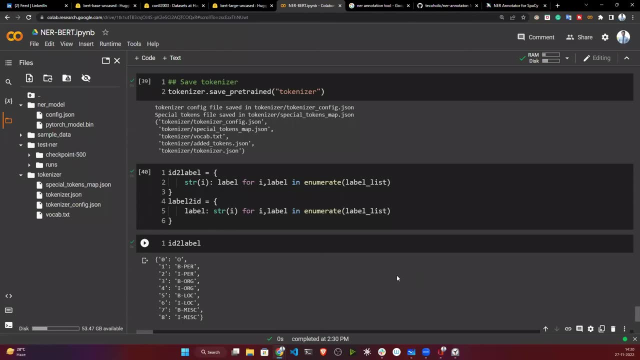 okay, like, this is my level and this is my id- unique id, because it will help me during prediction. okay, now what i need to do. i need to suppose you have saved your model and all now. now you can download. these are the thing. okay, you can download these two file. 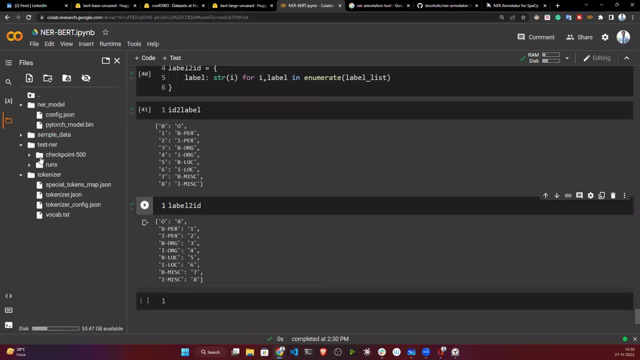 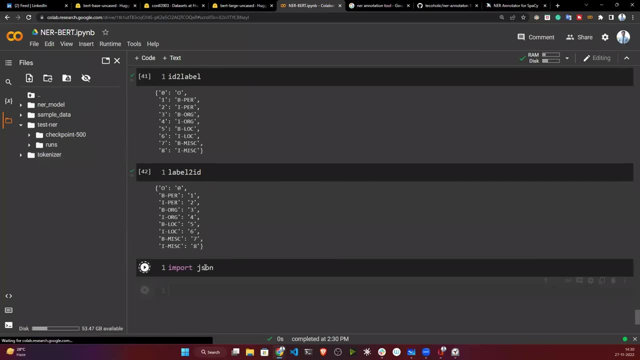 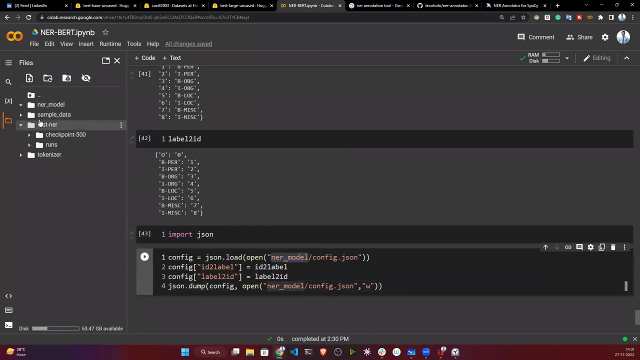 one is your ner model, one is your tokenizer in your local and how your local code will look like. first of all, you need to import json. you need to load the configuration first of all. load configuration means ner model. there is a config file, configjson. okay, this is the. 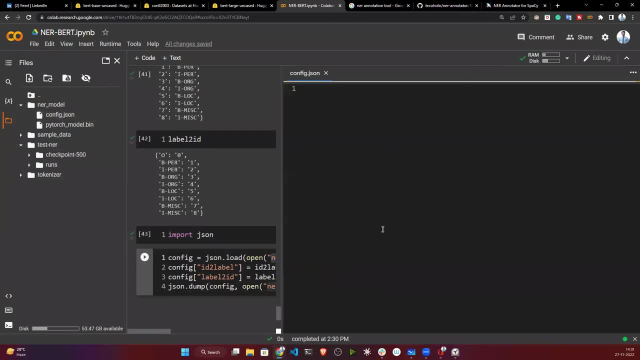 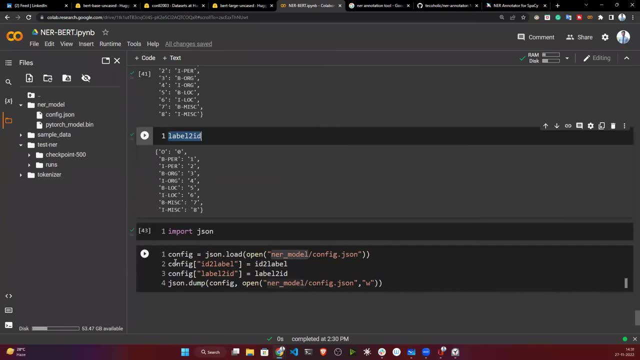 configured configuration file. so here you need to add these two things. one is like your label to id to label and label to id. okay, that is what i am doing. see, i'm creating another- you can say, fee inside key. i'm restoring the value, okay, and after that i'm dumping the same. 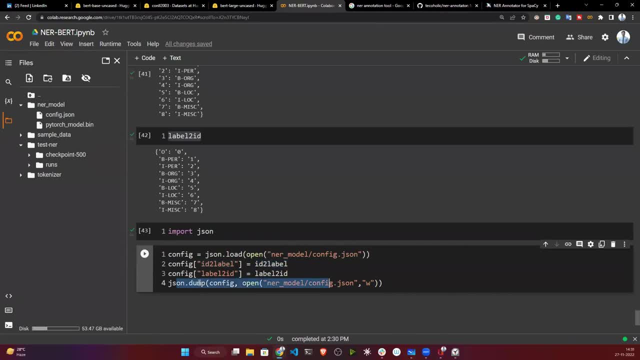 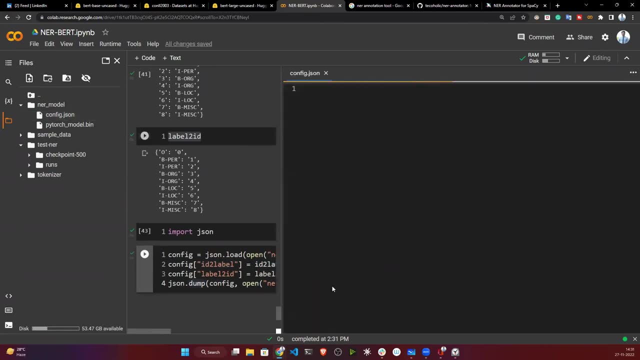 json file. okay, first of all i'm loading, then i'm dumping. now, if i execute, now, if i again refresh and if i again call open the configjson now you'll see it has been changed. okay, now all my label name you can see here. okay, so this changes you need to do. 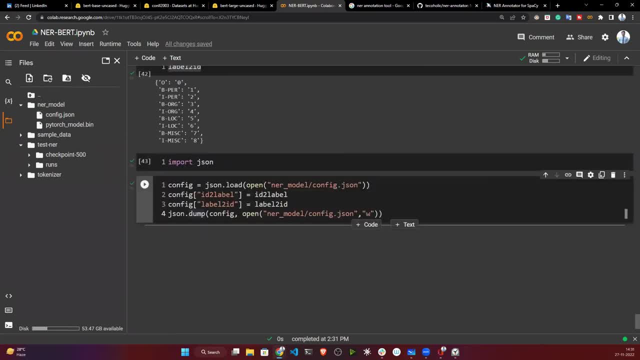 now, once it is done. now you can load your model, your fine-tuned model, whichever you have trained, just provide the name, that is, ner model. it will automatically pick up this pytorch modelbin. with respect to that, it will automatically pick up this configjson. okay, now let's execute. see, it has loaded everything and 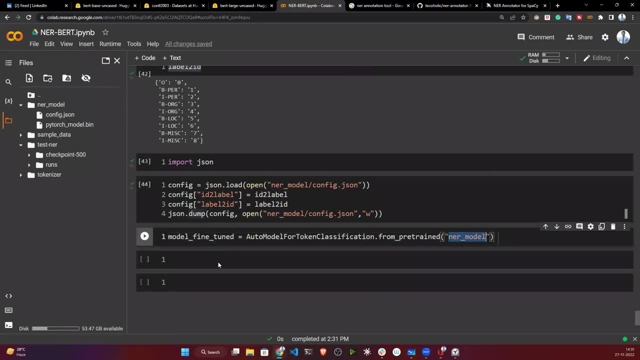 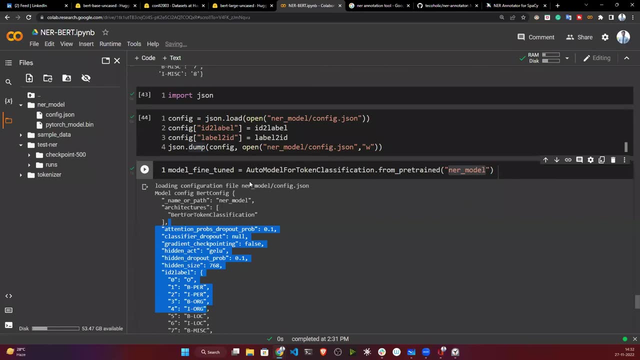 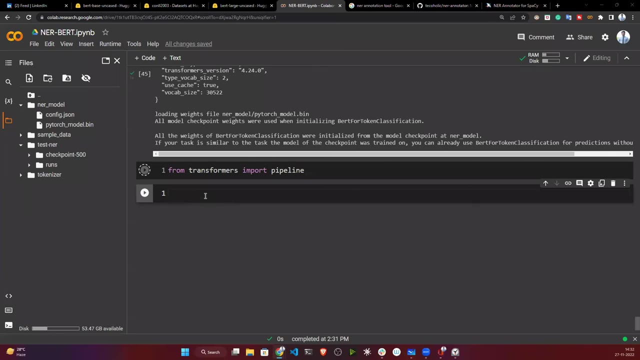 you can see. see, you have set this configuration already. every configuration you would be able to see here now. once it is done, now just call the pipeline from the transformer. okay, now initialize your pipeline. so nlp, i'm giving as just a variable name pipeline. what task you want to perform, give any. 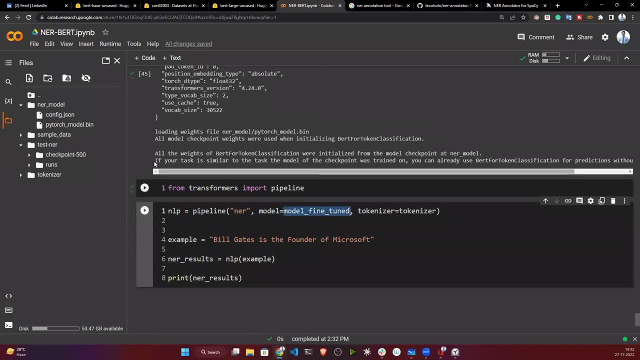 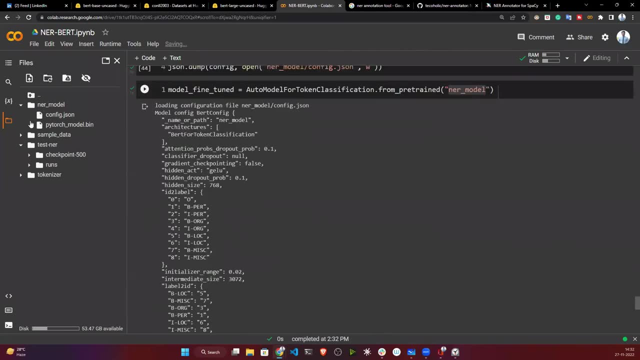 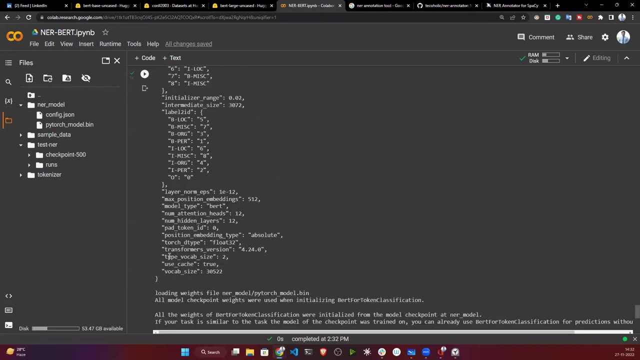 model, your model: fine tune, that means you have imported the model already. this model, just pass your training model. tokenizer: the same tokenizer you you already dumped here, which is i already loaded here, i think, if you see tokenizer. okay, so pass the tokenizer. and this is my example code. 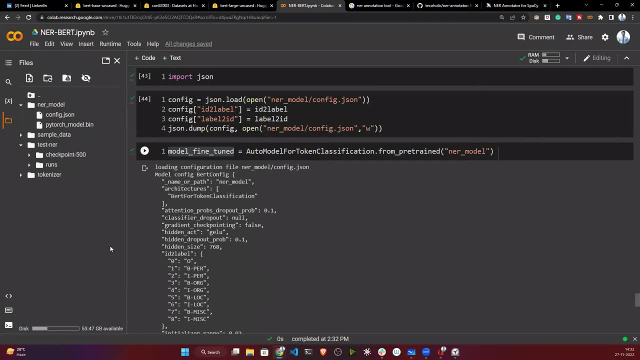 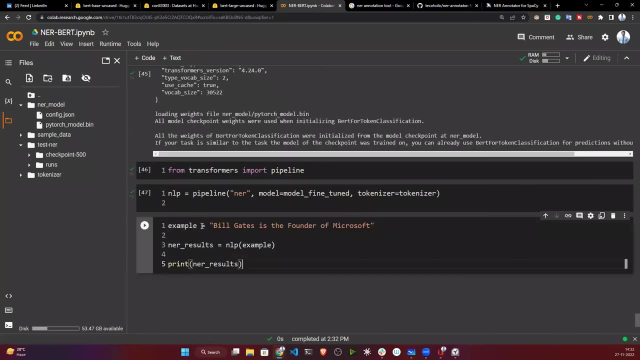 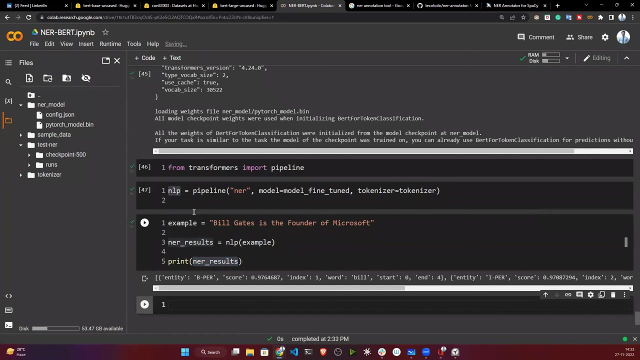 support. let's initialize the model first. i will cut, so it will initialize my pretend model. now, if i provide one example, suppose bill gates is the founder of microsoft, the same example i am passing, i am calling my nlp this model, passing the example, printing the results now. let's print, now you can see the entity, now b person you are getting with. 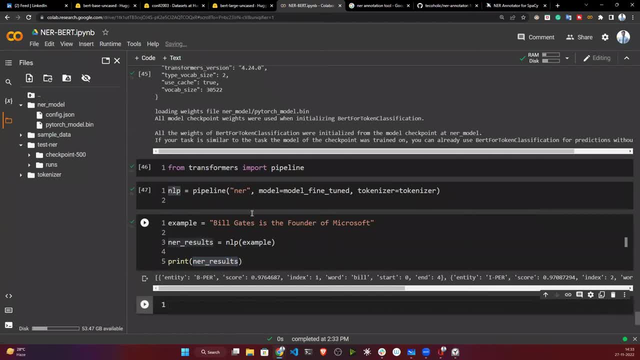 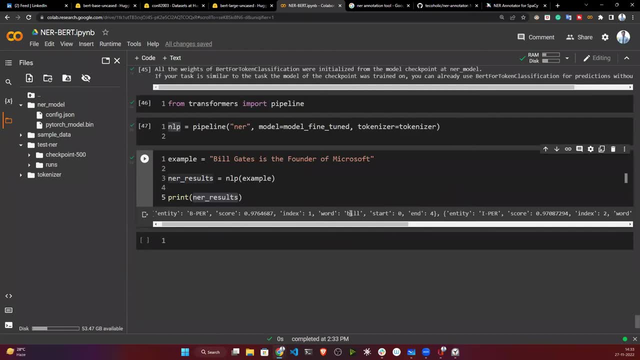 the score of 0.90. index. one word: bill. so bill is what bill is a person? right, you are getting b person. is what b is the beginning of the sentence? you are getting b person, okay now. second entity, you are getting i person, which is nothing, but your gets that is inside of the person. and the third. 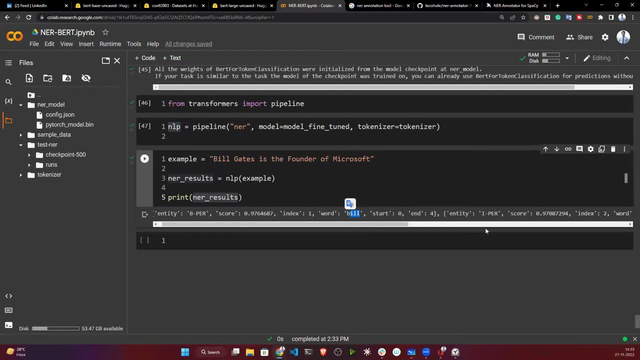 you are getting microsoft. that means organization, because here it is not considering the uh designation. okay, and all the objects you can see is the off it will automatically ignore. okay, now i am able to extract the relevant information from this text. i think it should be clear now. 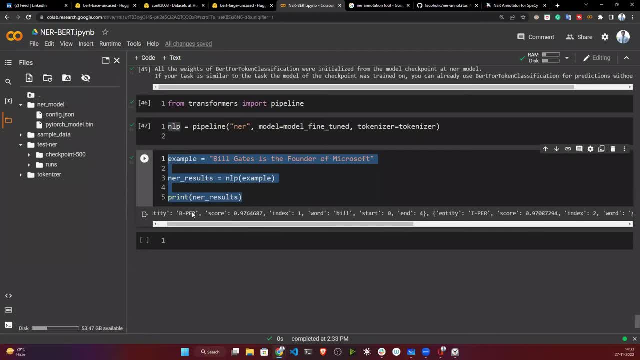 this is your final output. now try to extract the output. try to show okay in your ui. suppose this is your inputted text. with respect to that, i have extracted. these are the information. guys. clear how to load your pretend model and how to do the inferencing. 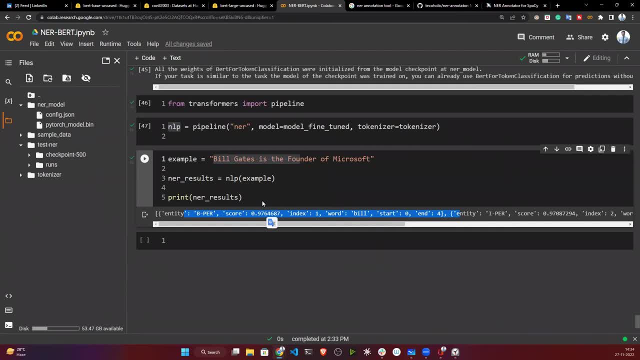 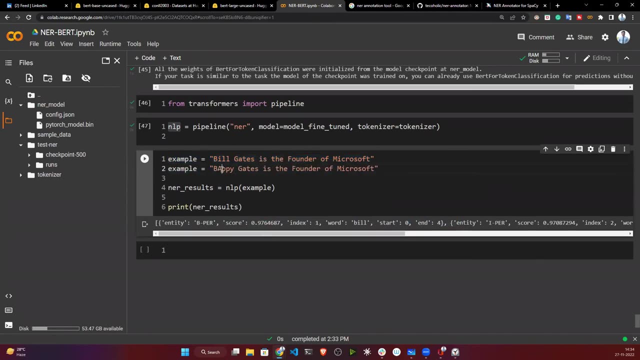 yes or no. yes, i can give another name. let's give another name here. let's copy the example. let's give my name now, if you see. see, it is doing sub-level tokenization. もうpell nowvo하하 Mis Ali. first of all, it is doing the tokenization. if it is not able to understand the 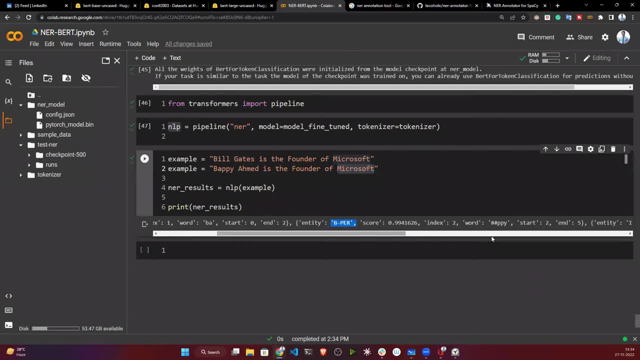 world. it will do subtokenization using hashash right now. if you see, ah, はい, ah, Croatian is again person that is inside of the person, then entity you can see here, microsoft is, is what it's. our organization got it, guys, clear. visualize prediction. you can write some of the code like you can use matplotlib anything. 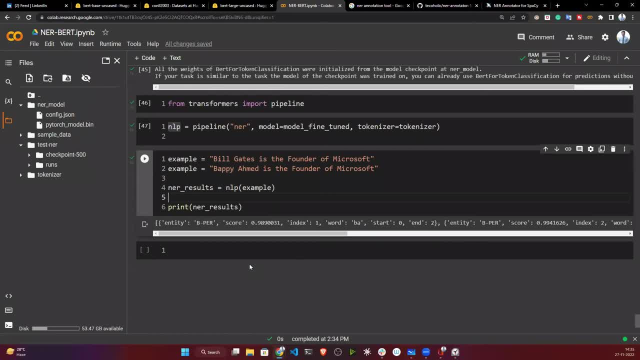 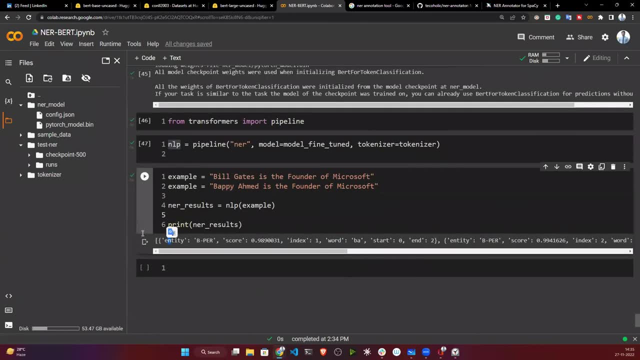 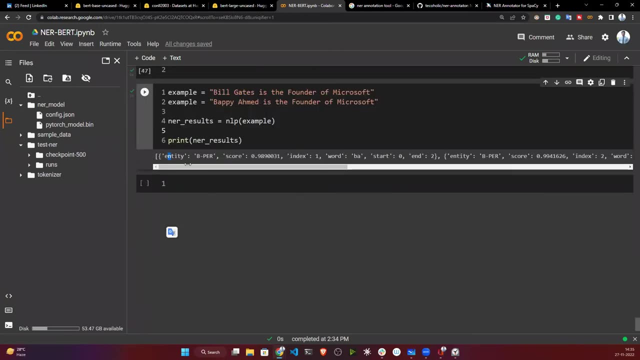 you can do the visualization. it's up to you. okay, but this is your final prediction. this is your code, like you need to run. now you have the entire idea how to create your own ner model. it should be clear, guys. so one task is clear: how to create any model. you can do these projects. 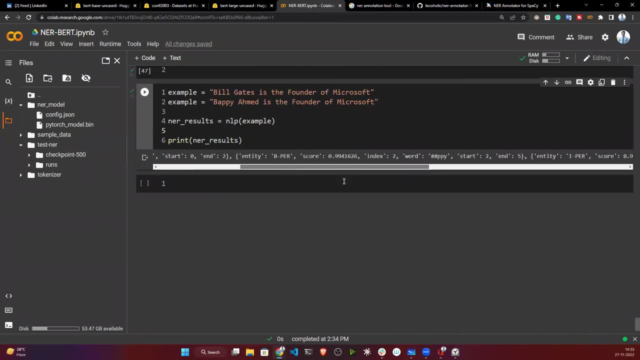 suppose if i give you resume data, if i give you check data, you can perform. first of all, you need to prepare data somehow like that. okay, how to prepare, you know python, you know pandas, just do it. prepare your data, got it. try to bring your data in that format. try to. 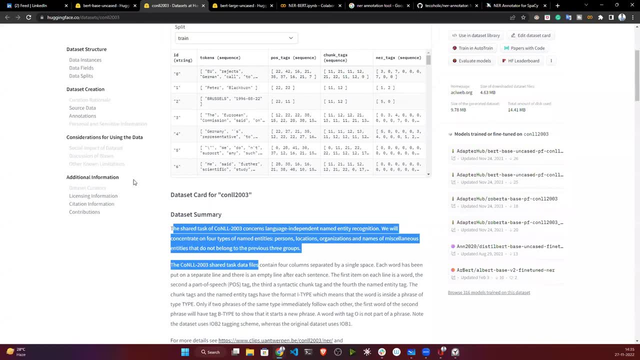 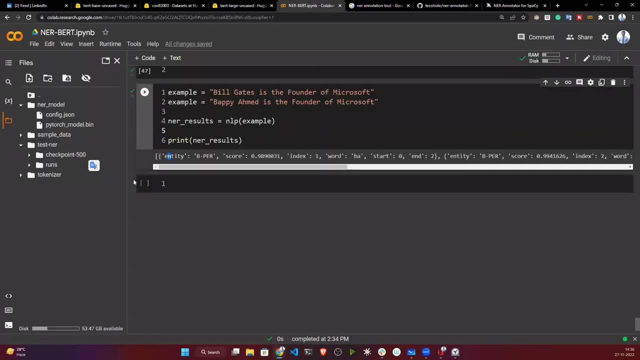 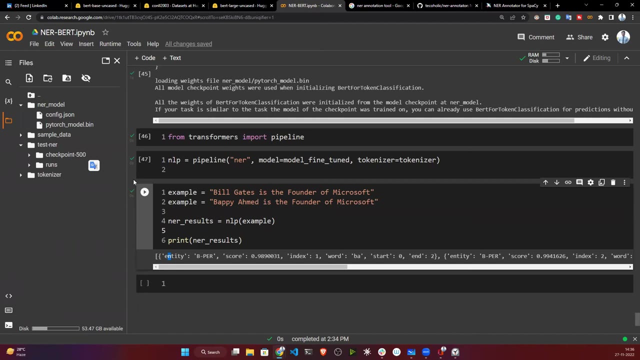 apply the same thing, this notebook. that's it. okay, guys, is it clear? guys just tell me yes or no. it was very easy and i have broken down each and everything's as a component and i explain like: okay, so this is nothing, but your any unlimited recognition? okay, you fine-tune in the part. but 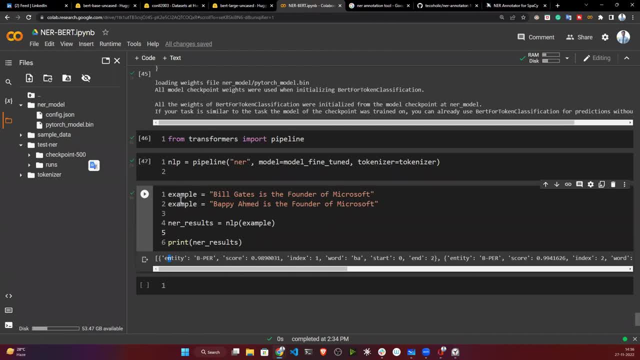 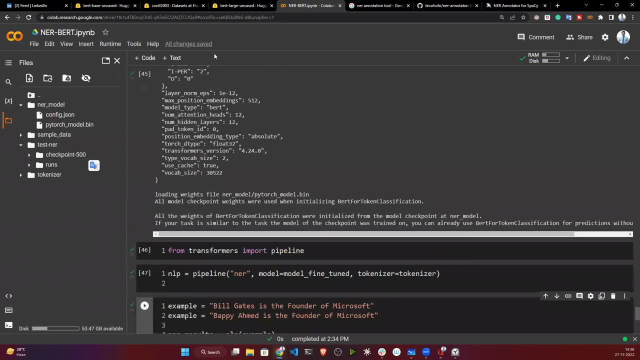 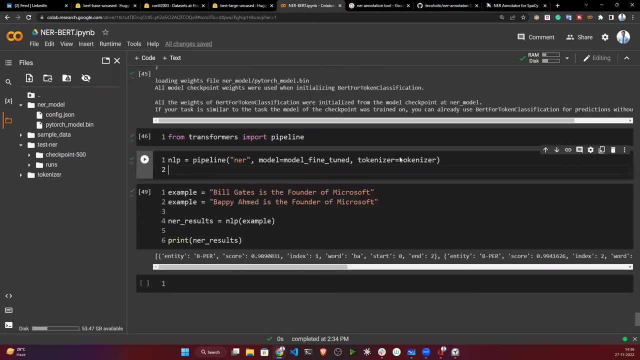 suppose you don't want to fine-tune the part. okay, suppose here i am using my own model, my own pretend model, but you want to use the like already, model like available inside here. just copy the name. okay, just give here model name. tokenizer. use the default tokenizer. 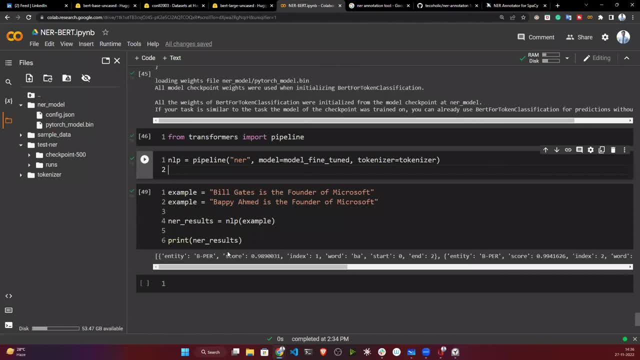 do the prediction, it will also work. but again, it may give you some wrong results, because if you are using your custom data, so better. if you are fine tuning it, at least 100 epochs, okay. so yes, guys. uh, this was all about from my side. okay, i think you got it. how to create nr using 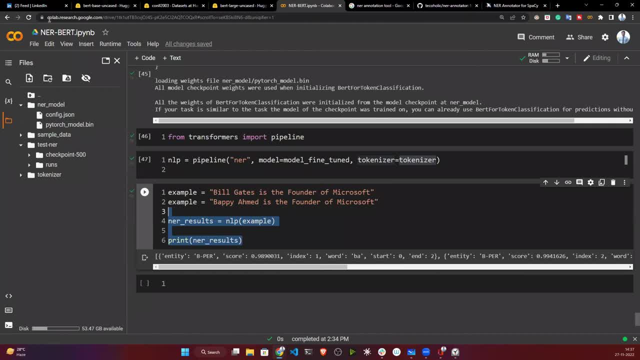 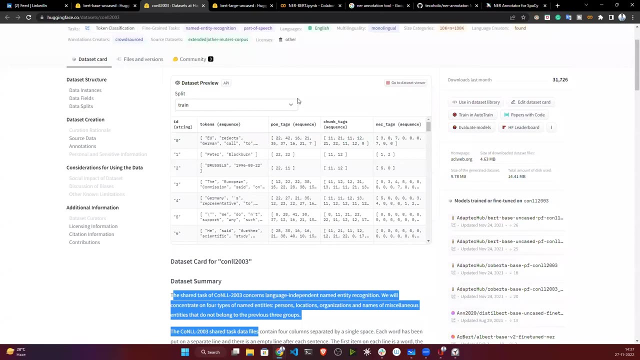 but so you can try with other model also i used, but with unkissed. so there are many model. if you go here, uh, model, select the task, token, classification, select the library you want. so see, i can. but nr is also there. if you want to use the model, copy the name and then you can use the. 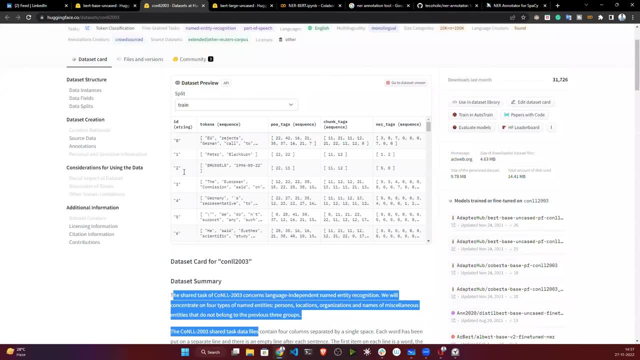 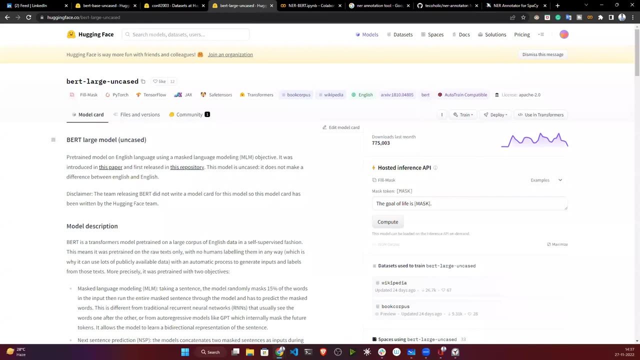 name. try with now: just play with this hugging phase guys. just play with this hugging phase api. the more you will be exploring, the more you will be learning. try to read, okay, and at the last, like there is also like some tutorials also, if you see. 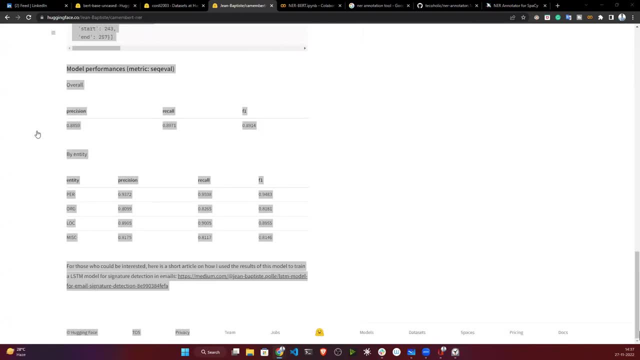 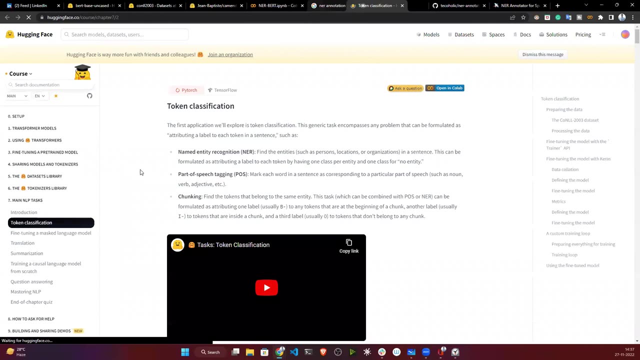 i can face, also tutorials how to do token classification, how to fine tuning the model. they have given their small, small video section. also try to see. okay, then i, i think, referred one book: natural language processing is also a good way to do that. okay, so i think that's it for this. 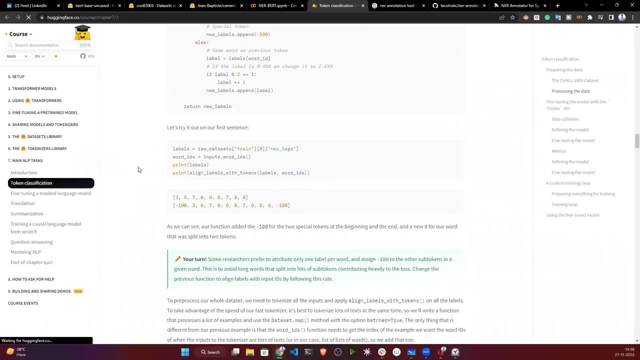 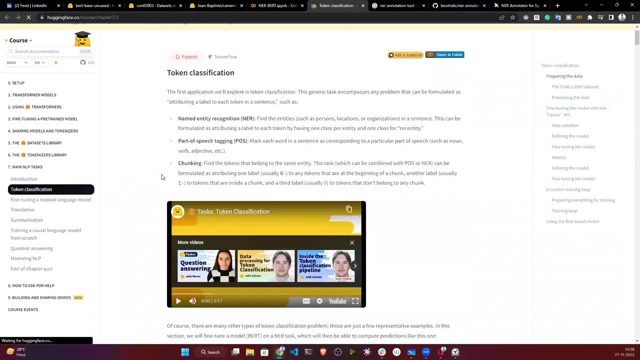 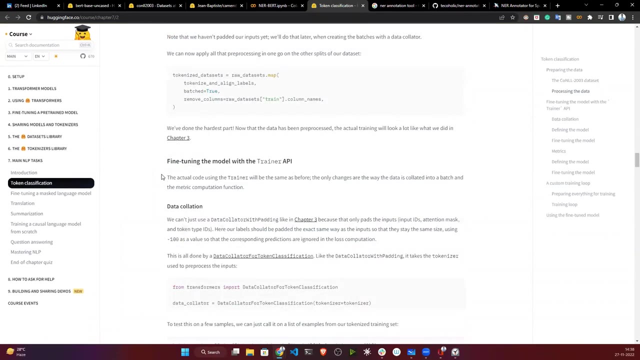 video. if you want to learn more about natural language processing with transformers, try to buy this book, because this book has been written by this developer. only hugging face developer- only if you see they have also mentioned their book name here somewhere. let me find natural language processing. i think somewhere they have mentioned nature. 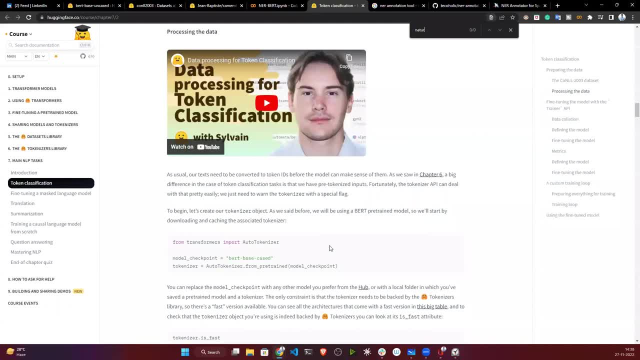 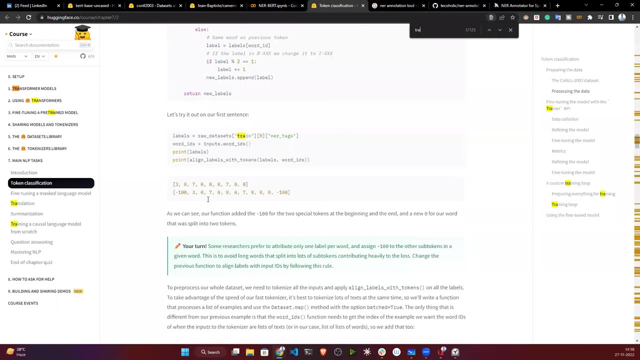 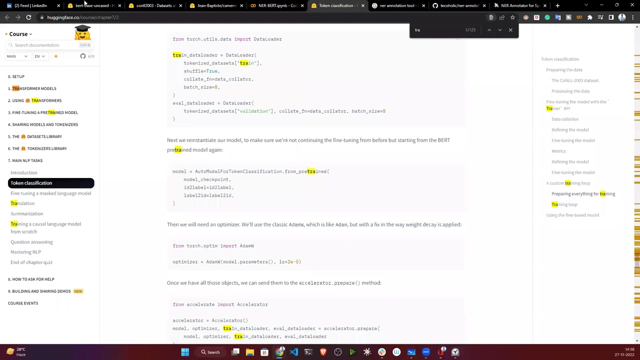 i, i think i saw somewhere they also mentioned their book to refer, hugging, first course. if you see, if you just read down somewhere, they mentioned the book book name already. okay, i, the book i shared with you. this book is also there. uh, natural language processing with transformers. 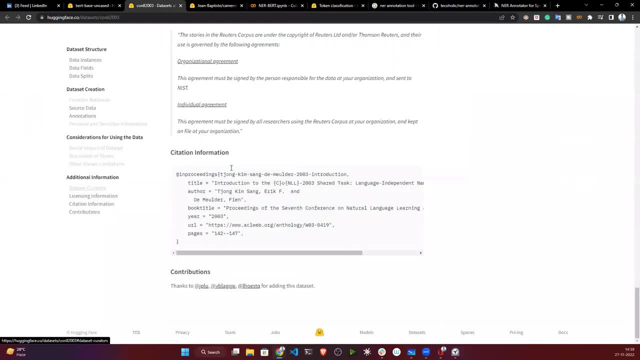 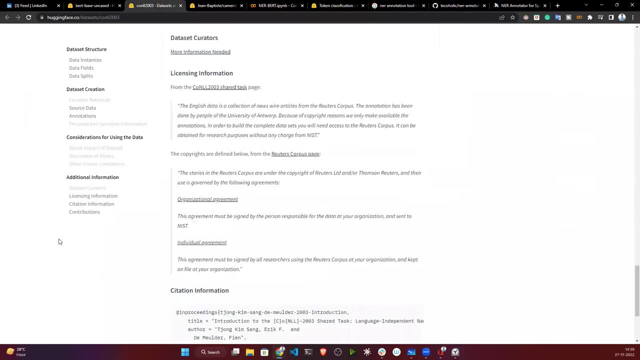 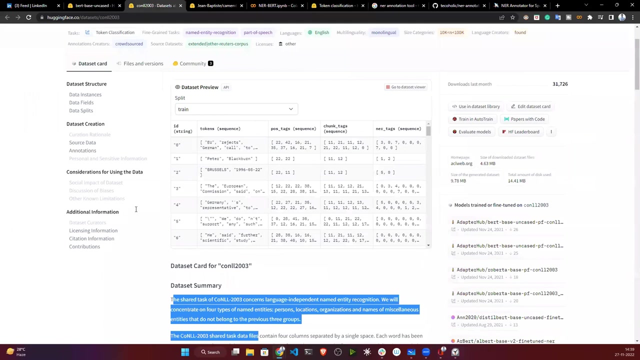 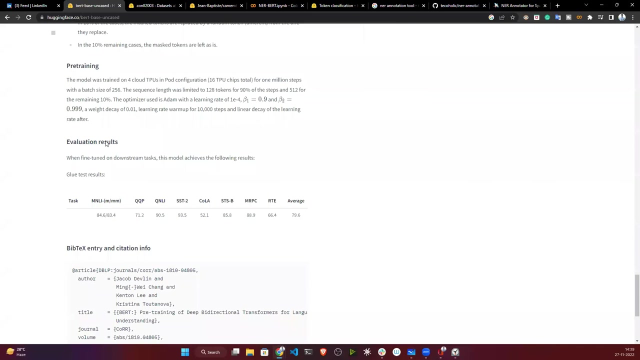 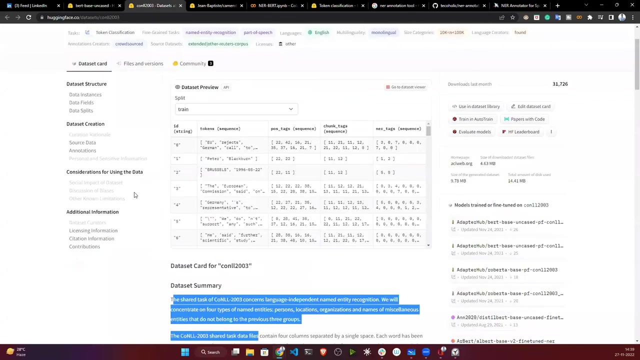 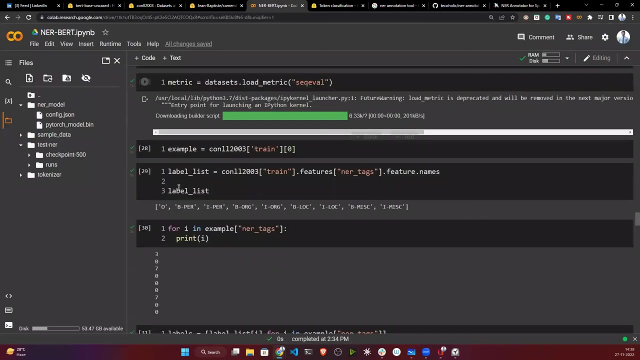 after my tutorial i will just talk about what you see. alternative source: yes, it is there. uh, so for that actually you need to write code. the code from scratch, like how to do is doing this tokenization? you can even write your own class, own function using pytorch or keras. okay, but again, it's like very challenging. 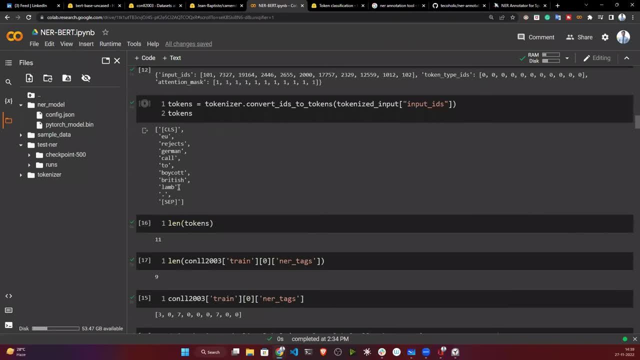 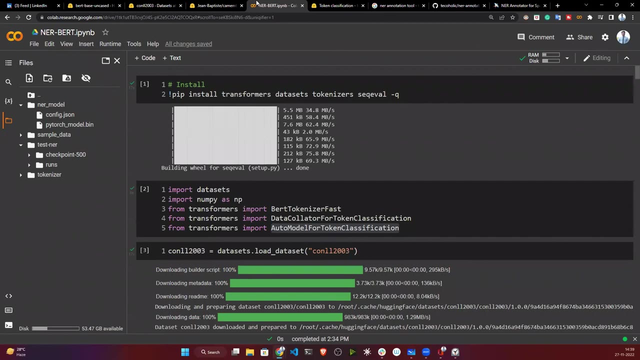 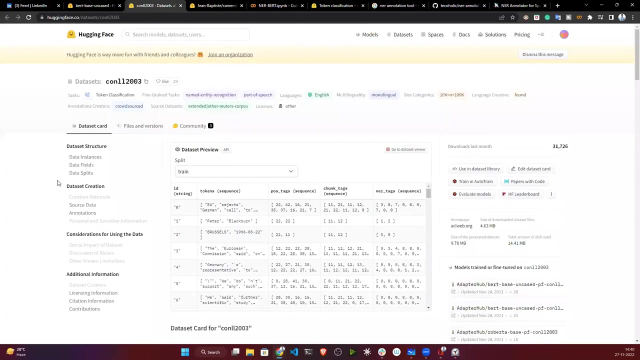 organize all the things better if you use hugging face. if you are working with the transformer based model, i will suggest you use hugging face okay, but if you are using small, small model using lstm gru, then i showed you- use keras, create your own layer, custom layer, try to train the model. but here you are loading bigger model. 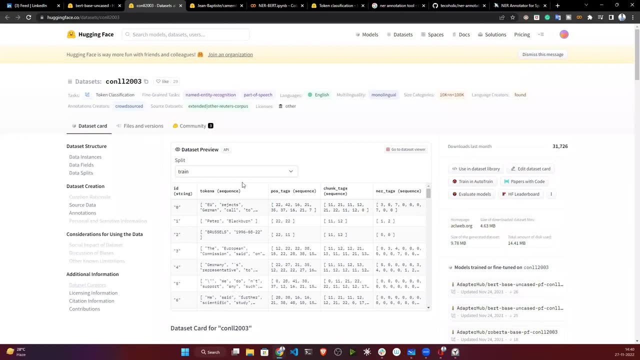 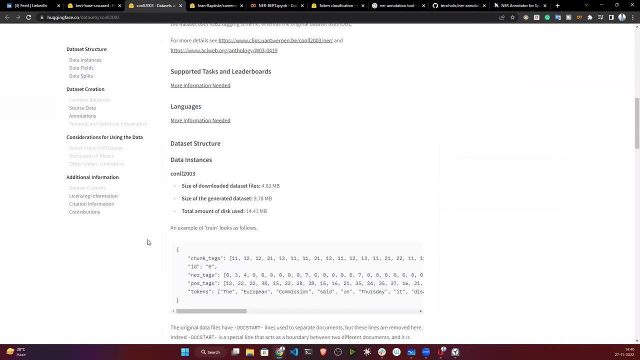 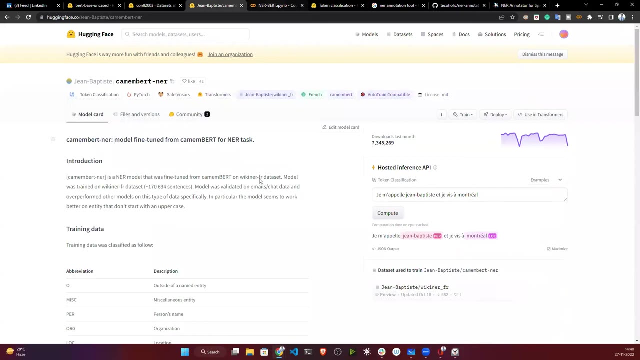 it is also memory. optimized time. complexity matters a lot, so it's an everything they are handling in their backend. you don't supposed to consider. you will be only focusing on your task, okay, so if you are writing this code, so what will happen at that position of time? your memory? 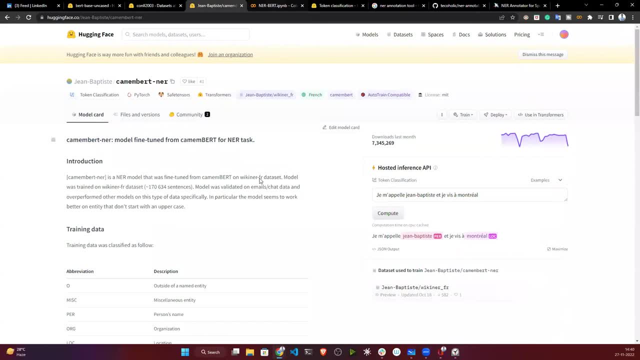 will get full. you will get a error, memory error if you are writing the code. but this api they have written. it is already optimized code, everything. see the data, the way the they are loading the data. you can see it's pretty much great. it is not showing all the information. 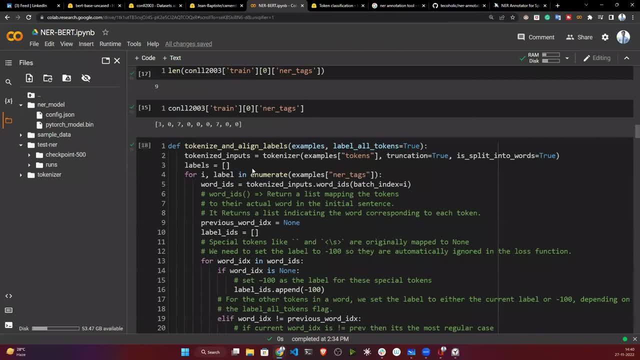 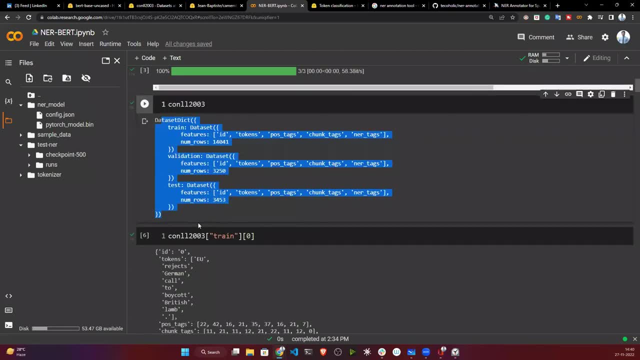 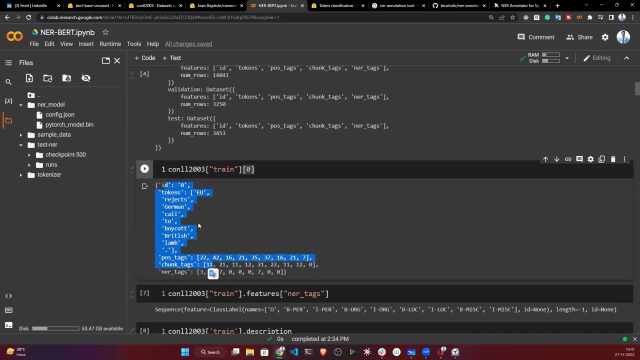 it's only giving the dictionary object and if i want to see something, i can call by their id and i can see the data. okay, so that's actually you need to. you need dsa actually to write x, like you can say: well organized code. okay, yes, see, not only hugging face, you just don't consider. hanging face is just like you can. 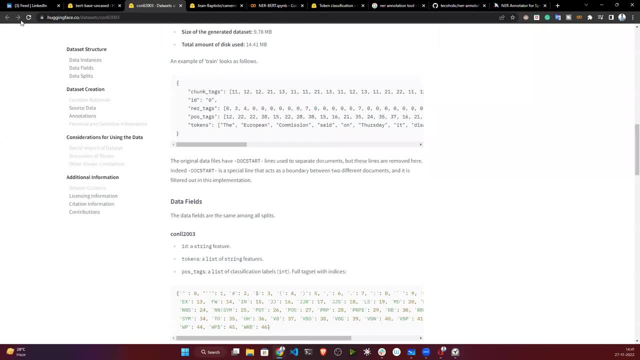 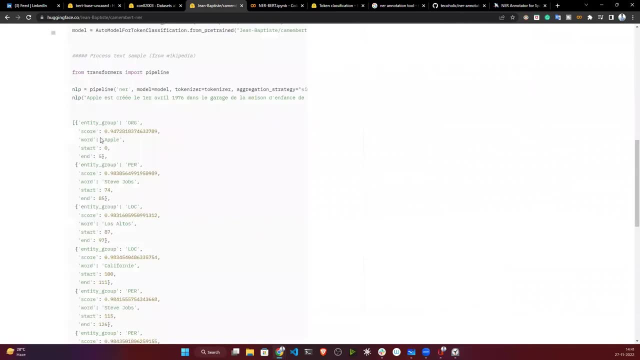 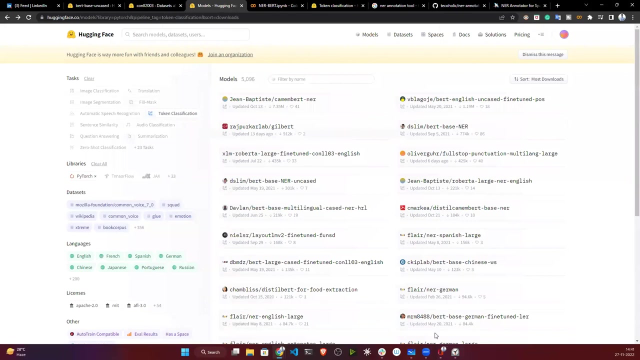 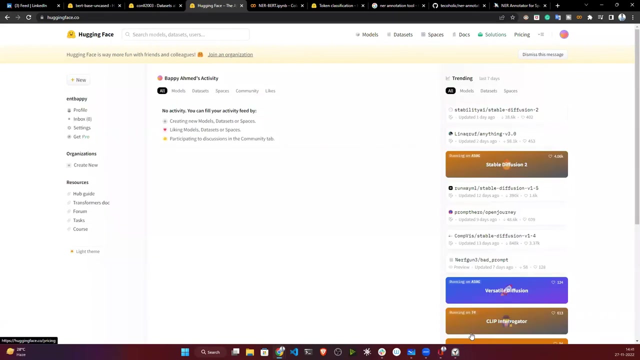 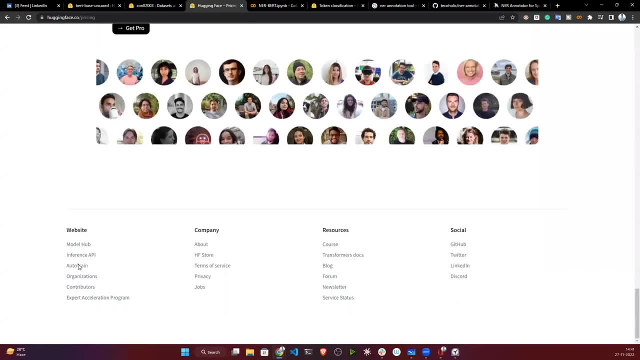 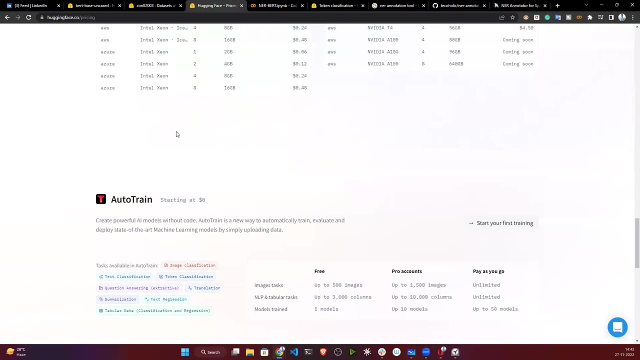 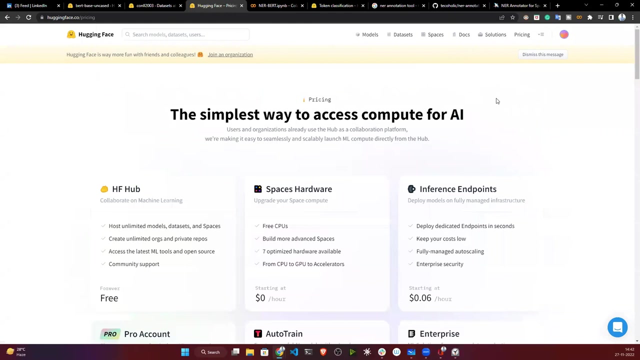 website: account comparses. website: account comparses company. it pretty much big organization. actually many of the fang company are using this hugging face as it is. even they are contributing also. yes, yes, industry is using hanging face weirdly. i'm going to discord organization. 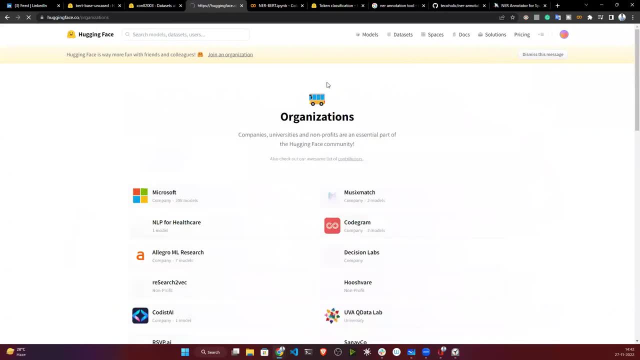 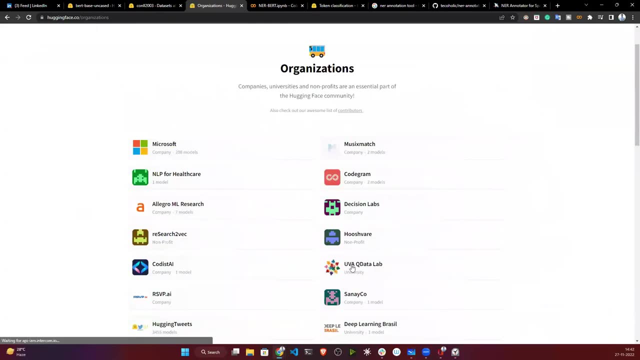 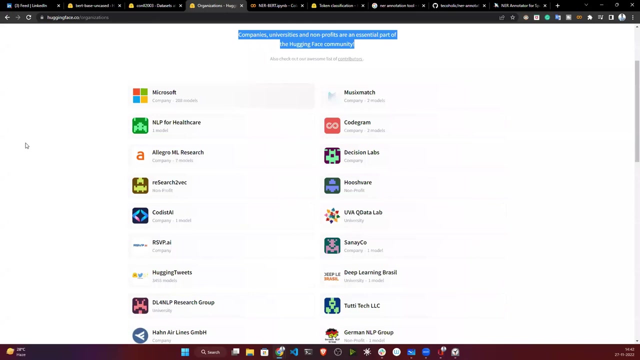 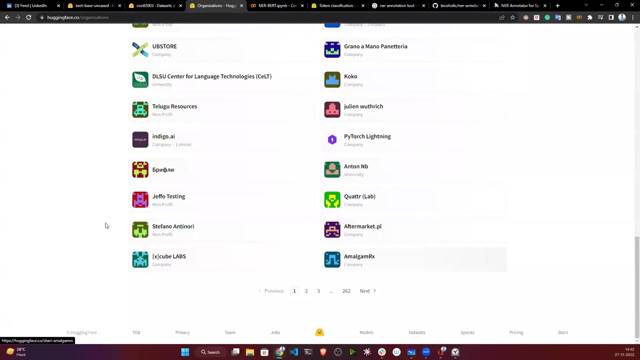 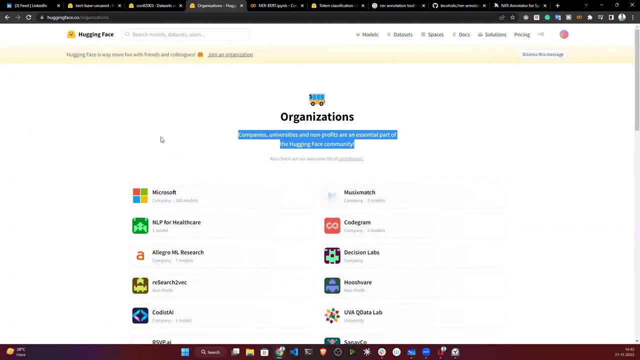 see companies part of the hugging face community. microsoft is there. these are the bigger, bigger company. if you see, see got it, even some like some days i go like google ceo- i think you know sundar, so he was. he was like one podcast so he mentioned hugging face also. like in google also they are using 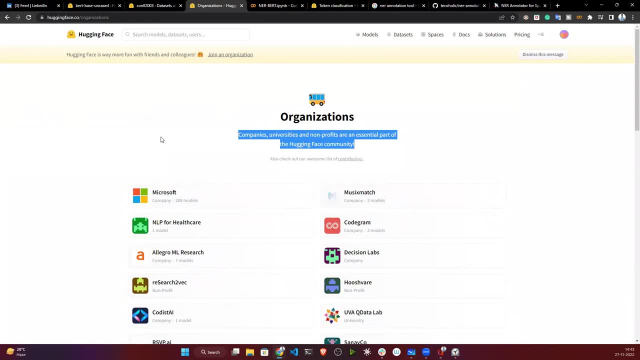 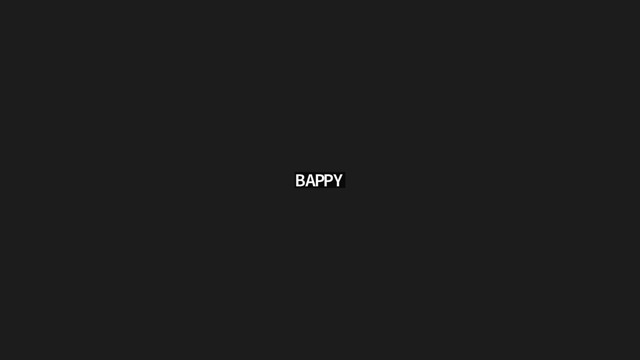 hugging face and it is pretty much good library. they're liking it okay, so yeah. so yes, guys. this was all about from my side and i think i given one task, guys, this creating this summarization application. how many of you have done so? because, see, we are showing each and everything. now it's your exploration, whatever things. 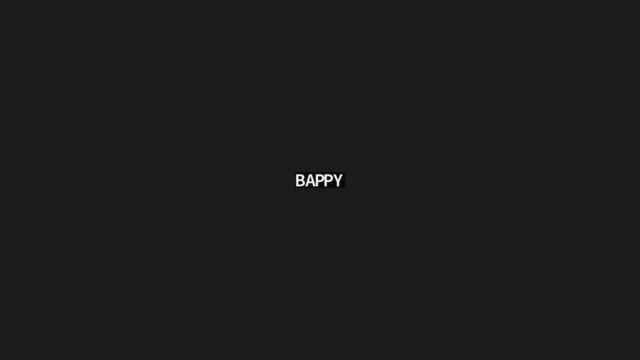 you have learned till now. try to combine them together, try to create something. okay, unless and until you are not doing exploration from your site, then it would be very difficult. okay, guys? so it is fine from my side. i think we can conclude the session. just give me yes or no. 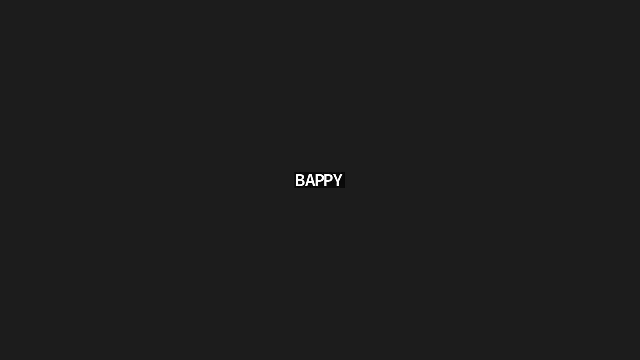 okay, palla, we did it. let me see. okay, i can see your github. you didn't deploy it right, okay? okay, i'll go through your code, but at least try to take some screenshot. okay, and it is okay. okay, so i did not deploy. okay, and i will show you how to install this, so just do this. 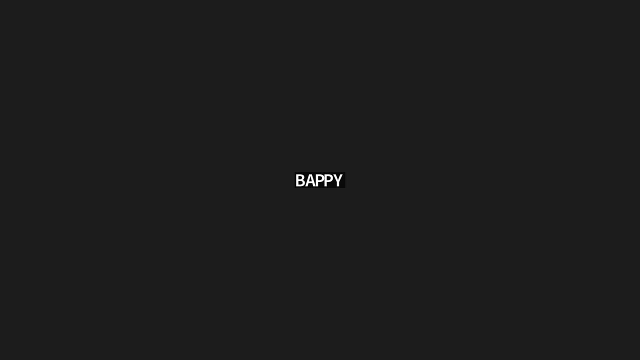 you go to the risk profile now i have mentioned in your readme, because, because it's not possible to clone the report on it, okay, at least if i see some demo you have, okay, that would be good. yeah, okay. so that's actually whatever you are learning. try to create the projects. it might be small projects, but try. 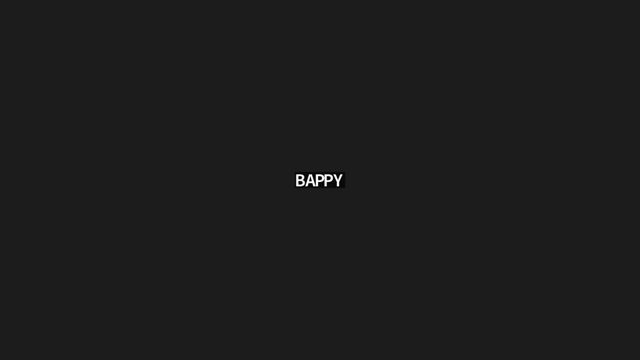 to create, then actually you are knowing how to create summarization, how to create any year you can. how i created this model. that's how i did this task. okay, like someone like asked me, asked to pause her. like i'm facing practical implementation, how to do it. that's how you need to do it. 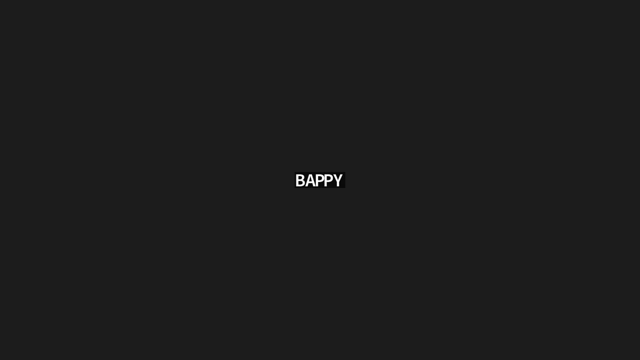 try to see separate, separate tasks, try to list down, try to do okay, try to upload it, the code in your github, then refer it in your future. you don't have to memorize everything okay, because every task has, like you can say, dependency on another task. i think i told you whenever i was discussing 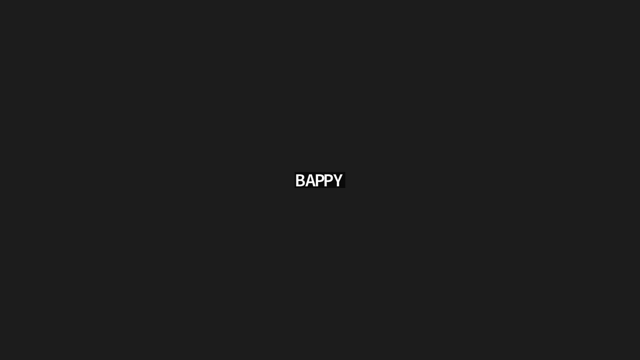 nlp pipeline, right. so first of all learn the basics. uh, like you can say: sentiment analysis, how to do classification, how to do any year. then like slowly, slowly go with like much complex problem statement. suppose, try to create chatbot? okay, try to see the example of chat, but how they? 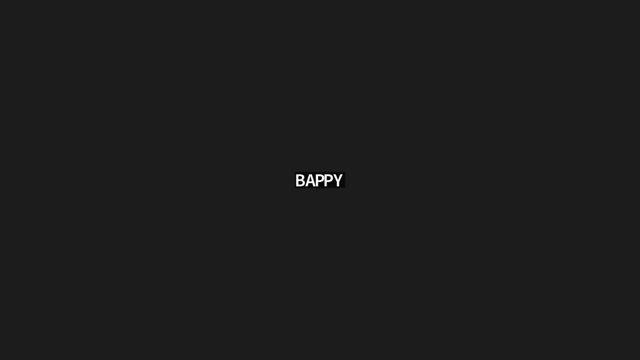 are creating. no, there is no code. i think i was explaining the theoretical way. okay, how to do classification. again, i told you see, nlp n2n is not possible, like training pipeline. it's not possible. because why? today you got the example i just trained one epochs: how, what, what was the? 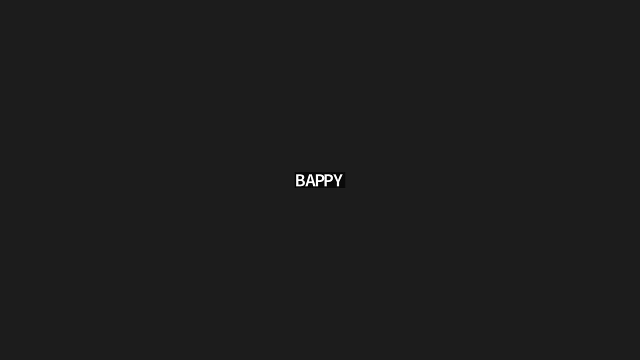 time it took. okay, n20, you can talk about, like, after training the model. you can load the model. okay, the data you are getting from the user. try to pre-process it, try to pass your to your model, try to show. okay, that's how you can do, but as per your machine learning projects you used to. 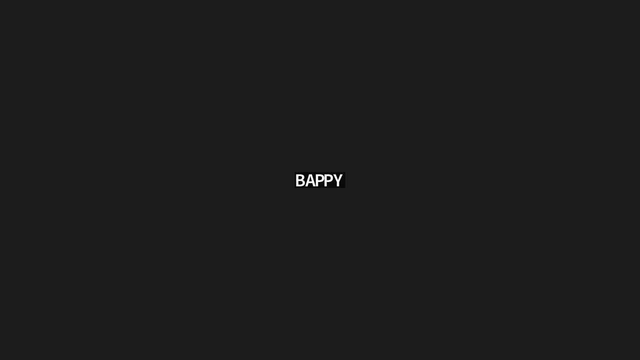 download the data. uh, in data injection, data validation, here it's not like possible, possible. you need good configuration system. again it's time taking, okay, again it's like cost effective. so better if you train your model, try to do inferencing, got it where you can apply end-to-end, suppose if you are using machine learning based algorithm or 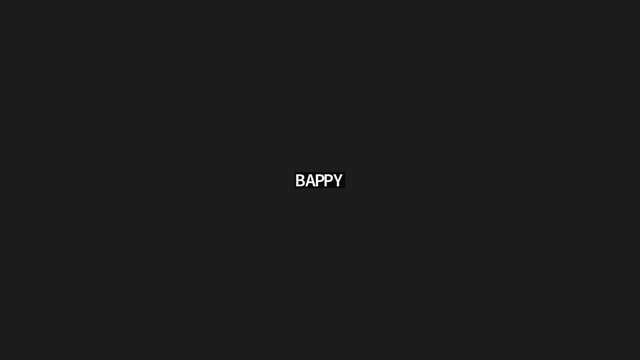 simple lstm gru at that time just create training pipeline because it will take less time, okay. but again you won't be using, because in production actually you need good accuracy always. so every time you will be using transformer based model and blindly you can trust on bart. 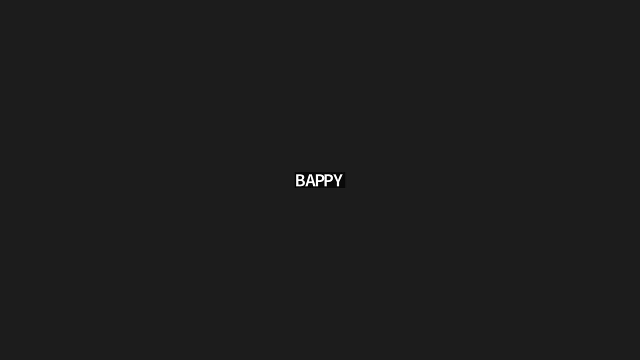 gpt, any task, okay, like in computer vision. you have vgg16 and resnet. suppose you don't know anything, you just apply vgg16. okay, it will work. okay, guys, okay. so what are we do? one thing: let's send a meeting, meeting link after uh.